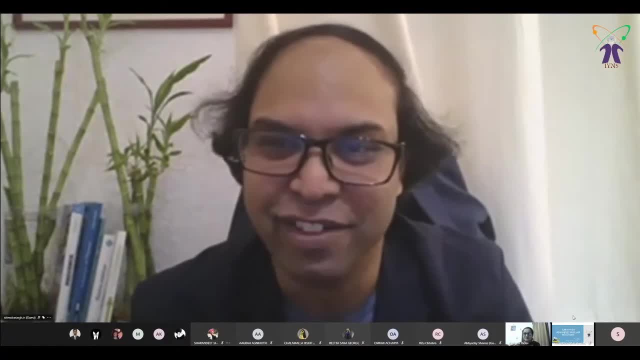 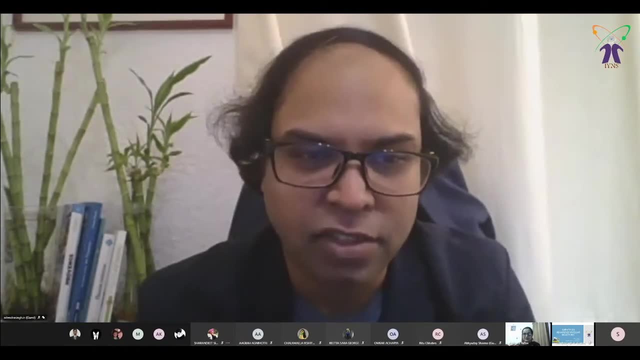 really shows the interest students on the topic. so yeah, feel free to ask anything during the conversation. as i mentioned, it should be more of an interactive session. you need not to just listen to me because i'll not be covering all the data or something which you need to mug up or 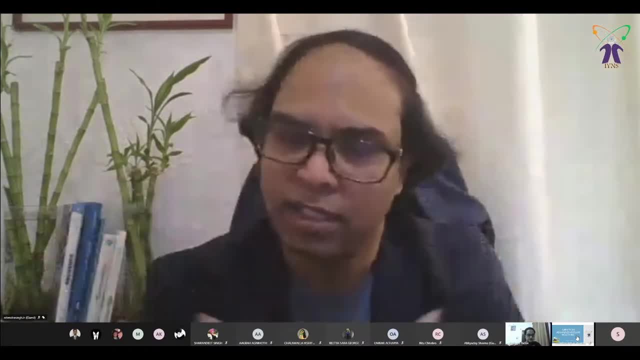 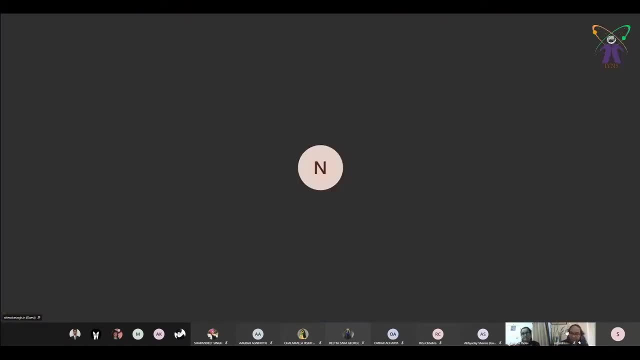 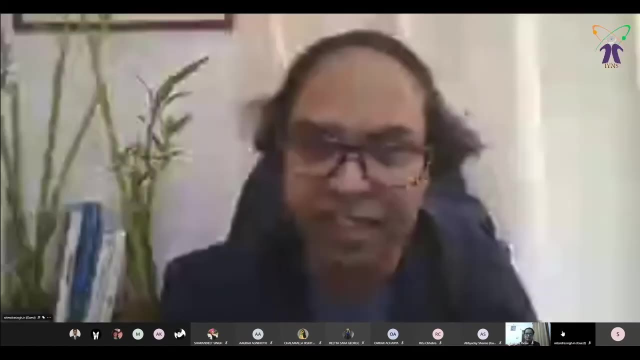 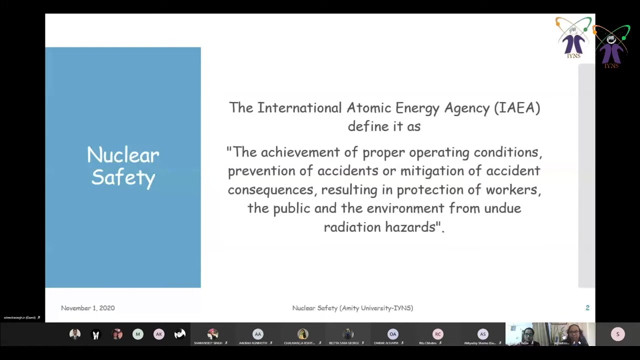 stuff, but we'll be focusing more on understanding. so yeah, today i am going to discuss more about safety, basically nuclear safety in advanced nuclear reactors. so let's begin. so very first of all, when we say nuclear safety, what do you basically understand by nuclear safety? so there is a proper definition, which is defined in international atomic energy. 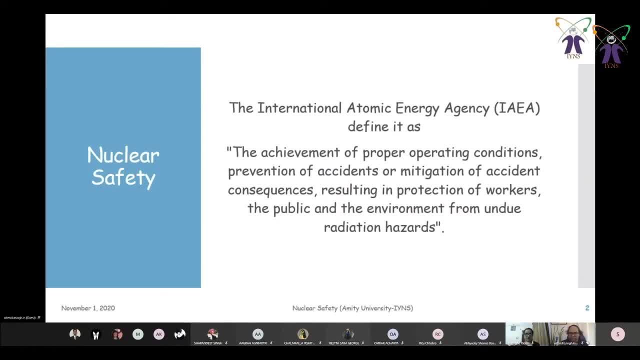 docs, uh, and it was defined very well after a long time and they have improved it. so so far, everyone across the globe is of basically taking this as the standard definition of nuclear safety, which states the achievement of proper operating conditions, prevention of accidents or mitigation of accident consequences resulting in protection of workers, the public. 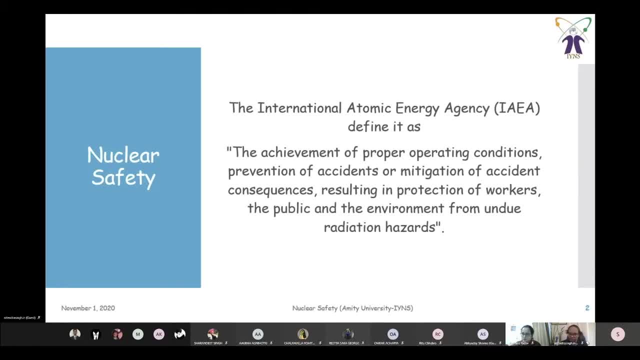 and the environment from undue radiation hazard. so if you try to understand this, this is basically a brief of everything we want to say about nuclear safety, which states like: our primary objective is to protect our workers, public and the environment from the from any kind of radiation hazard. so if you read it from back to first, then you will understand that this is the primary goal. 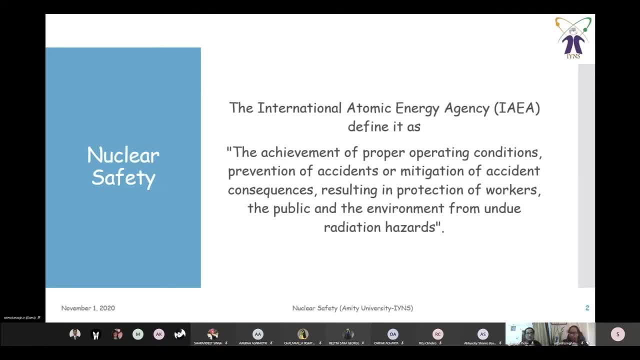 the primary objective. all the nuclear industry people, personnels, designers, operators, everyone associated with this industry- has to follow. so likewise, how you from from where these radiations hazard are coming. they might be coming from accidents or some, you know, deviation from normal operating conditions and likewise. so if you want to prevent that, you need to maintain a proper 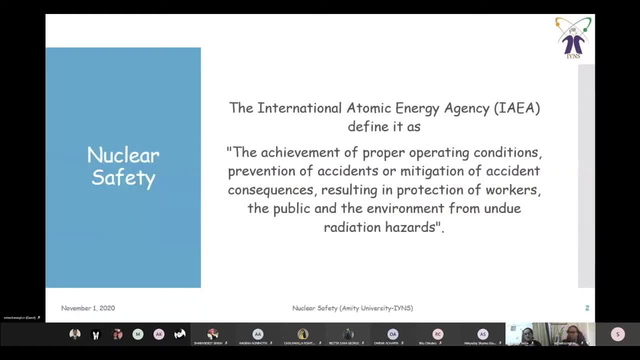 operating condition, or you must say like the safe uh or the standard operating conditions. so this way and uh. so i assume, when i am discussing this uh topic with you, all of you are well aware about the uh, the basic design of nuclear reactor. you understand what are the main components of a nuclear reactor. you have fuel. 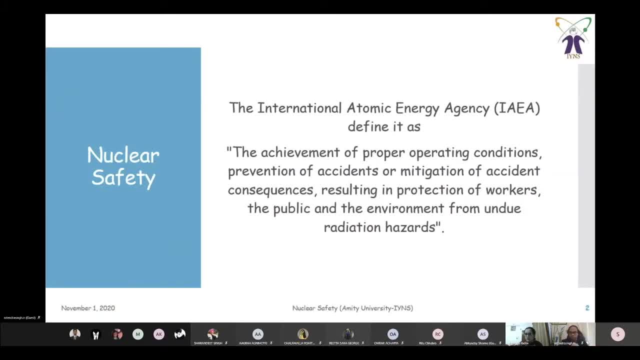 clad and all these uh internal components of a reactor combined well within the container. this is what i am assuming, yes, so yes, we are six semester plus students, so almost all of them are aware of the basic design. yeah, that will be, that will be nice. this is what i am assuming. 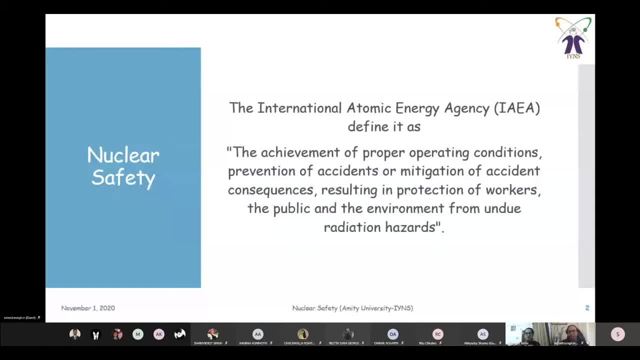 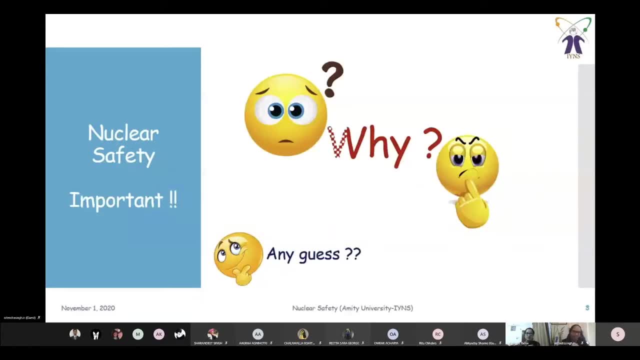 that you all. so this is the basically a definition of nuclear safety to begin with. but my question is why we actually need nuclear safety. what is so important about it? what? what do you understand, like why it is necessary? so i would say, uh, as in the definition it was mentioned from the. 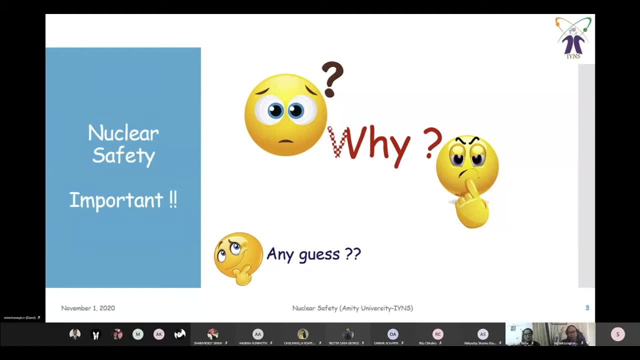 protection of personals from radiation hazard. so now the concern is: are radiations only concern or there are other aspects as well? so this we need to understand, like when we say we need to make our nuclear plants safer or when we talk about nuclear safety. so first need thing which need we? 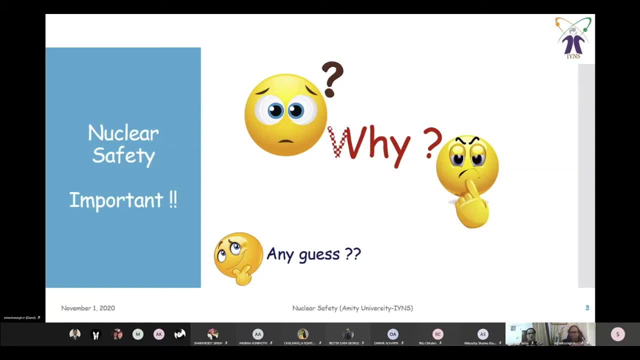 need to understand the paint on the nuclear station and do all the work we do about them, like why it is important. so radiation hazard, yes, of course. from where these radiations are coming? they might be coming from your fuel, but the fuel is very well within the core. they might be coming. 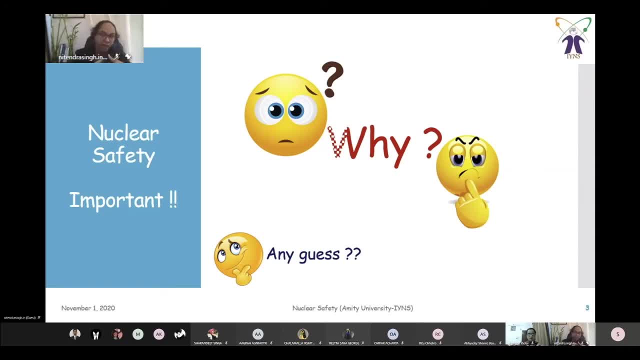 from other accidents, but why these accident have happened and, as we are saying as a designer, or we are saying that if we want to have a safe, safe reactor, then why we really need to have this nuclear safety aspect. so, coming to the next topic, why we need it. 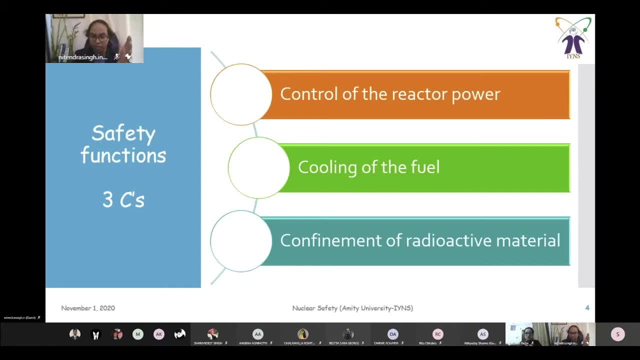 so, as i mentioned, if you want to protect your environment, your people, you need to maintain this radioactivity with well within the boundaries. so to do so, there are three mainly safety functions. when we we say, we basically say three c's in general, so like: control of the reactor power, cooling of the fuel and confinement of the radioactive material. 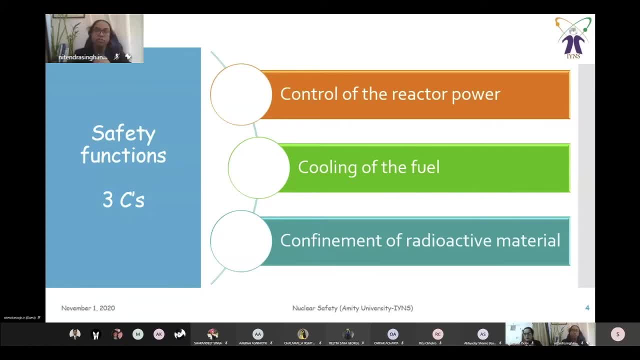 so let's discuss one by one, so, control of the nuclear powers. so you all know that nuclear fuel is, is is a very dense source of energy, so it has a lot of energy to give you. so if you need to control it in in such a manner that you can utilize it for the generation of 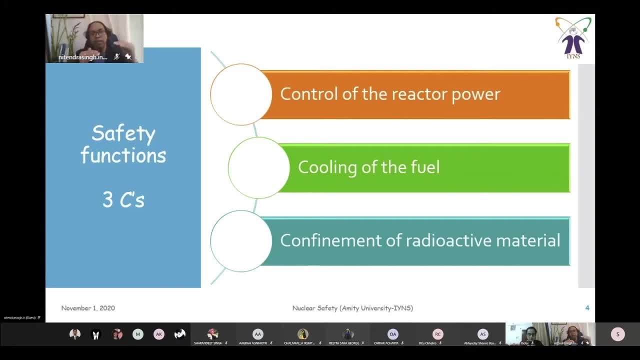 electricity, otherwise it has a lot of energy. so you need to control that in order to control you, in order to generate the uh standard electricity production. so you need to control the reactor power in such a manner that it should not exceed from your safety limits. so how you do, 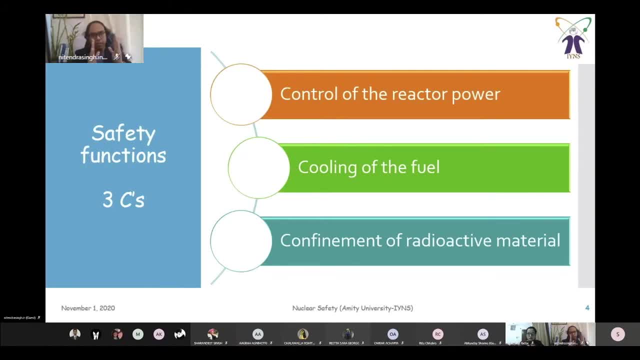 it that will discuss. so you need to like, if you understand the basic physics. there is a uranium as a fuel, for example, you bombard it with the nuclear, and if you have a lot of uranium atom or nuclei, then you, if you keep on bombarding with neutrons. 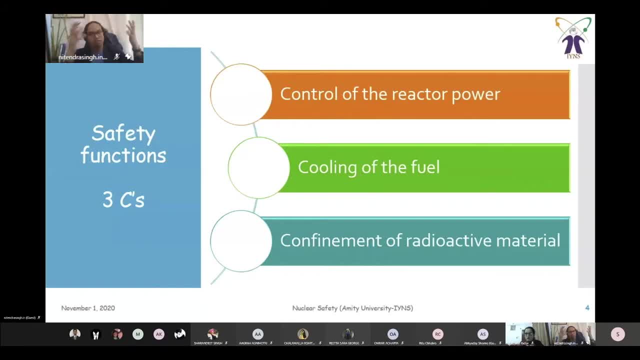 there is a chain reaction which is uncontrolled because of presence of so many uranium nuclei and in each nuclear reaction you are having additional neutron generation which can give you additional chain reaction or an uncontrolled chain reaction. so you need to control that power, you need to control that reaction to have the better operating or better functioning of the nuclear 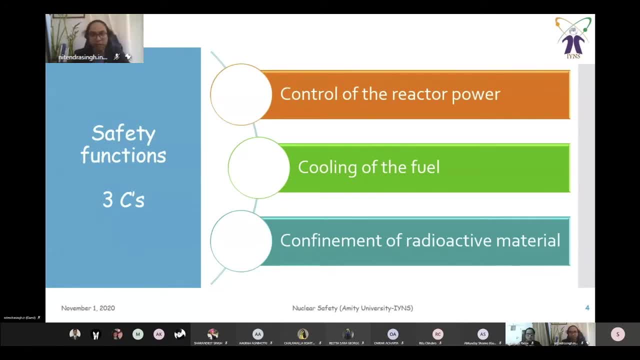 reactor. so this is one. secondly, cooling of the fuel. why fuel need to be cooled. so one in, not on normal condition, you say, because we need to cool the field, because we want to take out this energy. you want to convert that uh energy into your using that and you want to convert the coolant into 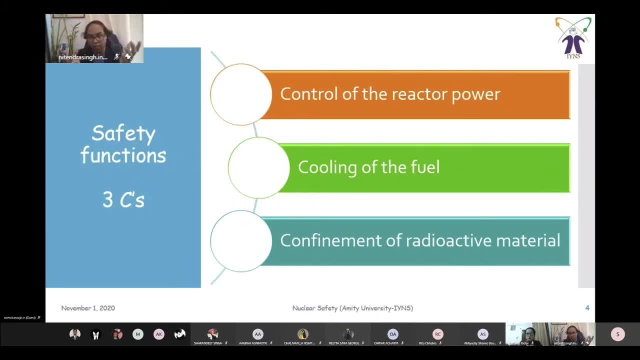 uh, the steam, and you want to generate the electricity. that that is one option. however, there is another aspect which is like: even if the fuel is not or the reactor is shut down, for example, so the fuel is still releasing some energy, which is called as decay heat. 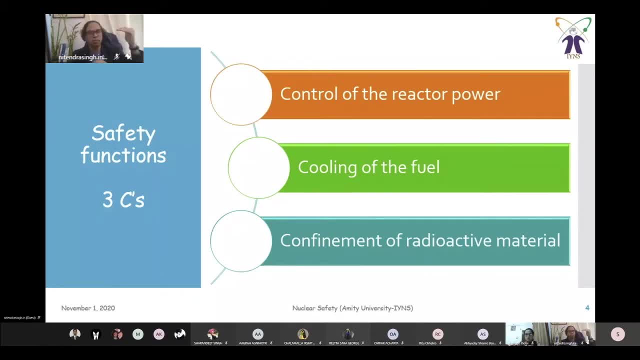 which comes mainly from the fission products. so when you have, like, a nuclear reaction between you with uranium and neutron, you generate some fission fragments which they continue to decay and keep on generating some decay heat as we call, say, and which is quite enormous, for example, if you 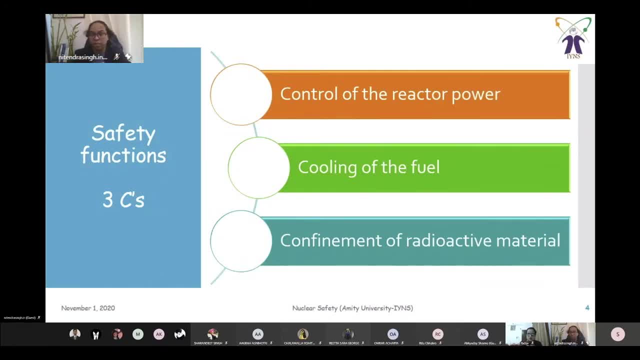 are having a 1000 megawatt electric of 1000 megawatt of a reactor, then even if this decay heat is point i mean one percent- then it's huge. it's like, uh, you know, it's like 10 megawatt you're having out of. 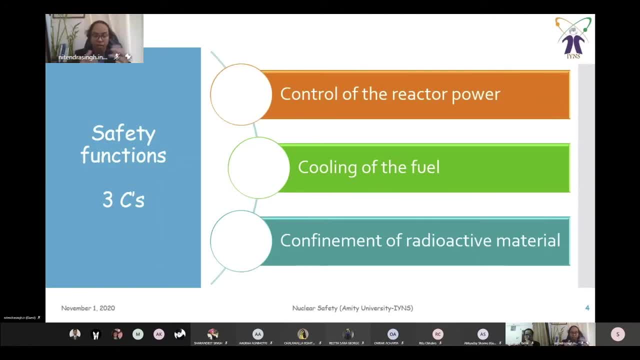 nowhere, which is a huge amount of electricity, energy. so to say so, you still need to con cool that fuel. so somehow, even if you don't cool it, then what will happen? so yeah, one thing i want to mention in the first topic as well: if you don't, 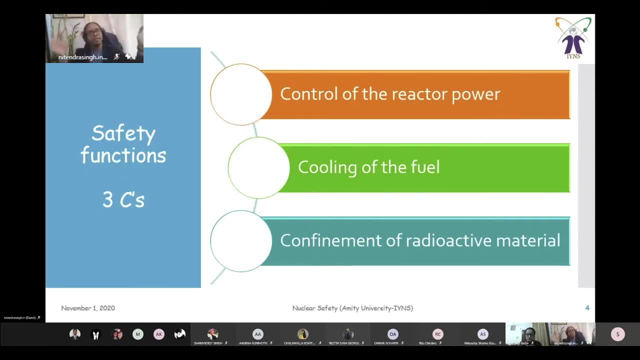 control the reactor power. what will happen? it will exceed the reactor power. it will, you know, produce enormous amount of energy which you will not be able to handle or which you will not be able to manage. so if you don't cool the fuel, it will keep on generating uh energy and which will result in increase in the temperature of fuel. 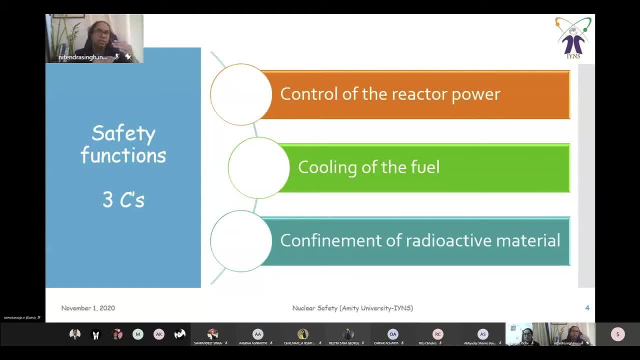 if you understand, if the fuel temperature will increase, then the surrounding clad temperature will increase. with the increase in this uh surrounding clear temperatures, there is a possibility of failure of this clack, which will result in the failure of other surrounding components and likewise this thing will keep on happening. so you need to control. 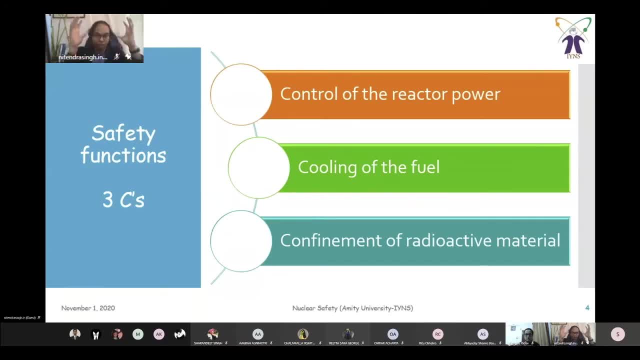 reactor power, why? to control the, the reaction and control the energy which could be generated, you need to cool the fuel so that the fuel temperature and everything should not reach uh, should not raise to to the level where the failure of the surrounding components and the structure is a concern. and third, very important aspect is the confinement of the radiation. 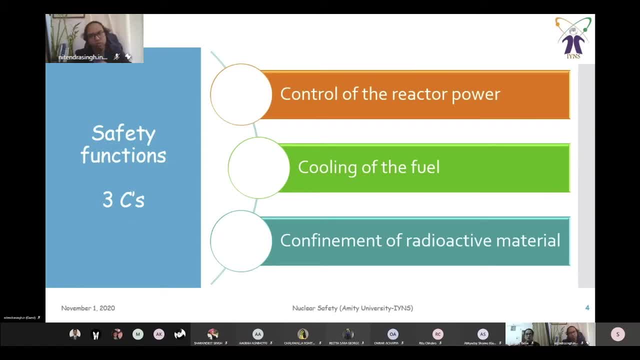 radioactive material. so if any of the two aspect, if you see the first and second, there is a possibility of radioactive release in the nuclear reactor or within the nuclear reactor. so if you go back to the definition, you understand we need to protect our environment or the people from this radioactive, so somehow you need to maintain it within the system or within the, within the zone. 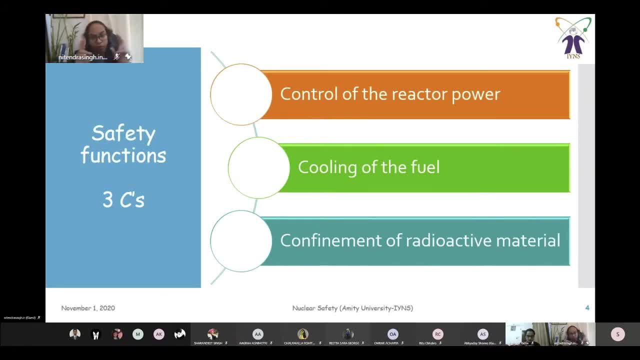 I would use the word here- or to be precise, within the containment, because you should not. no radioactive material should go outside the reactor. then only we can say: we are able to maintain a reactor safe or radio nuclear safety is maintained. so these are the three safety function around which your entire entire nuclear industry is focused. everything you do is. 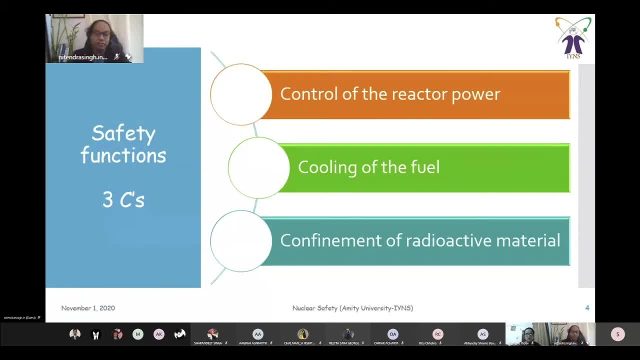 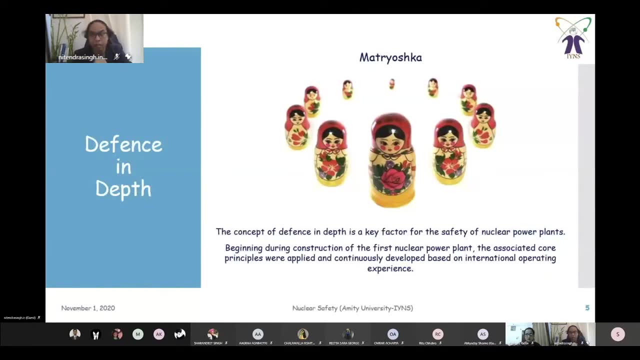 mainly to maintain these three functions in a nuclear reactor. one more concept: how you maintain these safety functions. so the concept you basically maintain this safety function is using the defense and depth philosophy. so what is this defense and depth philosophy? I'm sure all of you are aware of this. 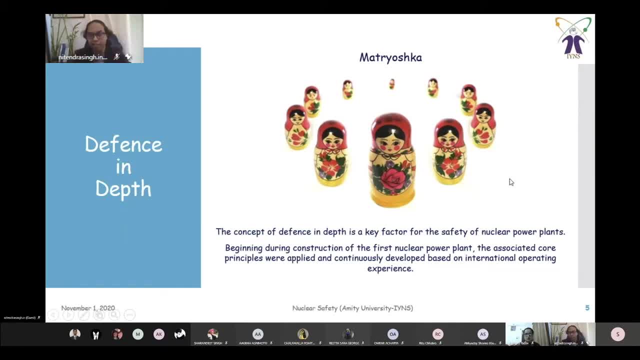 which is like in a common name known as the russian dogs. they are the dog with you, dogs with you, know, like waves, Jason, small dog, which is cap capsulated in Islander dog, which is capsulated in Islander dog, an other likewise, so you have a layer up in a similar fashion. we 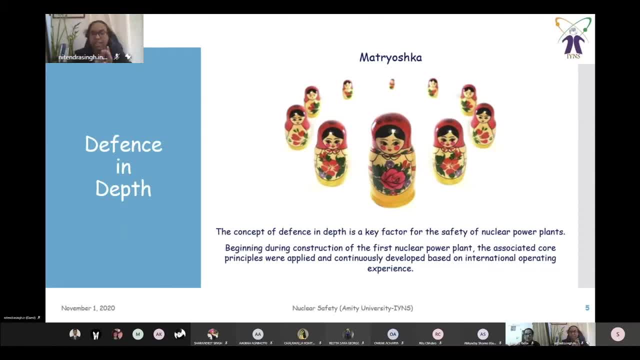 have this concept of the things, which is a key factor for the safety nuclear power plant. so concept of defense, and that is not only for nuclear powers, it is applicable in any condition. it is very well applicable and is being used as well in aircraft industries, in, I mean in aviation, in your IT industry, for all. 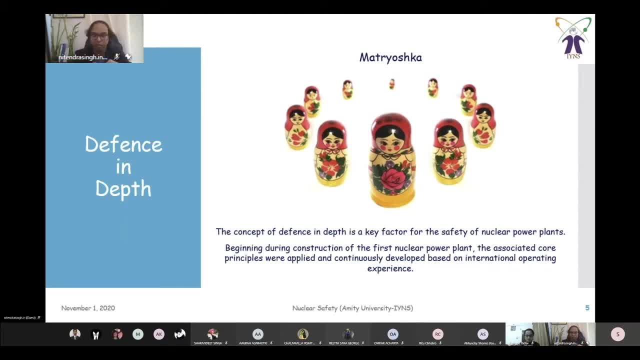 the firewalls and all, and of course in in nuclear industry but in many other another industries where the risk factor is high, you know. so we apply in a nuclear industry, we apply the concept of defense in depth since inception of the- you know- design and we beginning during the construction of the power. 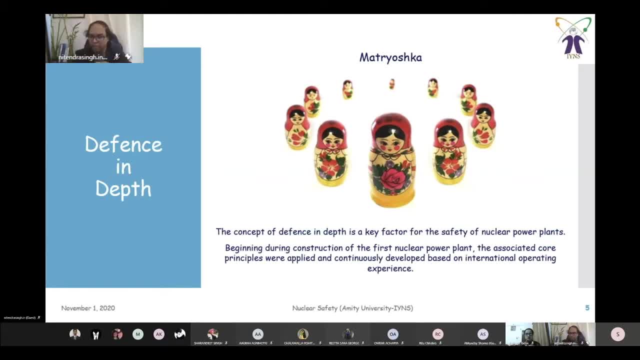 plant and we apply all the principles you know to develop this concept and culture within the, within the design as well as in operation, and this is continuously, you know, developed or improved, basically based on the international operating experiences, because not all countries can basically have all the experience. we have different type of reactors working across the globe, like 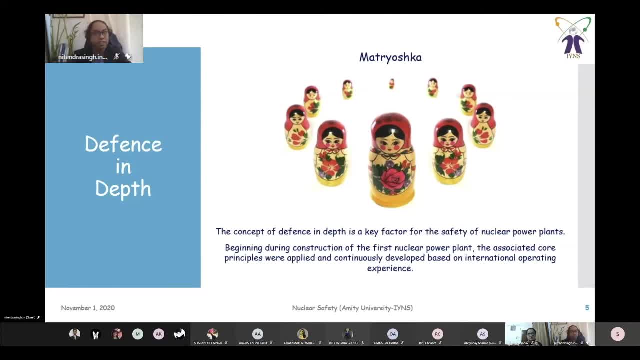 for the moment, around 438 different type of nuclear reactors are operating across the globe, so they all have a different kind of experience, different type of experience and different timeline of the experiences. so they all work together to improve this concept. now the thing is, what is difference in depth? we mentioned like it's something layered and 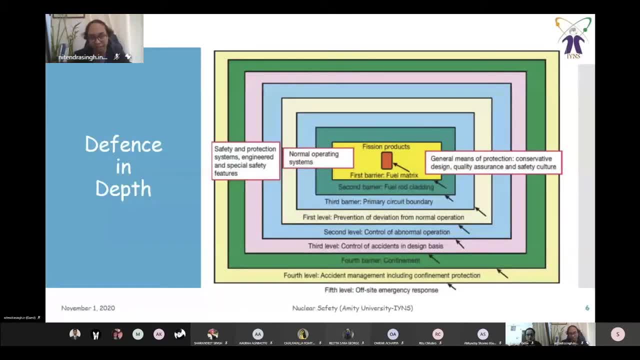 you might have seen this picture for quite a long time. this is something you will find in all the text, all the IAEA document, every book. they say this is the. you know different kind of layers you will find and different kind of systems you will find. so let's discuss a bit about it. I am more fascinated with the other pictures which I 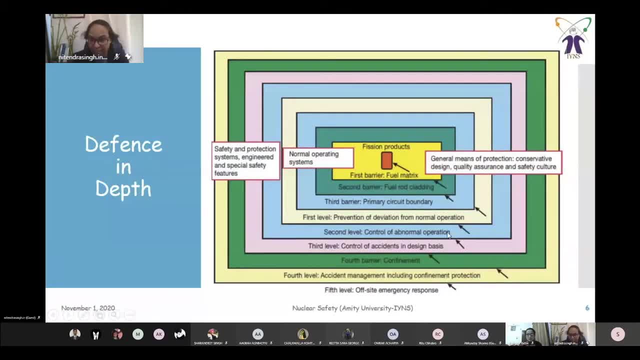 will show you later, but just briefly so, what this basically says. you have a safety barriers, so the first barrier is the your fuel itself, because the fuel is so designed that all the fission fragments and everything are within, that remains within that fuel itself, which which is encapsulated within a fuel slag or a fuel rod, or maybe even a fuel pump. that 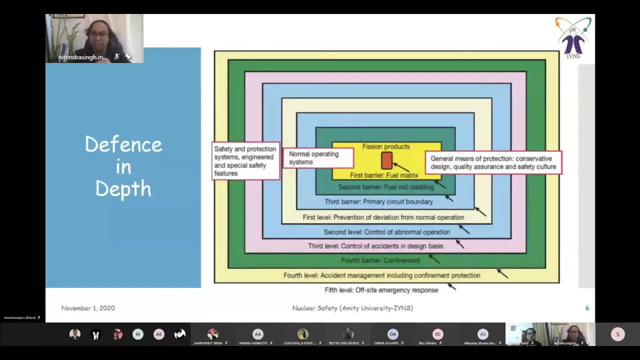 is really the fuel that comes with the fuel. so let's see how it covers the fuel itself. or a fume pin, different type of names it has. it is the second barrier. then you have the third barrier, which is the your primary circulation system, primary coolant system. or you can say: 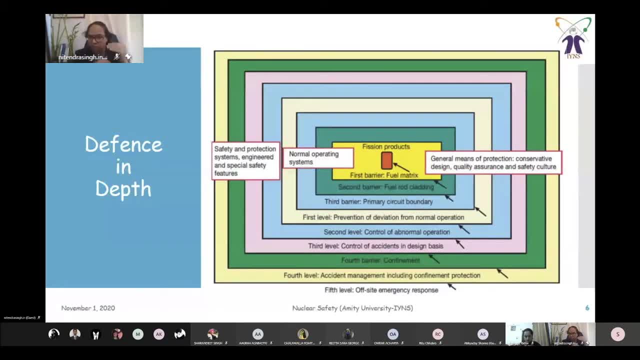 then you have a fourth barrier, which is the, which is your containment or containment building. you have seen the, the dome around this thing, so likewise you am. in some cases, you also apply a fifth barrier where you have this exclusion zone. it depends, it varies, uh, um, depending on. 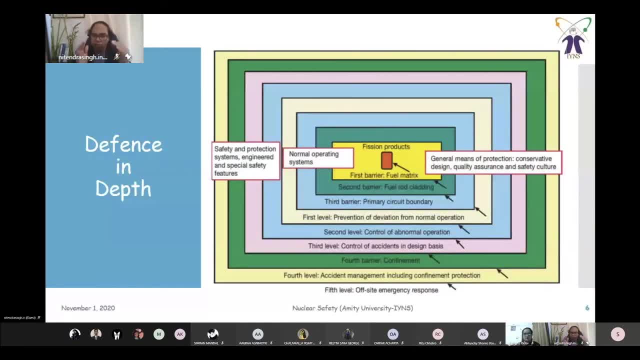 the policies of the of the country and along with that you also have the associated uh safety levels where you, you, you maintain like: firstly, level one, you try to prevent all the deviations from the normal you operation. and level two, you control. if something deviated, you try to control it. and in third, if 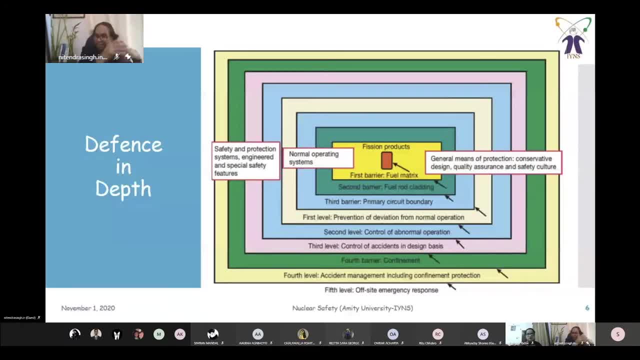 if something is happening, okay, you try to control the accident scenario within the uh design basis uh functions. so design basis scenarios are those where you have already thought that this might go wrong and if this will go wrong, we need to provide this as the safety function. so these are: 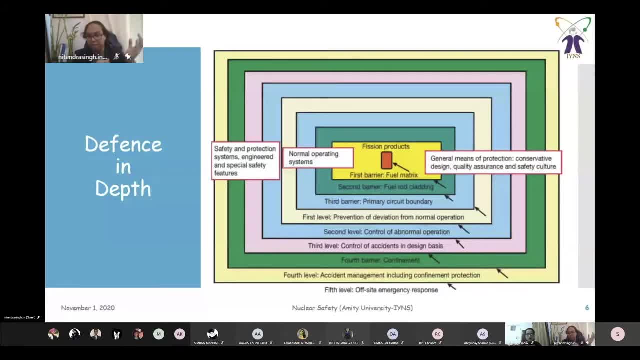 design basis uh levels. and uh fourth level is okay. now things are happening. you need to manage this accident, you need to control this accident progression so the damage could be minimized. and the fifth level: okay, it is going outside the uh boundary you need to be prepared for. 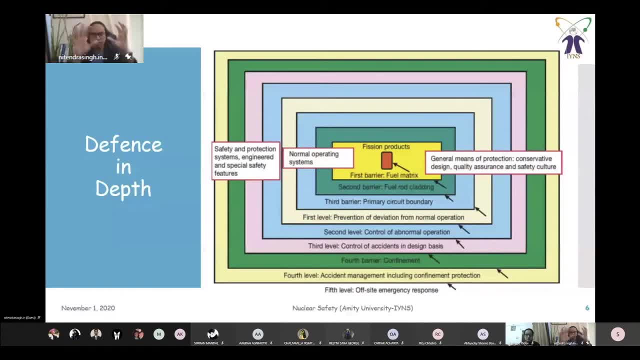 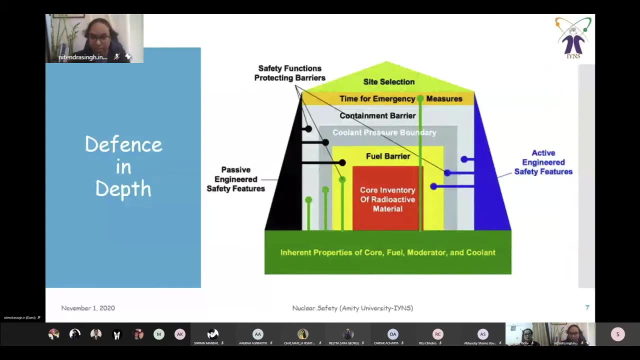 all the emergency responses for the public. so, like, this is the the the main idea. and how do you do it? uh, you have different type of systems for each level and something like this. i'll come to that. i am more happy with this site type of diagram, more colorful and more easy. so, like, as i mentioned you. 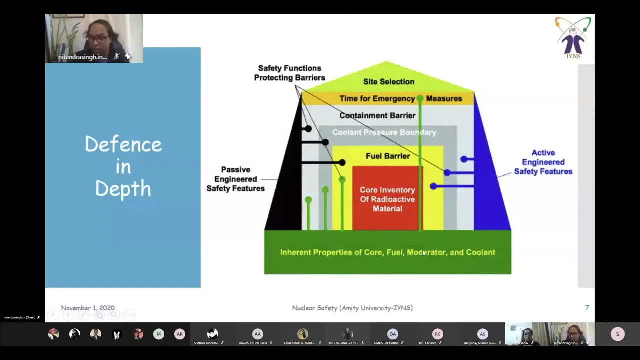 have a inherent properties of core, fuel, moderator and coolant which make it- uh, you know- more safer. and you have a core inventory and different type of barriers which i mentioned, like you know, fuel barrier, coolant, boundary containment barrier, then, of course, the the explosion zone. if you have something, and to maintain that you apply some engineered safety. 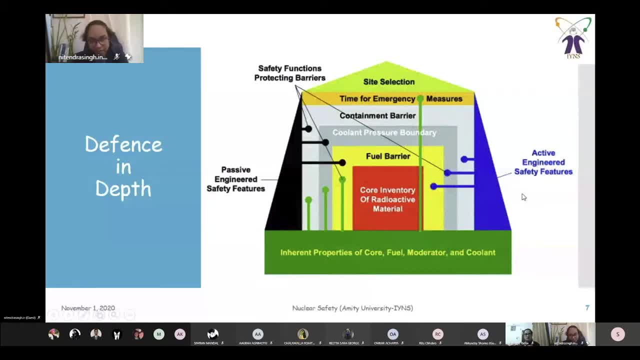 systems, or sometimes we call it safety systems for the reactors, and along with that, you also have safety barriers, which are already in place, uh, which are like this, this which are mentioned, and along with that, in the advanced reactor, we say passive engineered safety features or passive safety. 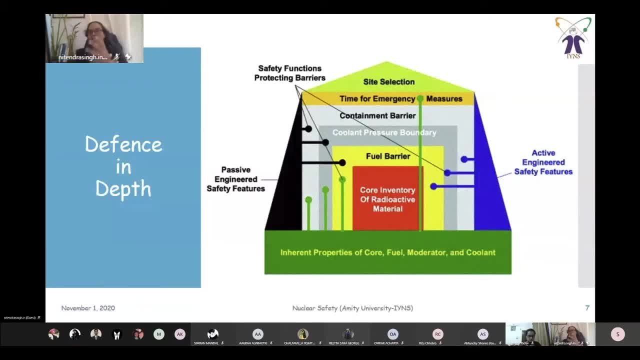 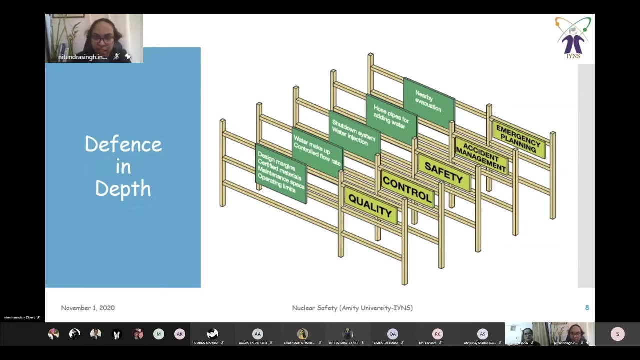 system that will discuss. so they all together now make your- you know, defense in depth philosophy for the nuclear safety in nuclear reactors. you might have seen this picture as well. i am not very sure if you have not seen it. so, as i was mentioning. so there are possibility if 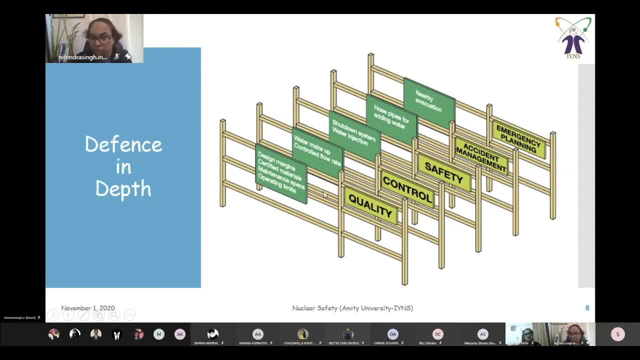 you want to maintain these five levels, how you can do it. so this is one diagram which i always wanted to show everyone. like there are design margins and you know the design margins, the you can maintain every function within your operating limits and how you can do it. you 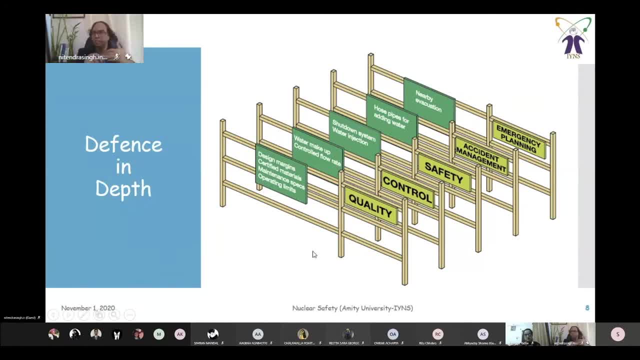 have to maintain quality, quality in everything, quality in material, quality in people, quality in working, everything that you need to maintain that quality. then if something, some deviations are happening, some, some deviations are there, then you try to control that, using, for example here they have mentioned, like if there is a loss of flow or use, it seems like water will be low. 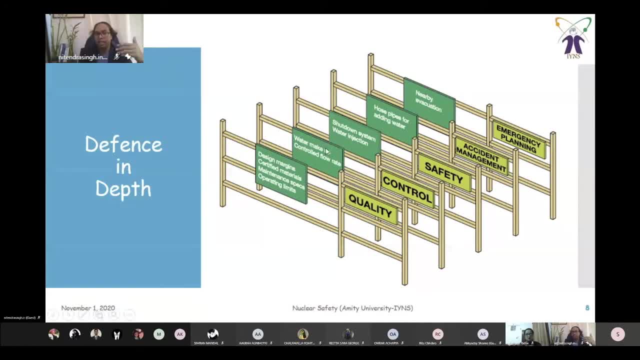 to cool the fuel, then you try to make up with the water and then the next is safety. okay, if something is happening, it's you shut down everything. then even then, in the shutdown situation, you maintain the shutdown cooling because of the decay heat. so you maintain the 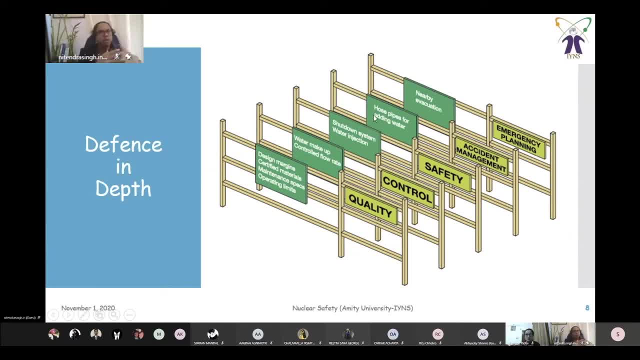 safety still, and if something is happening you are not able to control, as I was mentioning. so you try to minimize the accident progression, so which is called as accident management, and if everything has happened, now the radioactivity is going out, then you try to work on emergency responses. so different way of explaining. 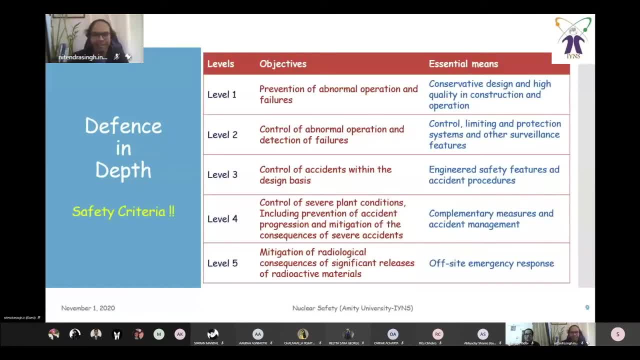 many thing, and this is the more standard way, more textbook way. so there are the five levels in depth and these are the primary objectives which we need to follow for each level, and how do you follow it? this is the important part which we should discuss, as i was discussing in the 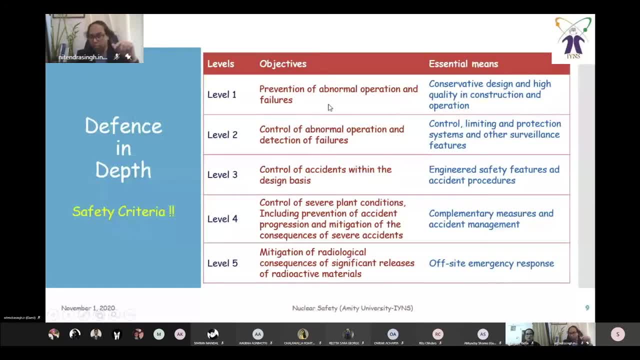 previous uh picture. so if you want to prevent all the abnormal operation or the deviations, you try to maintain the conservative design, as i was mentioning. you maintain the quality in design, construction and in operation. similarly, if something has happened, some deviations are there, then you try to control these operations and detect the failures and for that you use 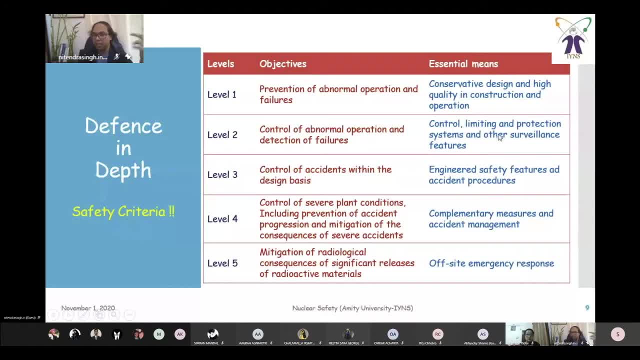 different kind of control system, limiting system, protection system and other surveillance features. and if something is happening now, the accident is in progression, then you control the accident within the design basis and for that you use the senior safety system, as i was uh mentioning, and also, of course, the accident procedures to 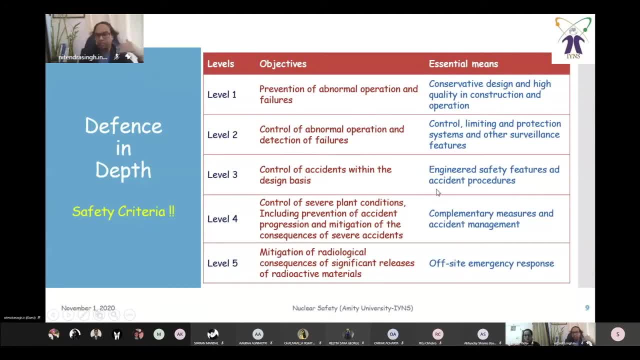 maintain everything within the design business. but if something is beyond, if it is going beyond design business, ex accidents, then we call the term in: it's the severe accidents. then you try to control the severe plant conditions as much as possible. you try to prevent the accident progression. 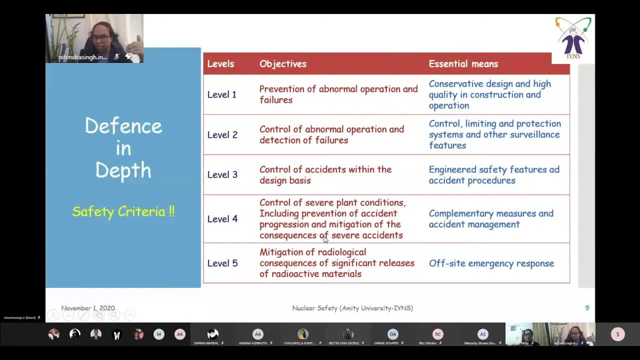 you try to mitigate the consequence, consequences of severe accident. you try to minimize the the losses, and to do so you use different complementary measures and accident management. and this is the very level 4. earlier it was thought like level 4 is not the something which we will deal with, but after fukushima this is something. 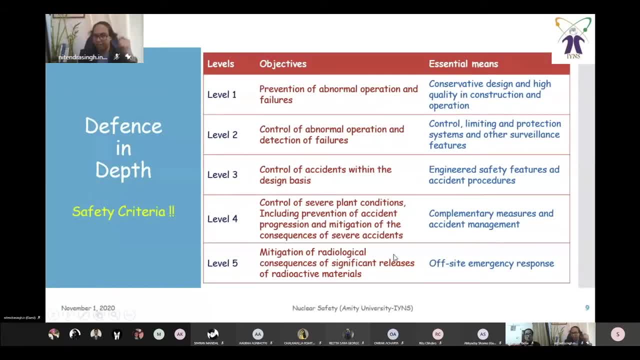 which everyone has realized that we should work on this as well. level 5 is. level 5 is the mitigation of radiological consequences. so after this, if radio activity is releasing to the environment, then you try to mitigate that so that the you can reduce the this significant release of the radioactive material, and that you do using your. 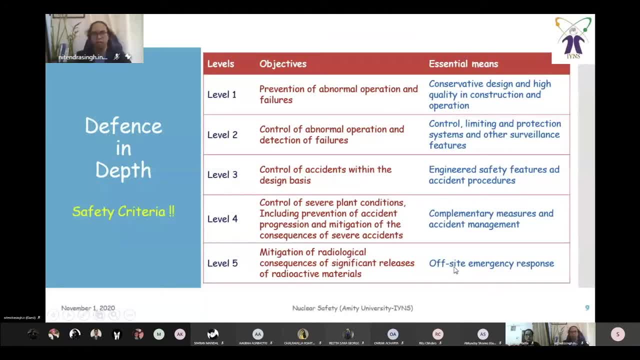 off-site emergency response. you may go for evacuation or you may plan it in a different manner, and these days we call it as a severe accident management guidelines and or, in some cases, severe accident management strategy, where these two levels works in indian and it's really important for all of us to. 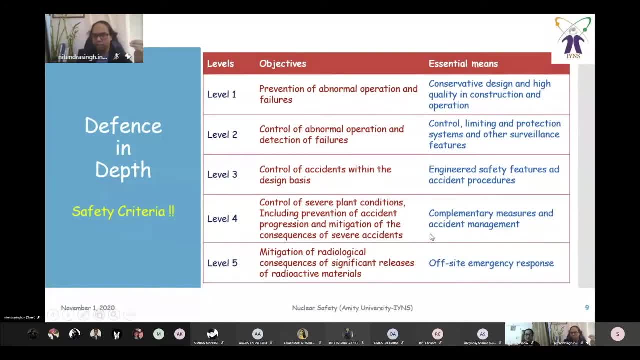 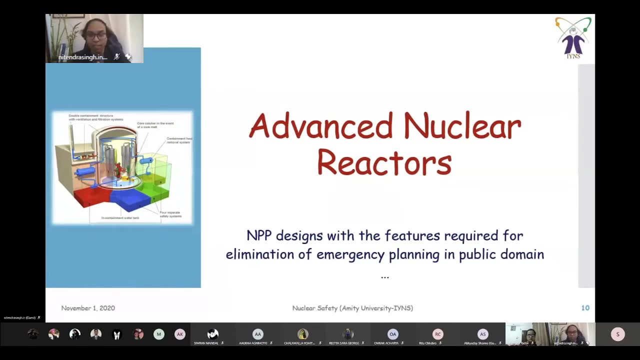 understand, as a, as the designers or the operators, that this is very important to manage because this is directly associated with the people around. so, coming to the technical part, it's all philosophy done now. what are the advanced nuclear reactor? you might have a notice that i have already mentioned. 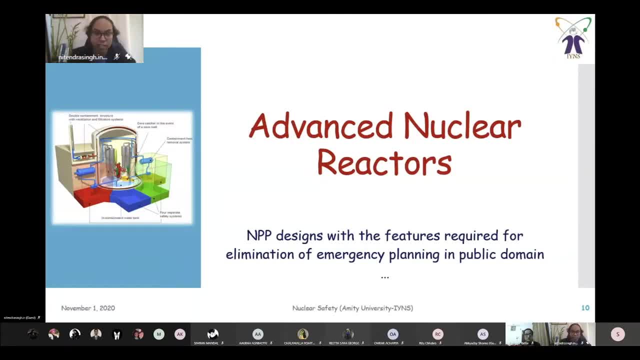 for advanced reactor, but how you will say, uh, what is an advanced nuclear reactor? so there is a you know brief definition which some designers decided it's the nuclear power plant, designs with a feature which required uh for the elimination of emergency planning in the population, the public domain, for example. so, as i was mentioning the fifth level, the off-site emergency response of 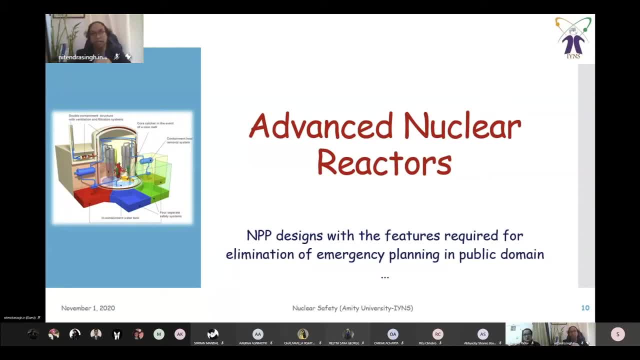 or the emergency planning in case of, you know, accident, severe accident progression. so advanced nuclear reactors are basically those designs which, uh, designers claim that they are so safe that you don't need to evacuate your people. you can make it, you know, within your city, and things like that. so now the question is: is it really? 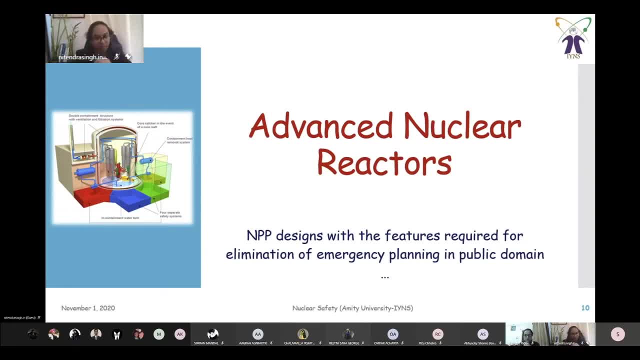 possible on, if you ask me. yes, it is very well, because, as a designer, you design all your things and you know there are many, uh, new things designers added to the um- previously improved versions as well, and that's how you call them- advanced reactor. so there are a few key aspects. 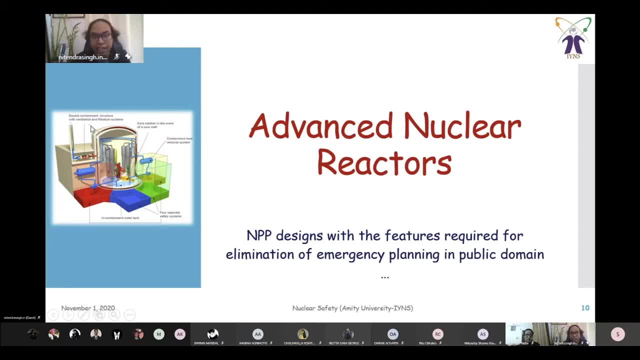 which i don't know if it is visible to you. so they added, like double containment system. they added the core catcher, uh, in the event of if the core is melting, and how to you know, collect it, cool it, maintain it. they added the containment cooling as well, uh, you know, to maintain the. 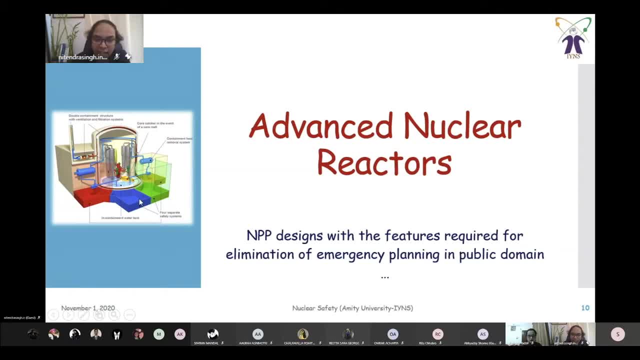 integrity of containment. they added the safe, separate safety systems for all different trains and different aspects so that every uh to avoid the common cause, failure and stuff. and they also added some some sort of water pool, extra water in case something has happened. so there should be some sort of water pool so in in different. 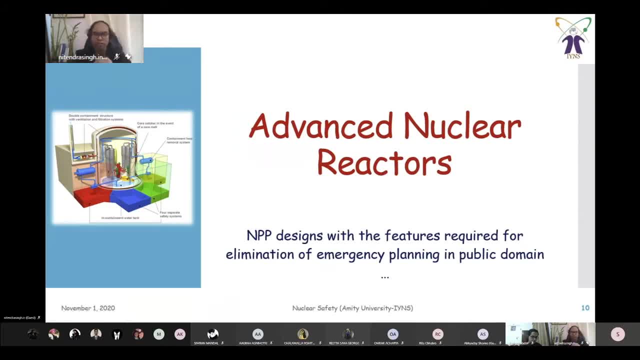 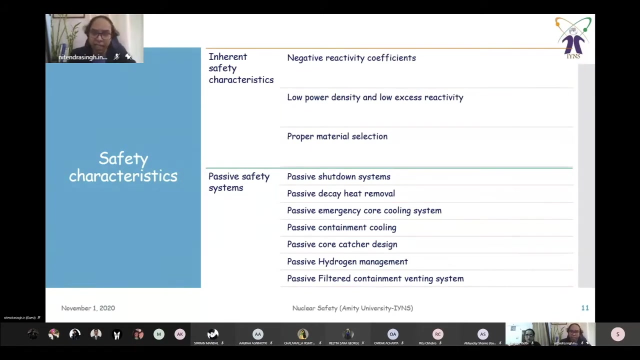 designs this, the placement of, uh, different reactors, i mean different components, may vary, but for the moment this is, uh you know, the brief about what could be the advanced nuclear reactors. so now, coming to the safety characteristics of the advanced nuclear reactors, there are two main characteristics these advanced reactors have which i want to highlight. 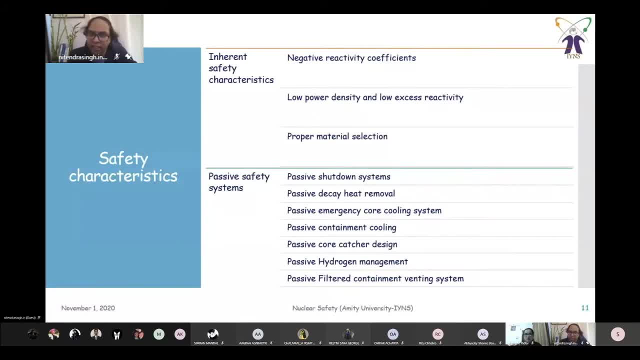 one is inherent safety characteristics and second one is, uh, passive safety systems, and these two all together take care of your plant in any situation. they- they try to, you know, give you all that confidence that your plant is safe in any scenario. so let's discuss about it. 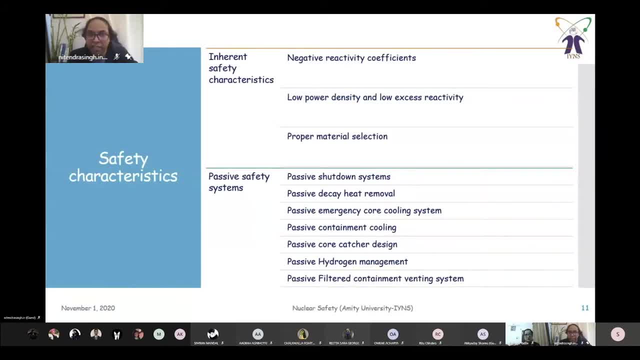 so let's talk about the safety characteristics of the advanced nuclear reactors. uh, so inherent safety characteristic, uh characteristic is the negative reactivity coefficient. you- i, i assume you- all know about reactivity coefficients. so if, in any case, there is a, some, um some situation where your fuel may try to have the different deviation, or your the, the activity coefficient. 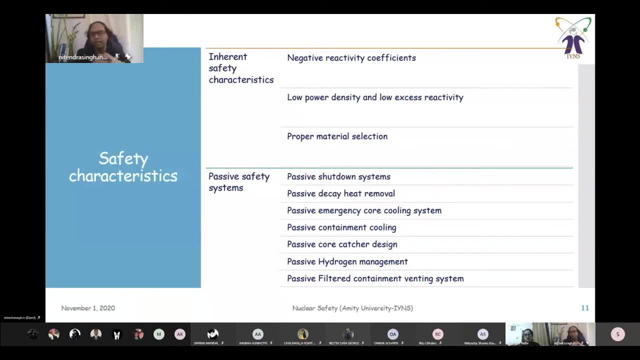 is trying to increase in uh. in any case, it is so maintained that it may try to meet that even if you combine all the possible coefficients, even then the reactivity coefficient will not go in a positive side. once it will not go to positive side, your reactor will always remain in the uh. 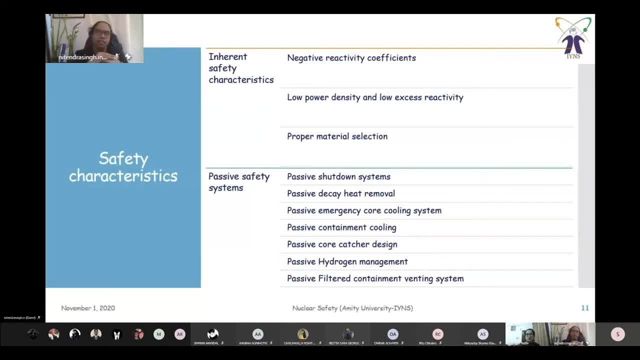 you know, inherently uncritical situation. so you are always trying to make it in, using the science or using the physics about it. you try to make your reactors of low part density, you know, uh and, and you design it in such a manner that there is a very low excess of reactivity so that even if you 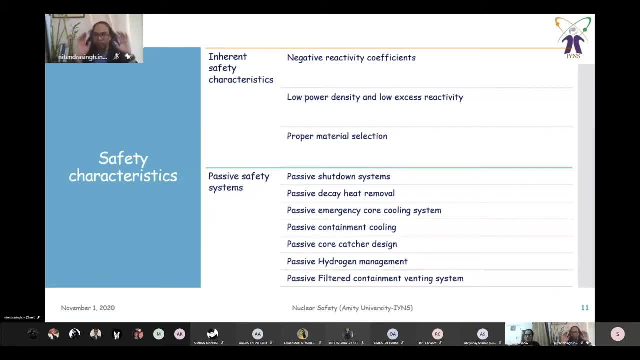 combined um the reactivity coming from the surrounding or from the structure material during the unforeseen situations. even then, the reactivity or the power will not exceed the the down power, so that you can maintain that situation in a controlled manner using your safety systems. the third, which is very important, uh, the proper material selection. this is where a lot of scope is. 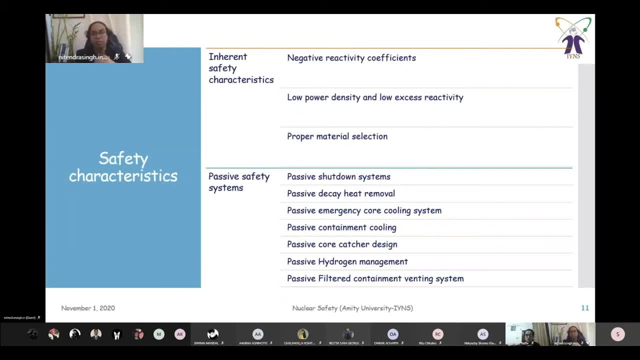 there for research as well. i'll come to that. so proper material selection. what i mean with that? you try to have material which are having high specific heat, so that if the temperature or surrounding or the fuel is in low of a certain temperature, or if the temperature is in low of some other temperature for some reason, 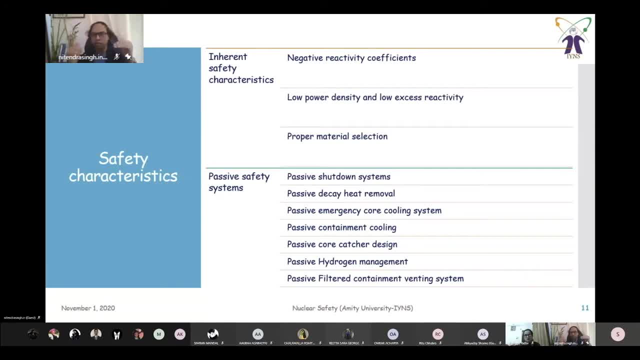 it will allow you to have a very high conductivity. you know which is very important if you want a very high conductivity. you know when it is round or round and the temperature is limited or the temperature is high and the structure of the vehicle can be maintained for a longer duration. 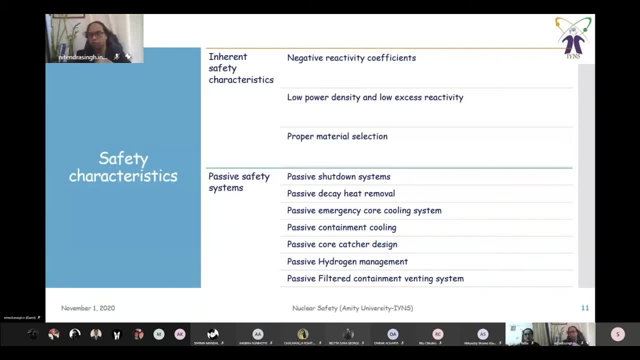 so you have to keep it that way. and if the structure is not so high, the condition of the, the structure and the integrity can be maintained for a longer duration. you should have high conductivity. so these are the inherent safety characteristics which you use, which you apply in your advanced 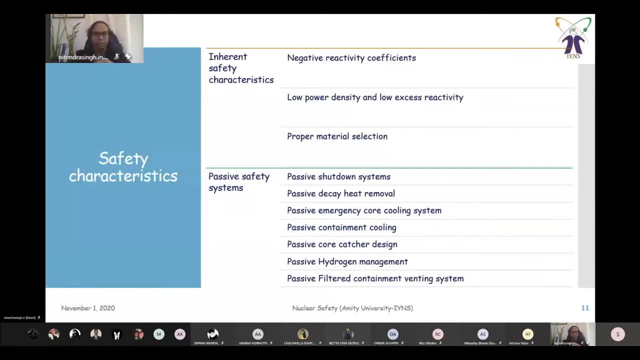 nuclear reactor based on the physics or science, i would say. then it comes the passive system, which is more of an engineering or the technology, i would say, which is of course based on the science. but when i say passive, by passive i mean that where the operator's intervention is not required. 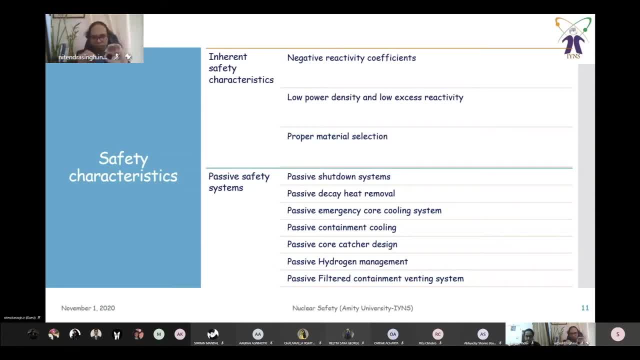 or least required. so if you, if you switch it on or if you leave it just like that, it will keep on functioning on its own and you are just like, sit back and see: okay, everything is cool. so that's what is the passive safety system. and now you might be wondering how it is possible. 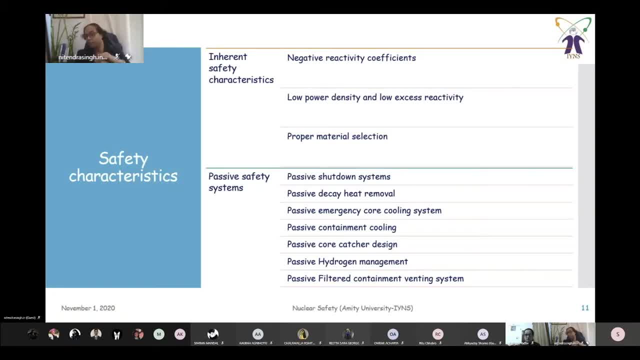 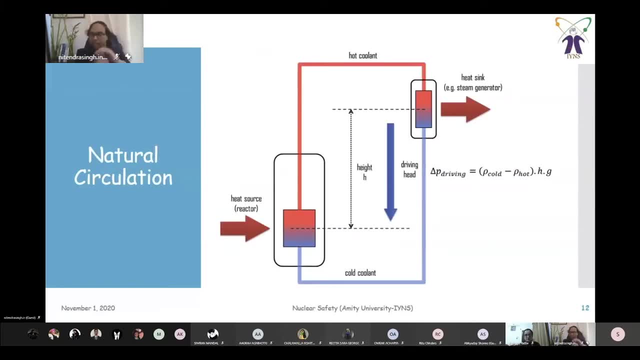 that you just sit back. there is no operator and things are taking place, so i'll go to next slide and then come back here. this is one thing i think all of you might have read somewhere or seen in some phenomenology or in some ex in experimental introduction in your earlier classes. 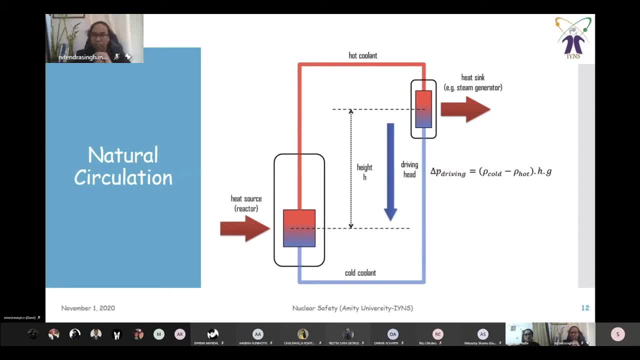 which we call as natural circulation. if you remember in our elementary classes when you used to study, like if you increase the temperature of a fluid, of, for example, if you increase the temperature of water, then its density, you know, decreases, it becomes lighter and it keep on rising high. so if you make one loop like this, for example, a closed loop like this: 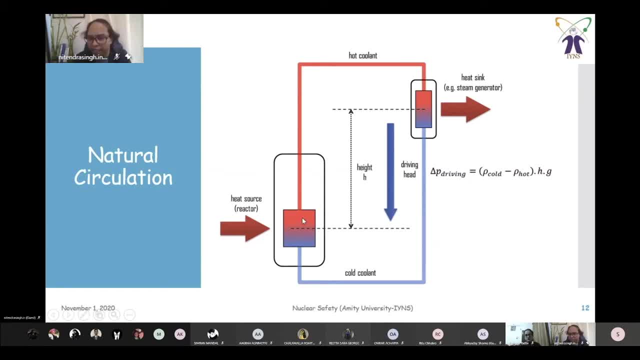 and at one point you heat it. you can heat it here, here, here, wherever you want. if you heat it, then the density of this water will decrease and, since it's a closed loop, you have a limited amount of space and limited and the fixed amount of water. so it will try to expand, try to move up, because 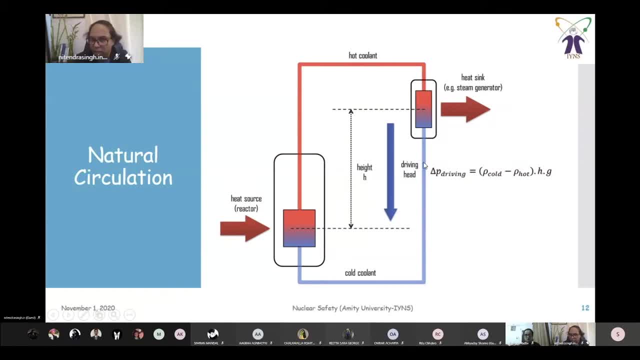 it's lighter and, this being heavy, it will try to come down and this gives a driving head or, as we say, driving pressure, or delta p driving, which basically in this kind of motion, a circular motion, which we call as natural circulation. so if, but if you keep. 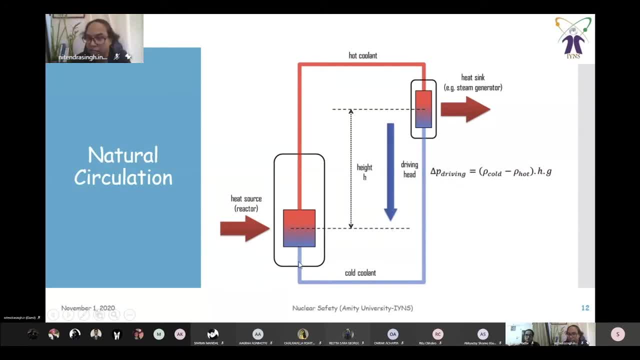 on heating this, so the temperature of entire fluid will keep on increasing. then after a while this head will try to keep minimize yourself because your delta t, your delta temperature, is now reducing. so if you want to maintain that you cool it at one point, you can use any heat sink or 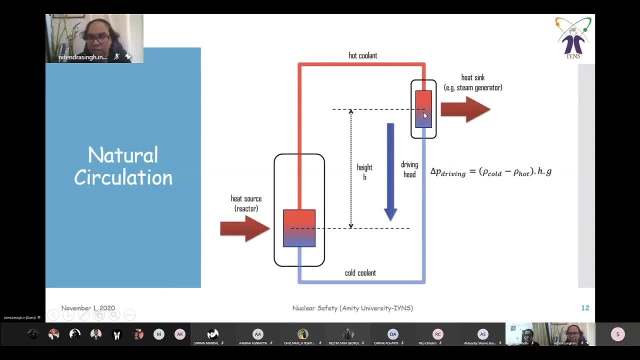 for example, steam generator or anything. so if you can maintain this kind of situation that you heat it from one point and you heat it from a different point which is at a height, then you can maintain this driving force. then, using the science, you don't have to do anything. this will keep on you. 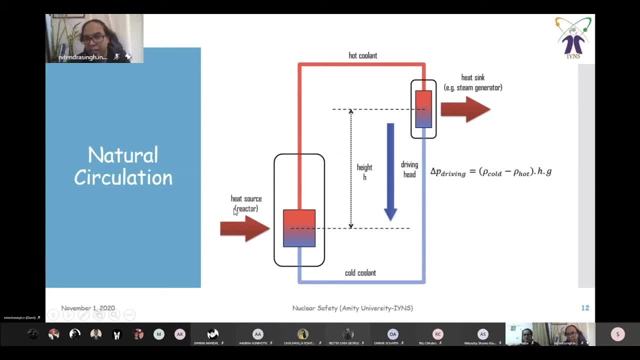 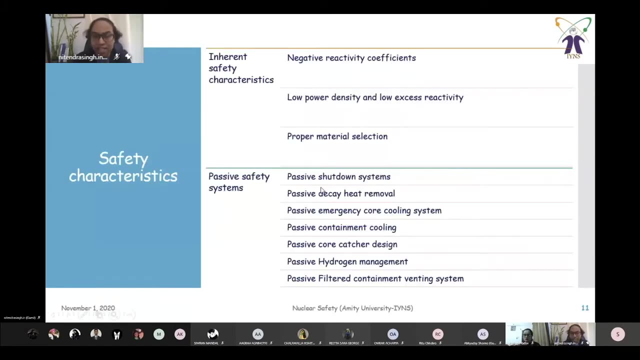 know, circulating there on its own, it will take heat, remove it somewhere else. so this is basically the phenomena which is the basis of all. so, coming back to this, you can have, like several kind of safety systems, passive in advanced reactor, which are now being incorporated in many of the designs. so then one is a very, very 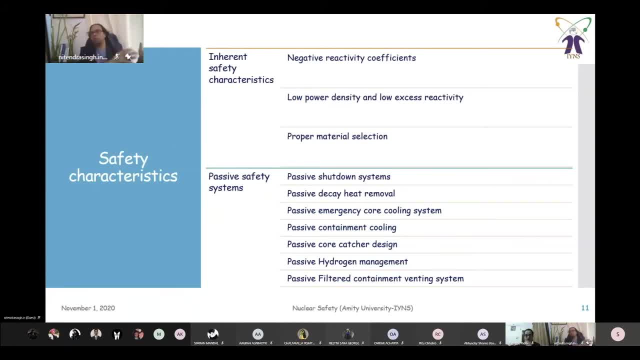 important point that you have to keep in mind is that you don't have to do anything. you have to concentrate on something. so have plenty of capacity which is enough, just like the wired awakened one or Заun, and then the hot end is shut down system. so once you shut down, stab down a. 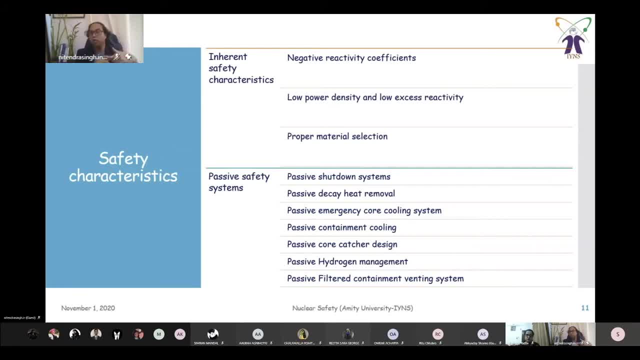 nuclear reactor you, as I mention, there is a GK heat, so even if it is shut down, you have to me cool the several components of our nuclear reactor. you cano do that using the space system. you can have a dedicated capacity key removal system which is directly. 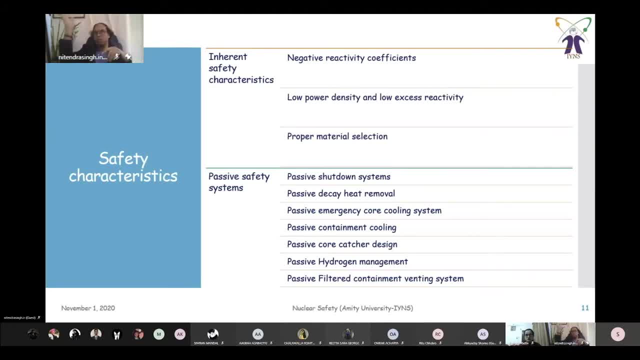 connected to your four and do you lower or outside sink through which you can cool the decay, cool the core directly? this can be one stage or two stage possibility. for example, you have the decay heat system directly connected through steam generator, through this same loop, and then you have the steam. 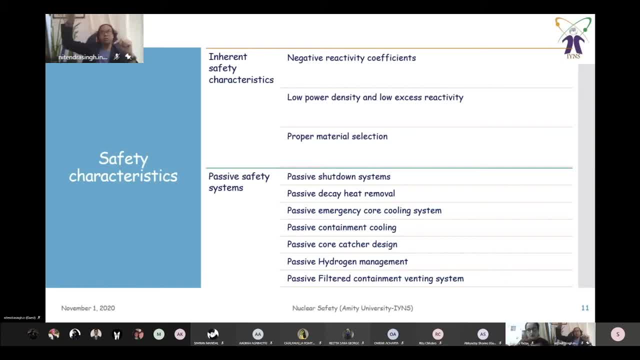 generator which is cooled via air using this same loop. so in first kind, the core will be your heating end and steam generator will be your cooling point. on the second loop, the steam generator will be the heating point and air will be the cooling point. so you know. 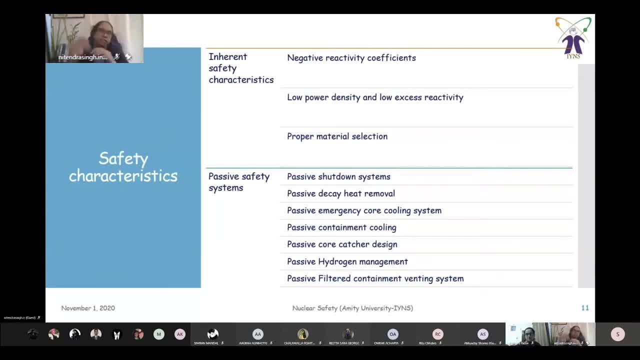 you can have a different type of coolant to maintain this sort of systems. so likewise you can have a passive emergency cooling system. you can have like ECCS, when you know when there is a loss of flow, then you need to add some water to the system and then you can. 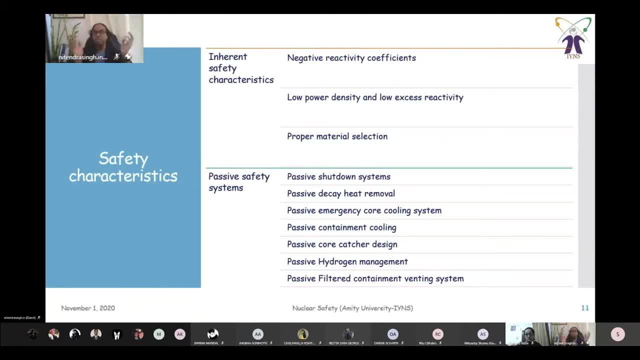 add some water directly to the core so you can have this passively earlier. you need to have you know operator should be attentive. if something is happening he need to switch it on. but you can have this sort of response passively. it is possible that you put some. 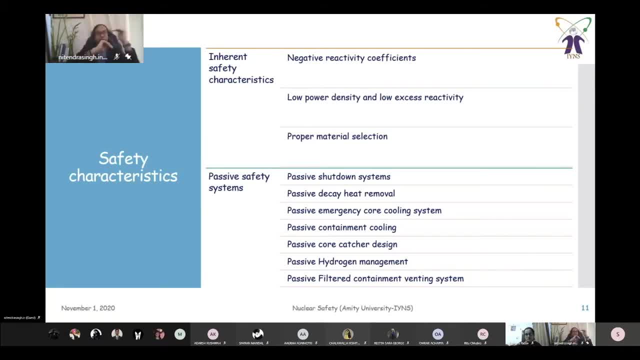 sort of passive valves which detect the situation, which detects the level of water which is going down, and then accordingly actuate the emergency core cooling system automatically. you have passive containment cooling system. you can have passive containment cooling system. so you might wonder the why we need containment cooling. this is very important. I will tell. 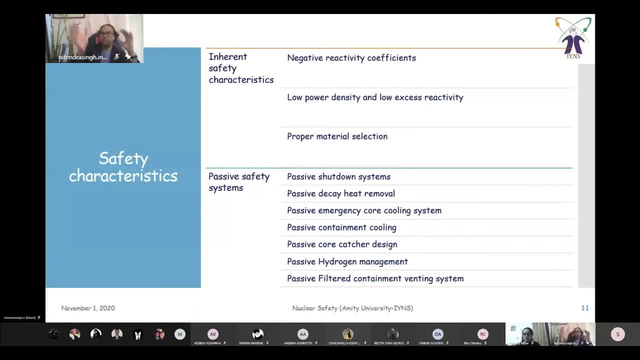 you why? so you can have a containment cooling. you have this containment and then you can have the air cooler. I mean the air natural circulation which can take the heat from inside the containment and cool it using the air side which is, like, always cooler compared to within in certain scenarios. so why containment cooling is important? you need to understand. 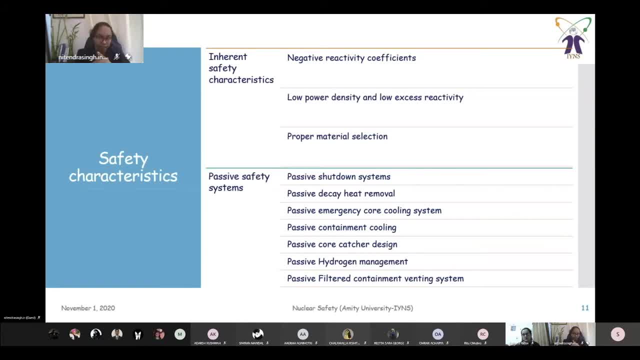 containment is made up of concrete and concrete has a lot of water. you know. more than 50 percent, 60 percent is the water content in a, in a concrete. so if your temperature within, within the containment, is rising beyond 100 degree Celsius, for example, then the water within this concrete will try. 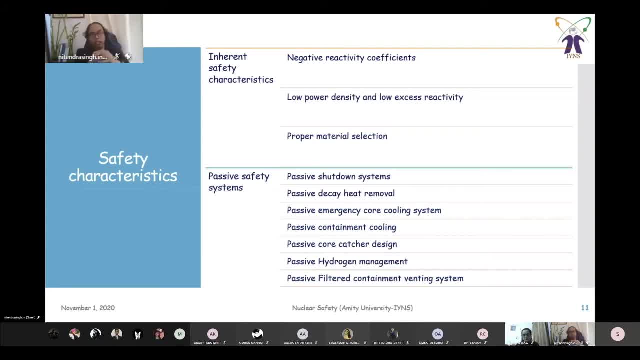 to evaporate or, you know, it will try to reduce. Reduction of this water within the containment, within the concrete, will reduce the strength of concrete and if, for example, if you remove all the water, it will crumble, because it will be nothing but the, but the collection of stones only. so somehow you need to understand that. 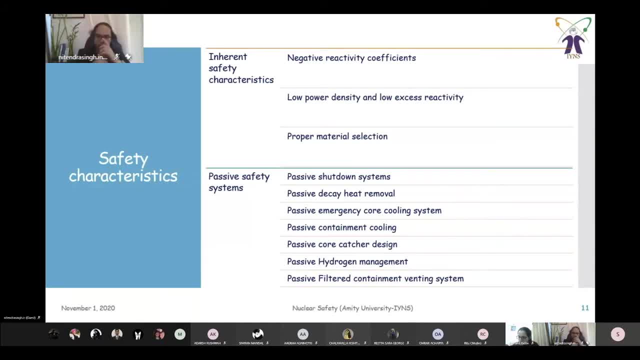 your containment should also remain cool, so you can have this passive containment cooling as well. And, as I was mentioning, core catcher is one of the key components of containment cooling and it is a very important part of the process. So you can have this passive containment cooling as well and, as I was mentioning, core catcher. 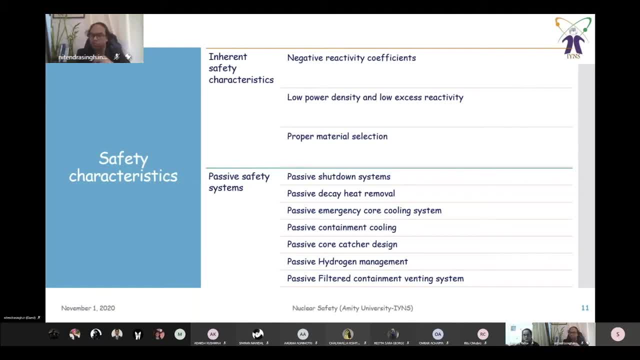 is one of the key components of containment. So core catcher is one of the key, key aspect or key design feature for all the all the advanced reactor. in fact, all three mentioned below are the one of the key features of all the advanced reactors. So core catcher is something where you collect all the molten core and you try and maintain. 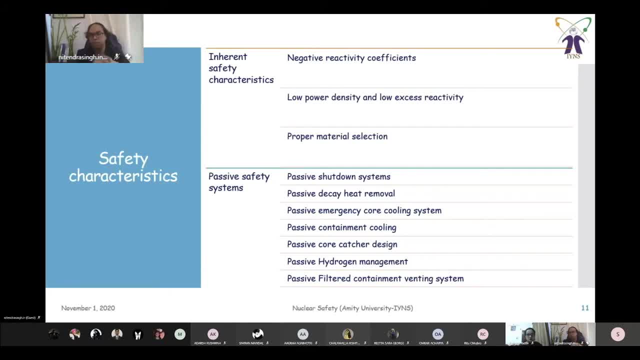 it, try to cool it and maintain it within the containment so that no radioactivity can go out. and similarly, you try to have passive hydrogen management. This you need to understand from where this hydrogen came, just like that. So it comes from the structural material I was mentioning. if, if you are not able to cool, 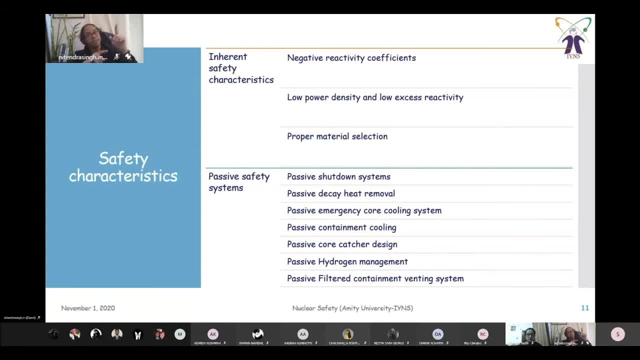 the fuel, its temperature will increase. when its temperature will increase the temperature of the clad which is usually in thermal reactors it is, it's a zircoloy or it has ZR- zirconium- in it, So that material will also heat up and its temperature will increase. 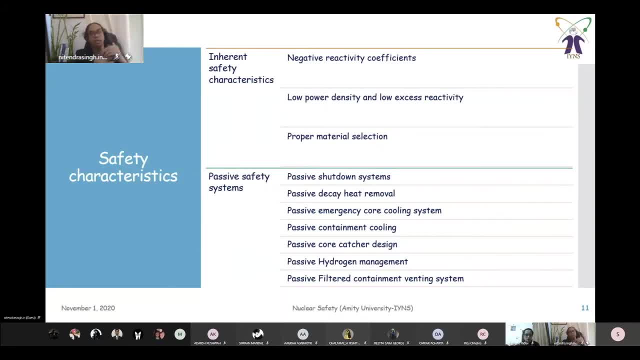 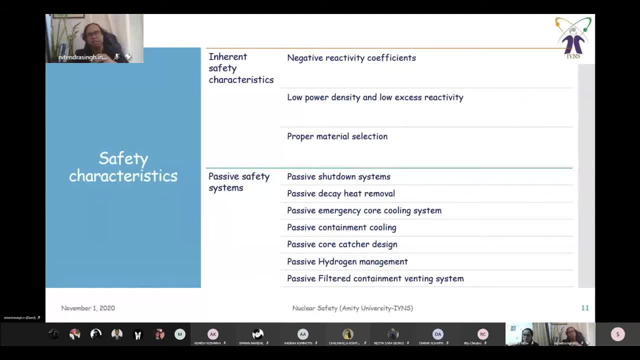 is the most. in most cases it at that temperature. when it interacts with the surrounding, it gives the hydrogen, it reduces to give the hydrogen and that hydrogen gets collected within the containment and it's risky. Why it's risky? because the hydrogen is inflammable, you know highly inflammable and it may catch. 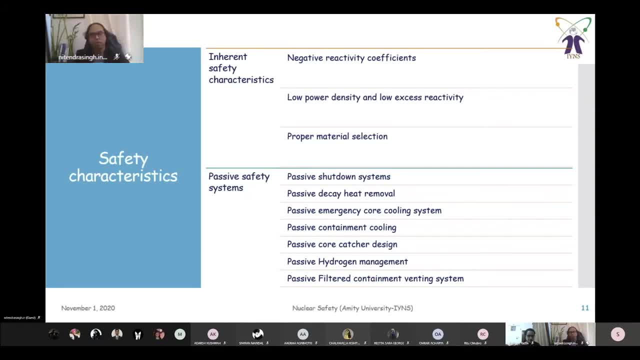 fire in presence of the hydrogen, Of course you have a lot of oxygen and when steam is coming in such scenarios, so it could be very risky. In fact, if you, if you don't know, I want to tell you: in Fukushima, the explosion which occurred in the containment on top, it was not a nuclear explosion, it was actually the. 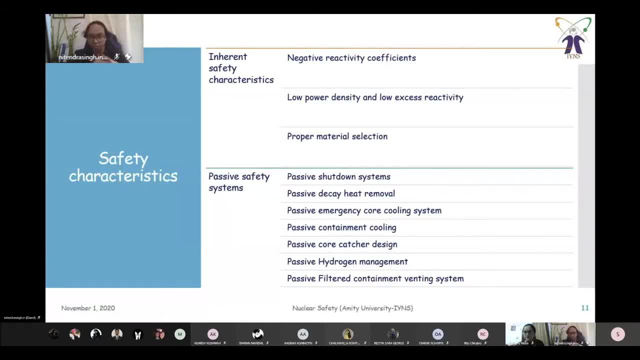 hydrogen explosion which occurred because of the accumulation of the hydrogen. So you know hydrogen which, which knew of the, whatever containment they have, they didn't have hydrogen, Not much, but whatever they have blew it off. So hydrogen management is really important in that sense. 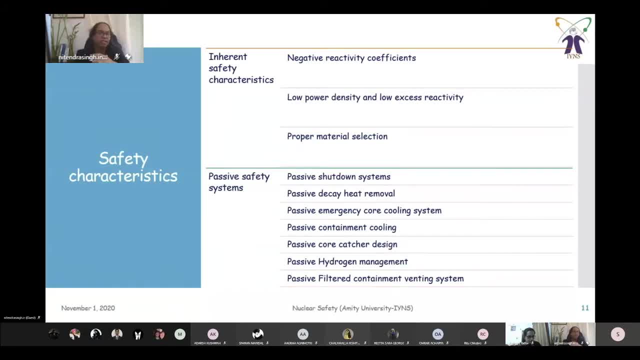 And also we need to have filtered containment venting system. So this is very important in this case. for example, if you have a lot of radioactivity within the containment and you, it will keep on pressurizing this containment, which will again add the stresses on the concrete. 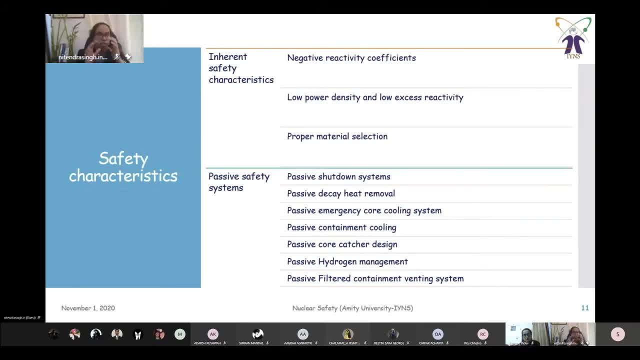 So you want to, you know, reduce that stress. So you want to, you know, reduce that stress On the concrete so that your containment integrity can be maintained. but if you release all this radioactivity outside, then there is no meaning of you are not maintaining your safety, you. 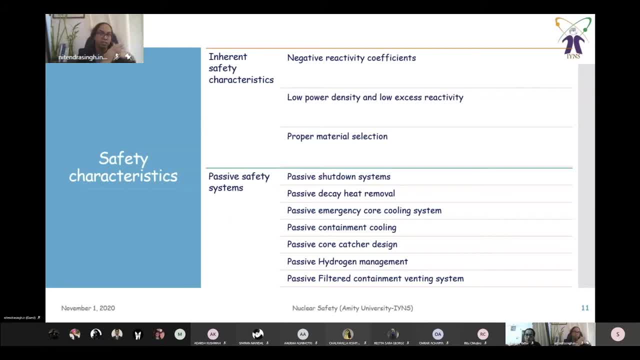 are not, you know, respecting your last confinement, safety function. So somehow you can do that by filtered containment venting, which is like you filter out the radioactivity material But you release the pressure outside. You know, you release the gases outside but you maintain the radioactivity within the. 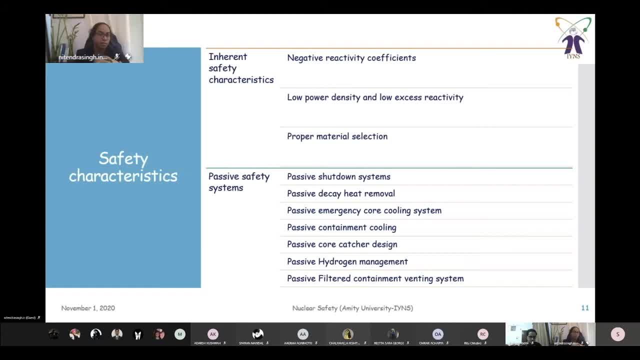 containment. So this is possible and they are now being used for, all you know, advanced nuclear reactors. So to give you some quick example of one of the safety system you can have, like many. but I'll give you one quick example of cold catcher with a nice animation. 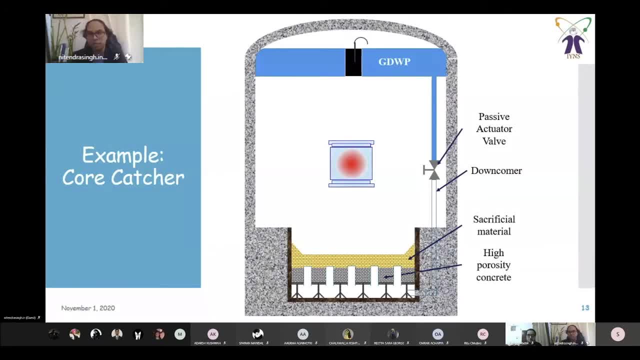 So this is one of the advanced nuclear reactor which India was, India is making or in constructing in a few years it has been approved. So in this case we design one cold catcher which looks something like this, which has you know some, some structure, and you have some sacrificial material to it and you pour. 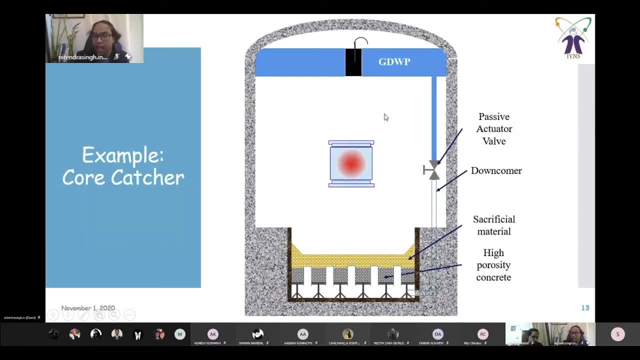 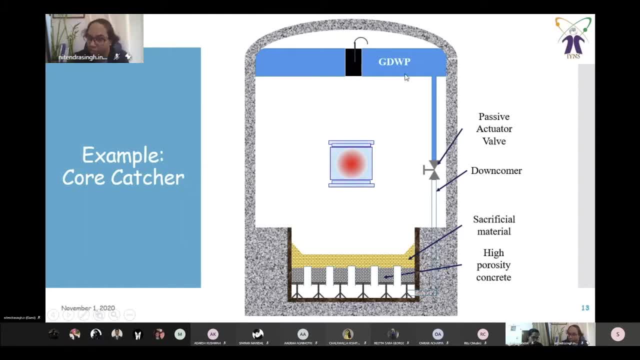 So this is your core. for example, And they have, as I was mentioning it, In all the advanced reactor they have made a provision of water pool somewhere. So in this reactor the water pool is on the top. Why it is on the top? 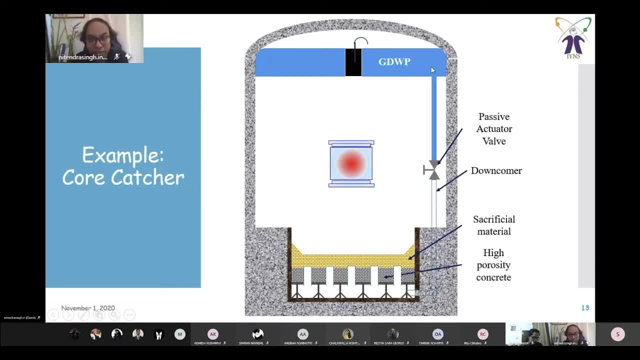 Just to make sure that everything can work passively, because if you have water on the top, then through gravity it will automatically will come down. So you have this core and due to some, some reasons, some, some sort of this accident is happening and some core is melting. 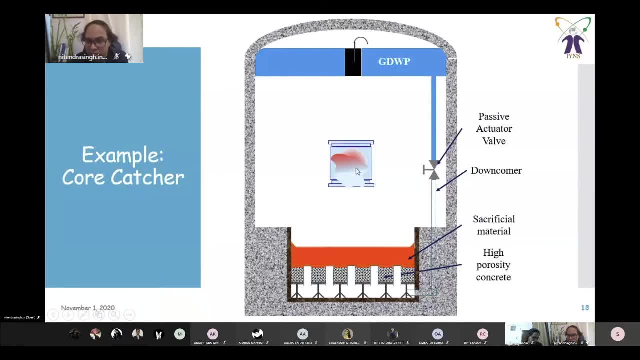 will breach the structural component of core and melt is coming down. it interacts with sacrificial material and then, you know, due to decay heat, it forms the melt pool like this. now, everything is passive. there is a passive actuator wall which will detect it and it will release the water. 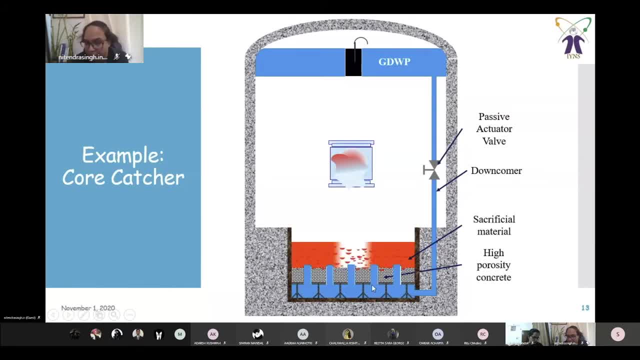 supply which will form the water from the bottom and it will then passively go through the melt and it will convert into the debris which will then automatically be cooled- you can see here- through the water pool. and this, this steam is, you know, can be collected within the containment or 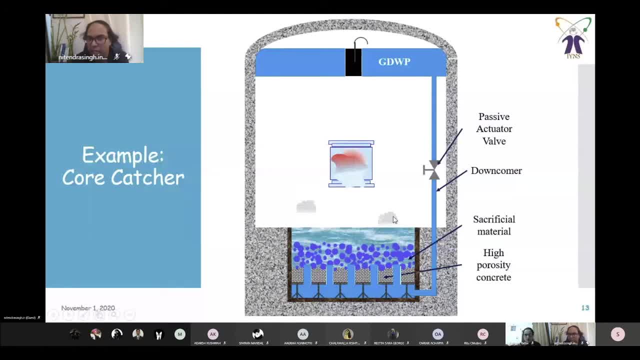 can be released through the filter containment system, and that's how you maintain this, this passive core catchment in a nuclear reactor. so this is one of the design which we, which we did recently. and now you should question one thing: okay, this is the scenario in a reactor, but how you basically 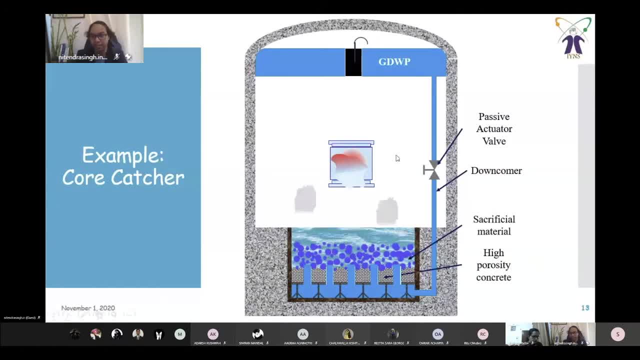 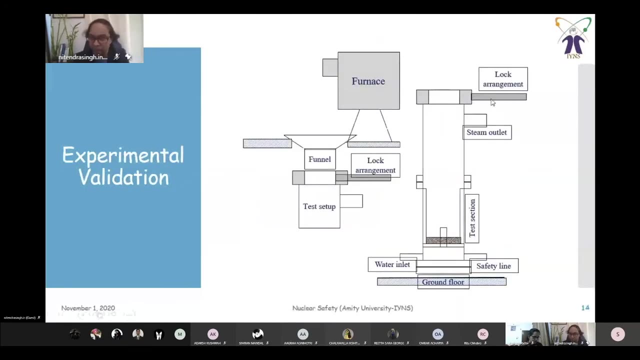 design it. so to design it like this is a concept you design. you need to validate those concepts, which you can do using the experiments. so how you recreate such scenarios in the experiment. i'll give you an example of this, which is like this: so instead of uh core, you use furnace to 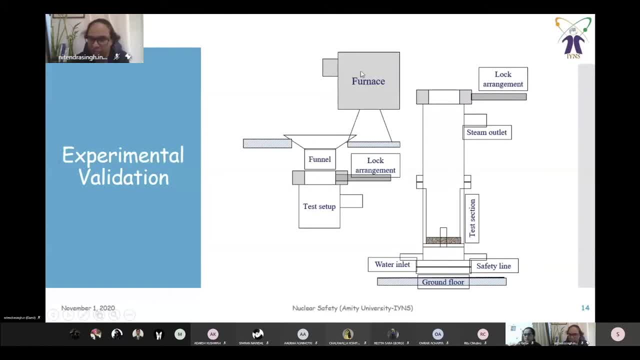 generate some, some simulated material or whatever material you feel like, to study the properties, and then you transfer it into the test setup. so this test setup is here, which is like this. so this, this is a two stage animation, okay, so in one case, you basically generate the melts, which is then poured through some. some makes sense. 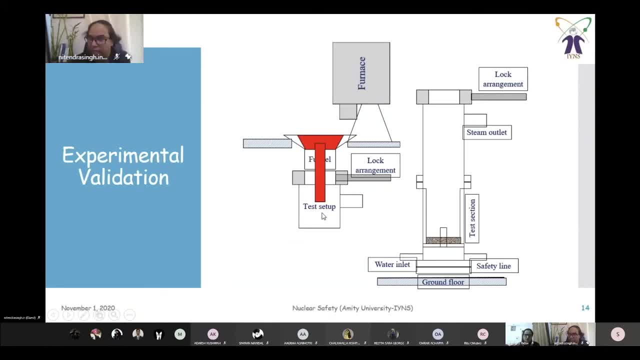 some final arrangement or something into the test section, and this tech section is basically now your uh reactor scenario. so, as i was mentioning there, the melt comes the reaction and then, by the time, the product is finished. and so there are two stages. you are having its own test process, you want the test set section, and once you have made the test, 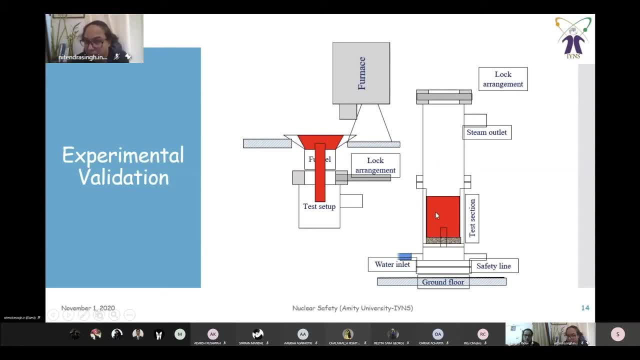 down. it interacts here. it makes the pool and then you add some decay heat to it, then water releases into it and then it forms the debris it cool, is down and you know. you collect all the data, all the measurements you do and you study, so you design this concept, you validate those concepts. 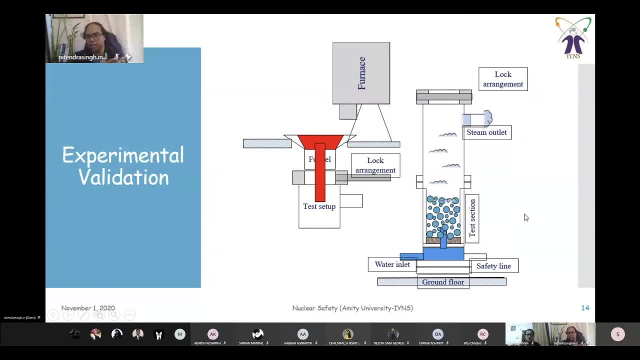 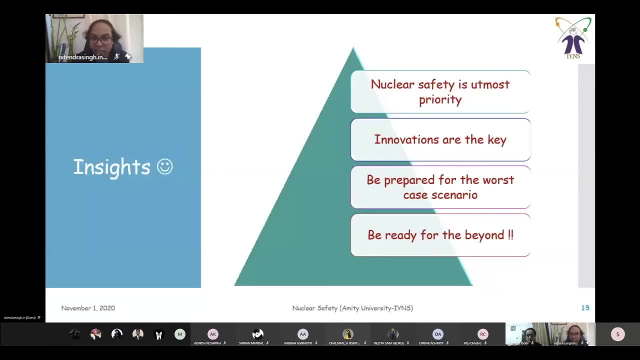 and then you use these concepts directly into the reactors. this, this is how you do it. so, concluding my presentation, what is most important for us is the nuclear safety, and nuclear safety is utmost priority for the nuclear industry and, as i was mentioning you like, innovations are the key. you need to come up with new ideas. 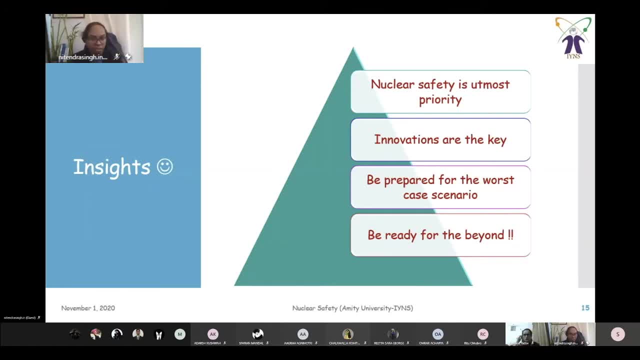 new possibilities, new technology to make sure that you take care of different kind of situation, and by a different kind of situation i mean you need to be prepared for the worst case scenario. whatever you can think beyond, you need to be ready for that beyond. so that's how you try to. 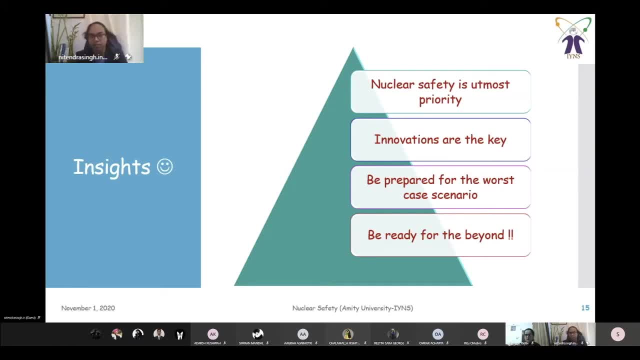 maintain the safety in all the advanced reactors. you have different kind of systems, different kind of technology, and this kind of technology will be a necessary part of your recovery training. They work all together and somehow you try to minimize the human interaction or human intervention or the operator's intervention to it so that, even if in unforeseen scenario, 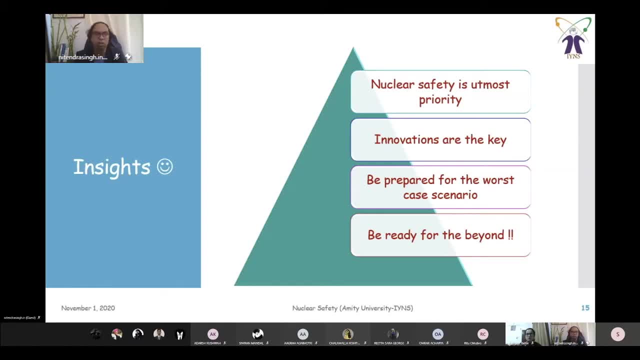 where operator is not available, or operator is not able to reach, or something has happened that there is no access to the control room, or something like this. even in that scenario, your reactor will remain safe on its own. that is one of the main feature of any advanced 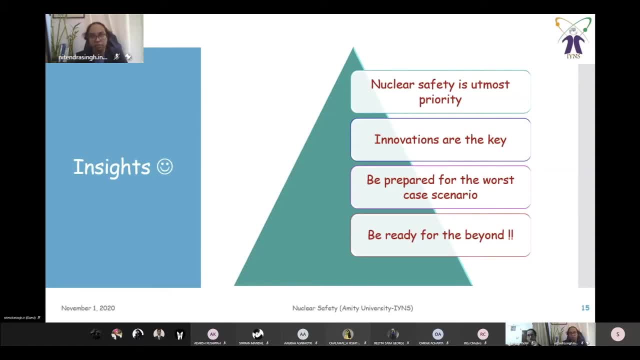 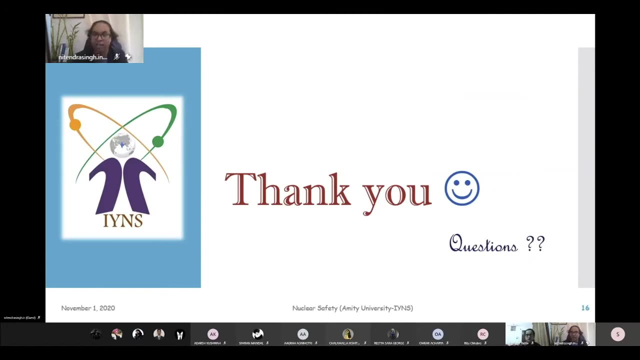 reactor which will be coming in future, which are already under design and some are already under constructions, and a few of them are already operating now. so that's all from my side. thank you so much, and if you have any question, I am ready to answer. Thank you. 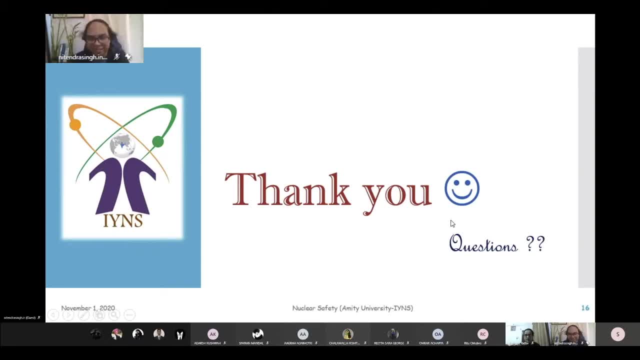 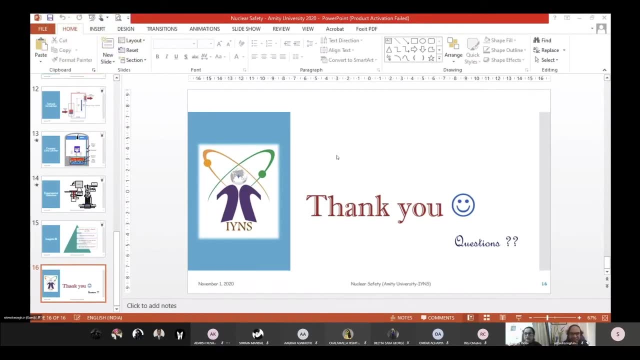 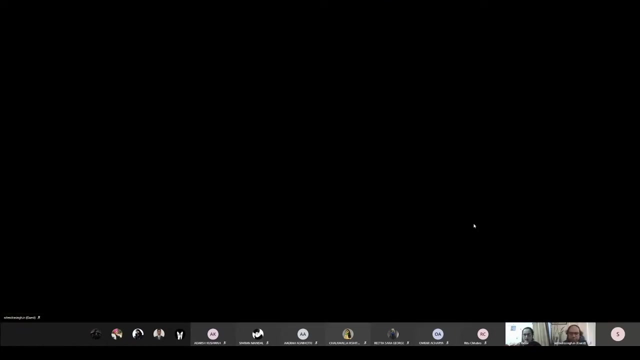 Thank you, Mishel, I have an explanation. I think Keeush has one question. Yes, please, Sorry for the echo, Keeush, you can unmute yourself and ask your question, if that's possible. I can read out his question. he says that you were talking about a source to connect and 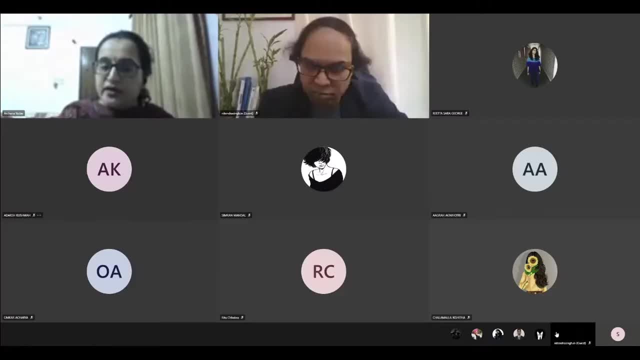 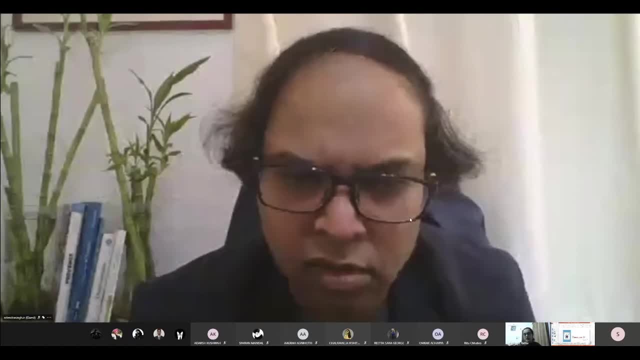 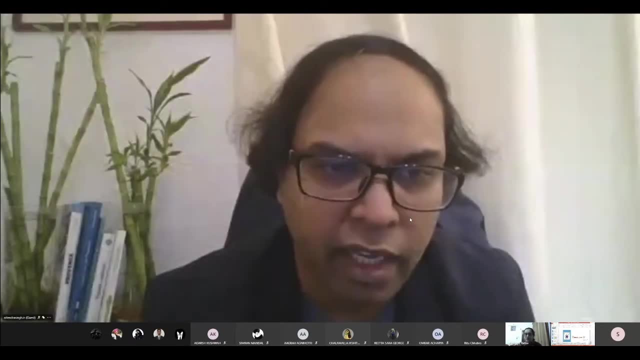 During the initial part of the presentation where you were discussing about that neutron is to be bombarded in the nuclear fuel section. Ah, okay, Yes, beforehand. Okay, okay here. So yeah, of course I am talking about all nuclear reactors. 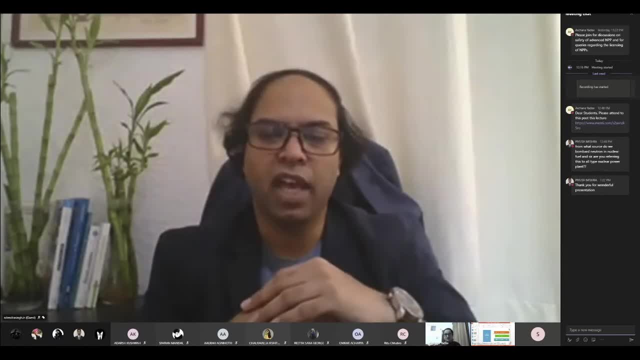 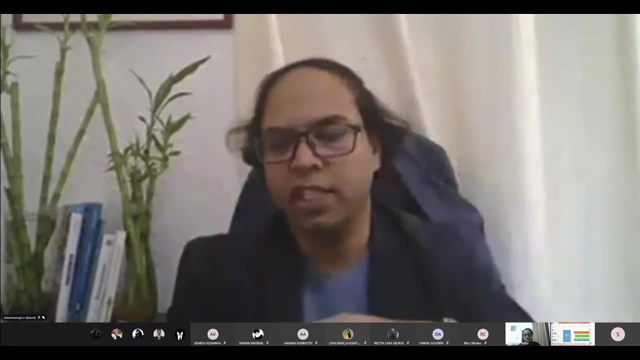 Basically, you all know you have this nuclear energy because of you have a nuclear fuel and you bombard it with neutrons, Then only it initiates a nuclear reaction and it continues the nuclear chain reaction and you try to maintain that chain reaction. So yes, I am talking about that particular physics phenomenology which occurs in all 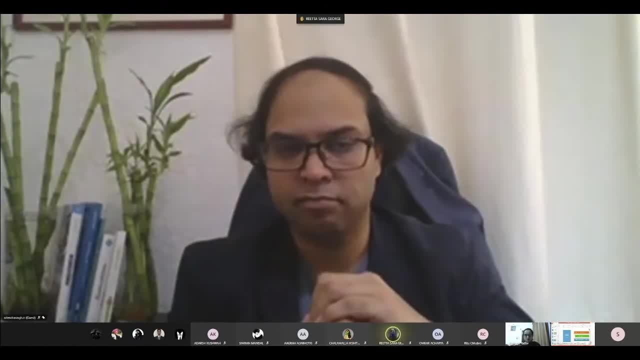 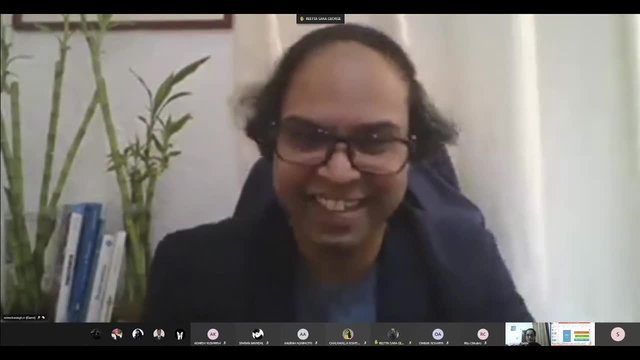 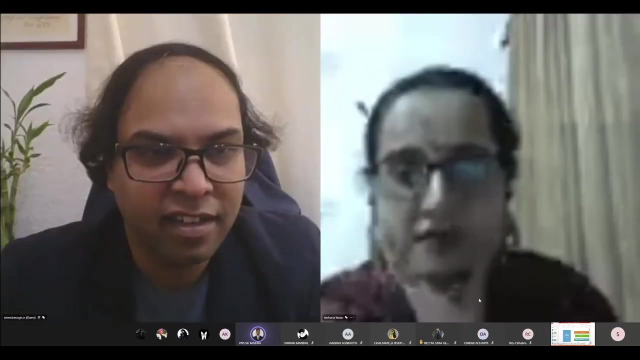 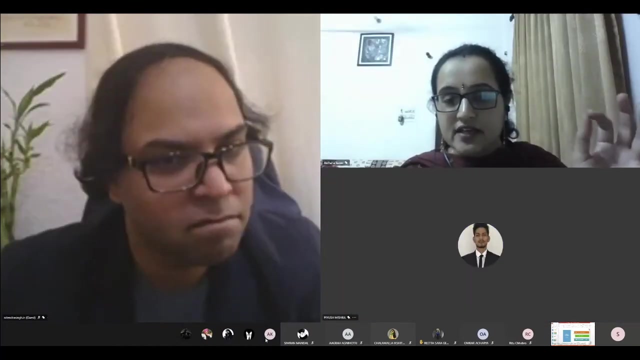 nuclear reactors. Okay, If I may, If I am able to answer you or if I have understood correctly, Yes, I think he will write the response Outside the source of neutrons. Am I audible? Yes, Please go ahead. I think he is asking about any external source that we are keeping for neutrons. 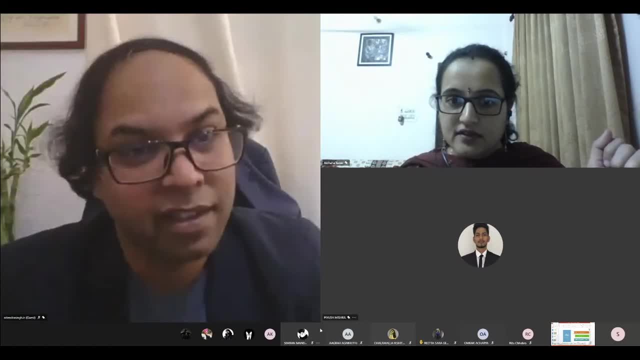 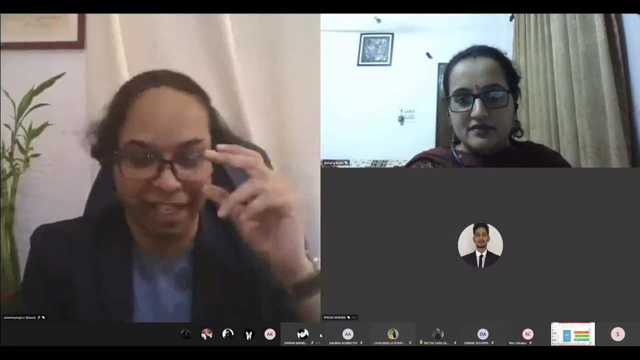 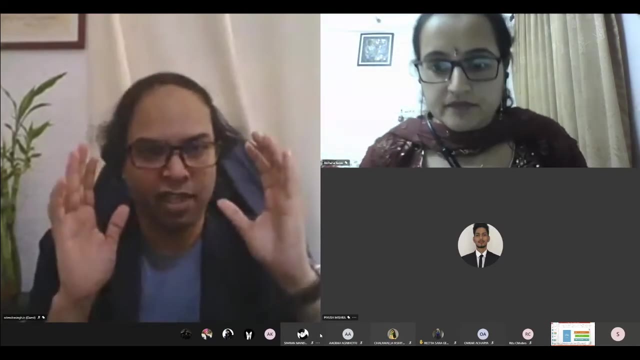 Ah, I see, Yes, ma'am, Yes, so you were asking about a very primitive scenario. Okay, so once you go, once you restart, once you start a nuclear reactor, for example, you have constructed a new reactor or you have put your new, very brand new fuel inside. 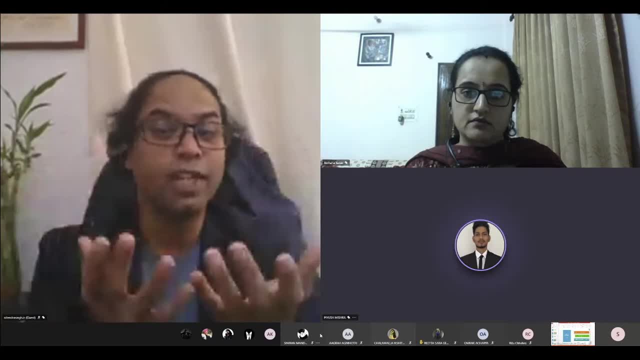 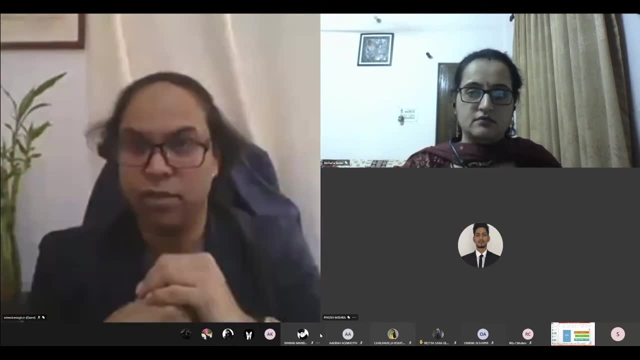 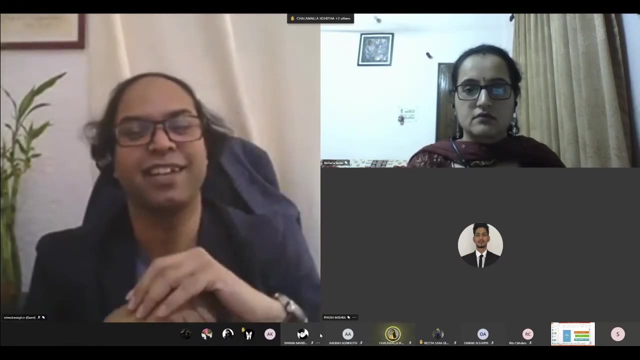 the inside, the core, entire core is new, entire fuel is new. there is no source, only the fuel. So there is no neutron in the surroundings. So you need- Okay, You need- first neutron. I would say you need first neutron to start the first nuclear reaction which will then. 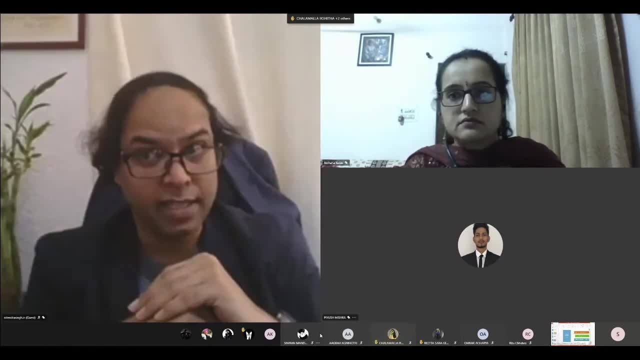 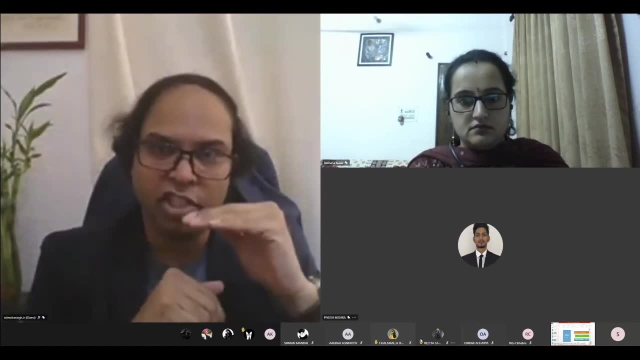 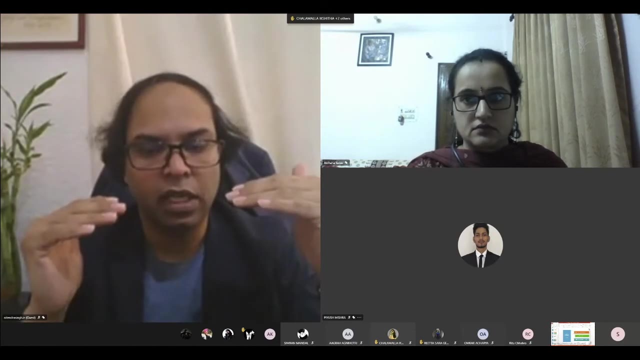 generate the further neutrons. So, yes, except for the Russian designs, in all nuclear reactors you put one source below the core, which which gives you, which gives, which do, or which performs two functions, mainly One: it. it gives you the initial data to the control room, which you know, okay, how many. 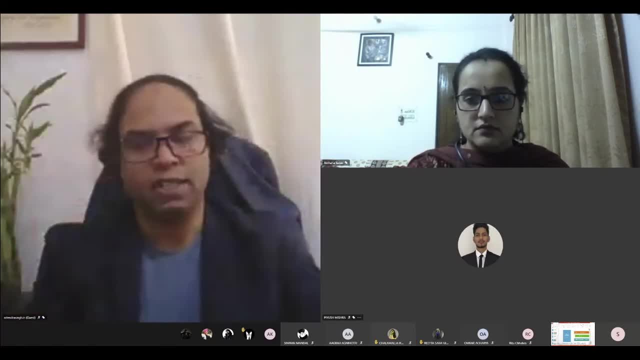 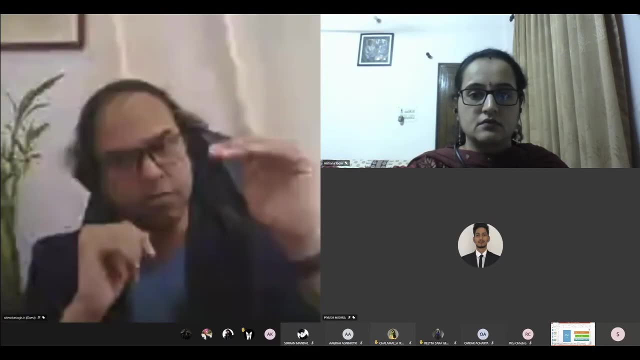 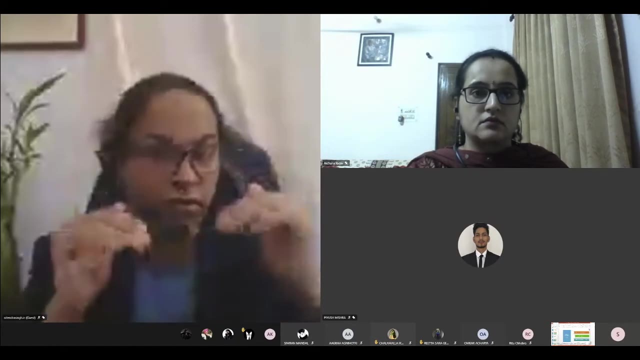 electron, how many neutrons are there? what? what is the surrounding and everything. And then, once you once this neutron source start, or once you remove the, you start removing the, the controller, for the first time. I'm talking about when you start removing the. 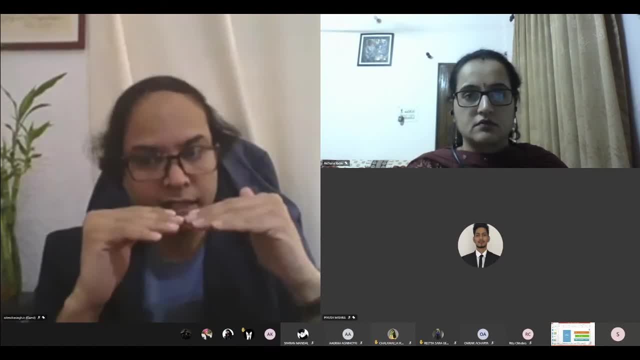 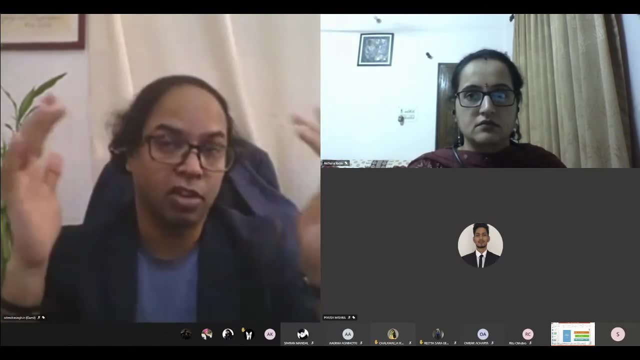 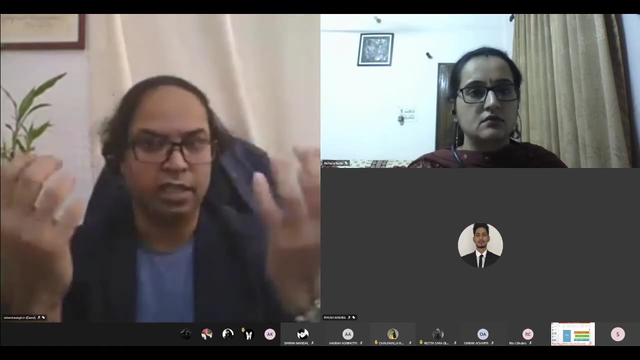 control, or very little, very little. then it interact with the surrounding fuel and then it gives you the first chain reaction, Okay, The first couple of chain reactions. um, then it increases the neutron flux. Then again the surrounding keep capturing this increment of neutron flux likewise, and 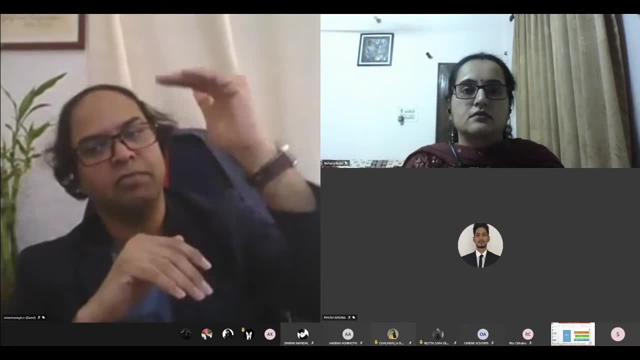 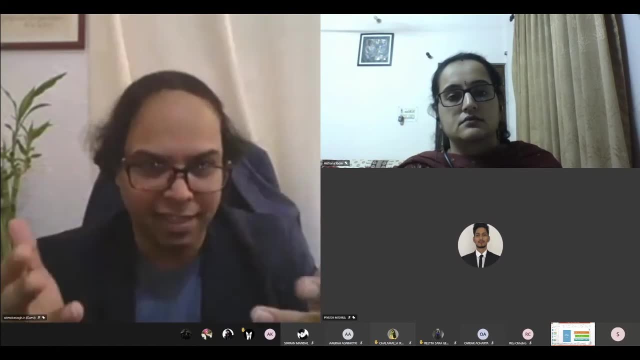 then you attain a different power. This is what we call this criticality of a reactor. or the reactor went critical, or you can say the reactor actually started. So yes, in the beginning, all the reactors. all the reactors, except for Russian designs. 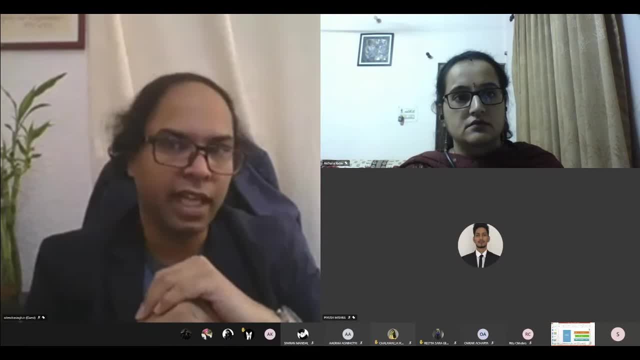 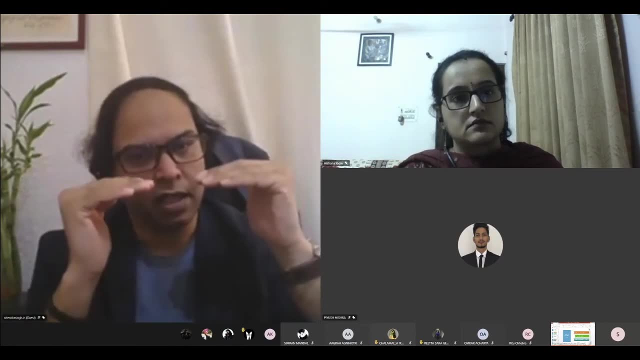 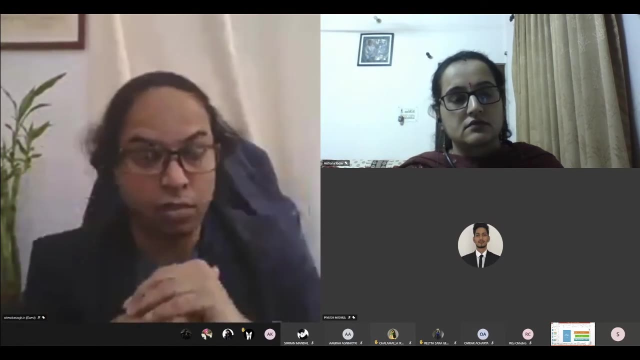 you have the neutron source In Russian design. they use different technique. uh, for that very a lot of experiences needed. They. they play with the um, uh, with the control rods. So they play with the control rods and then somehow do it. 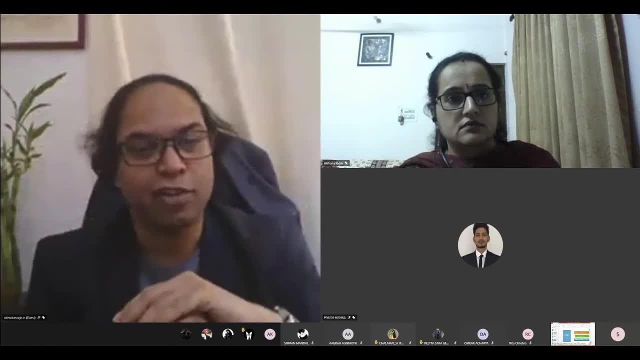 So it's a different technology, I would say, but except that all reactors have this initial neutron source. Later on they don't need it because, uh, you never remove your all fuel. So it's a different technology, I would say, but except that all reactors have this initial. 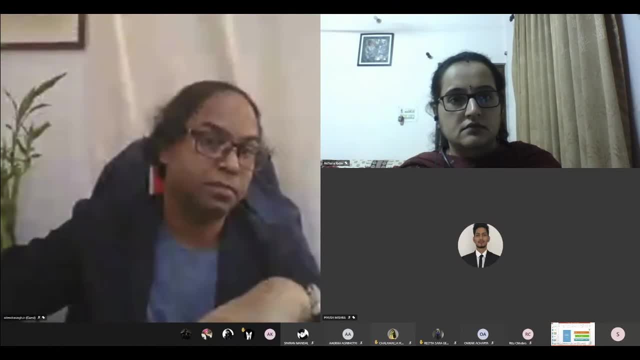 neutron source. So it will make sure you are all fuel out of your reactor. So there's always uh uh, some, some neutrons are there. Even if you shut it down, there is a certain level where neutrons are still there, decay. 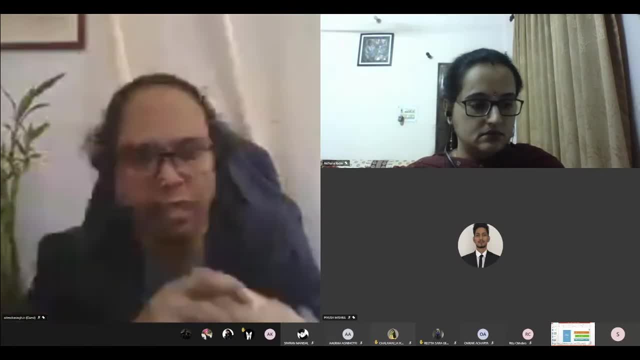 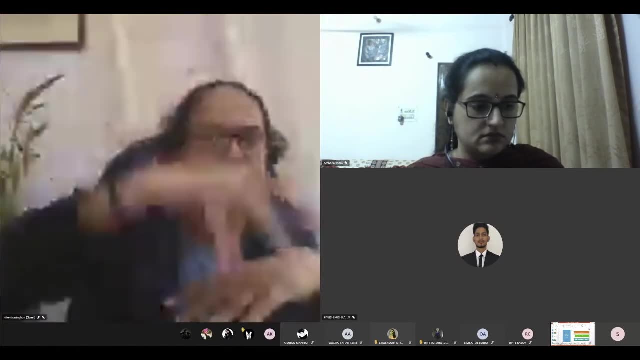 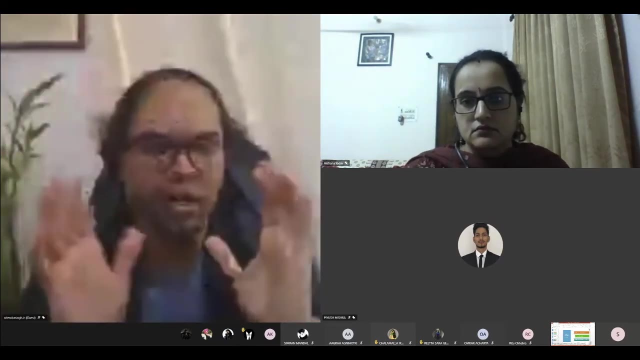 is still there And then you can continue, Even if you refuel it. when you refuel you don't refuel your entire. pour out, entire pour in. you remove one third of the core. So the rest of the core is still having new neutrons, somehow it's. it is a maintained 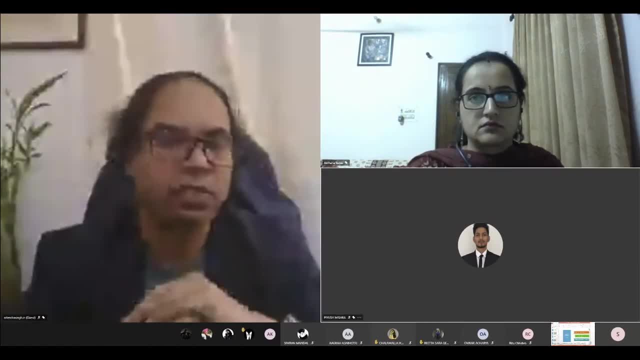 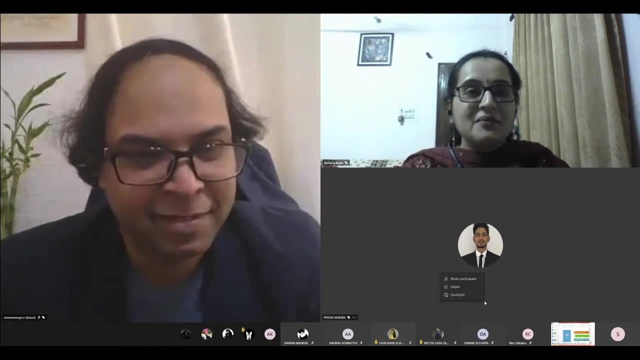 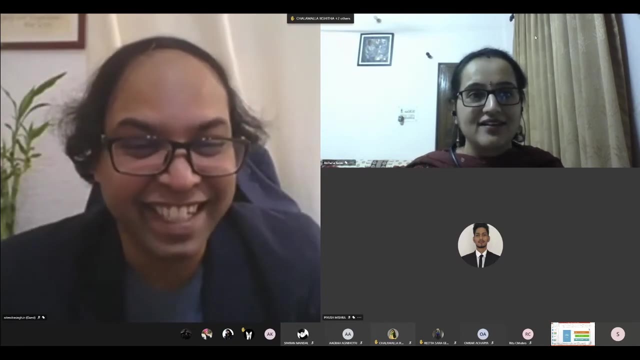 Um, so yeah, but yes, in the beginning you need that source. now i have understood and i think i am able to answer it, but now i am in a state of doubt. how do they do it in the russian reactors? yeah, that's, that's a cute thing. that's a cute thing, it's, it's a, it's a, it's a new technology. they always say. 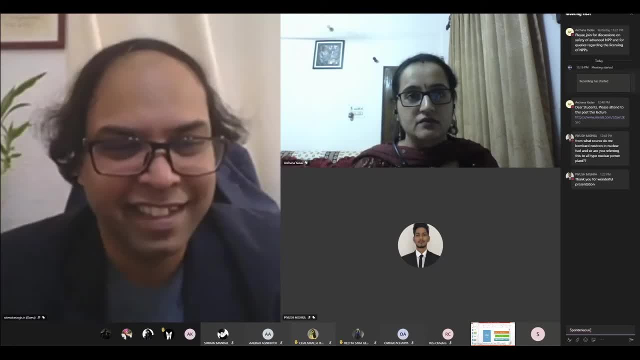 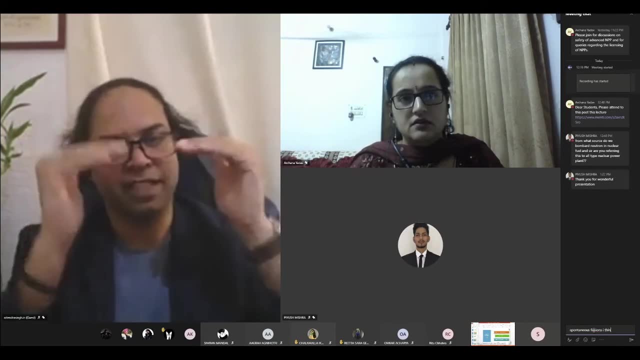 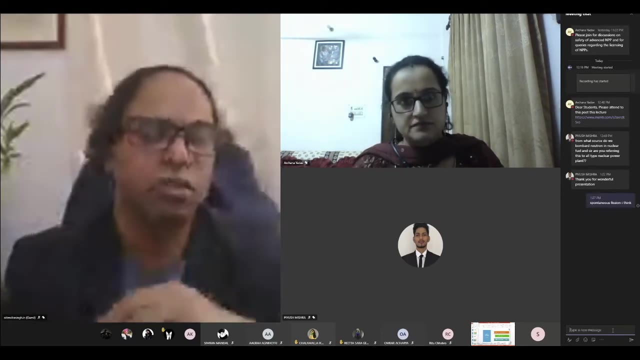 but in russian designs they do that. they don't disclose it, but they, yeah, they don't do it, but there they play it with the uh, with the control rods, because uh, one more thing is they also use two different kind of control rods. earlier most of the reactor were using only one kind of control. 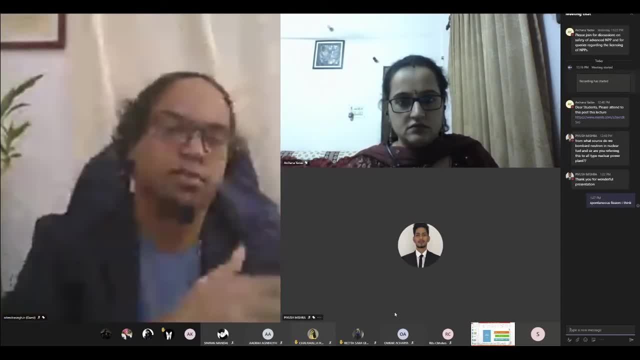 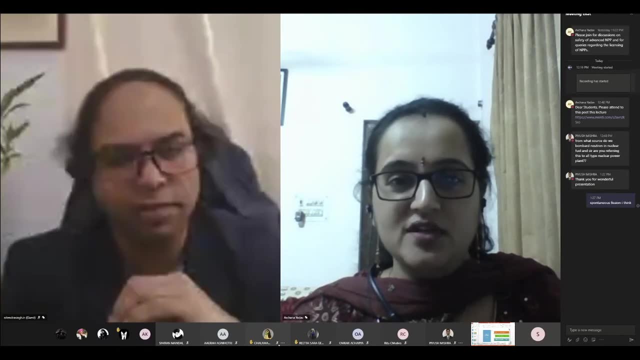 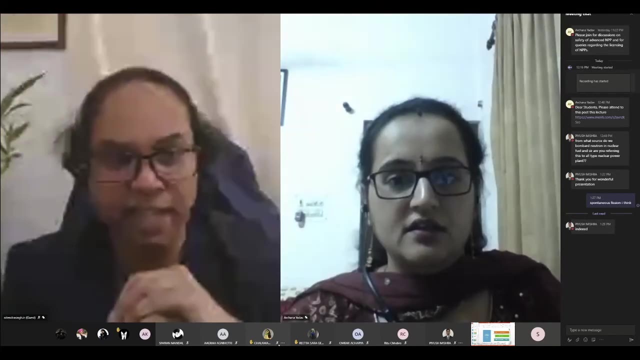 rods, but now all the advanced reactors. they use many types of control rods, so, using that, they they could play so. spontaneous vision: yes, this is the one region which which adds to spontaneous finishing. they maintain but, uh, as i mentioned mentioning, you, don't do it because you need a. 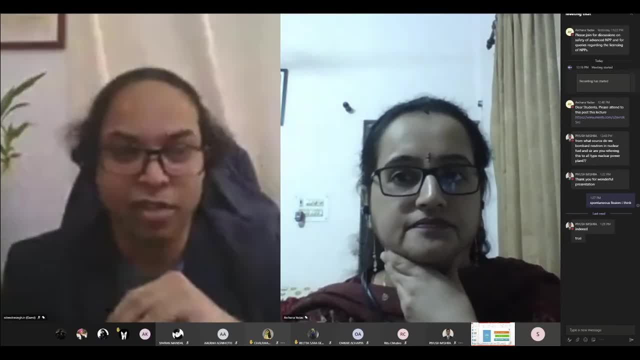 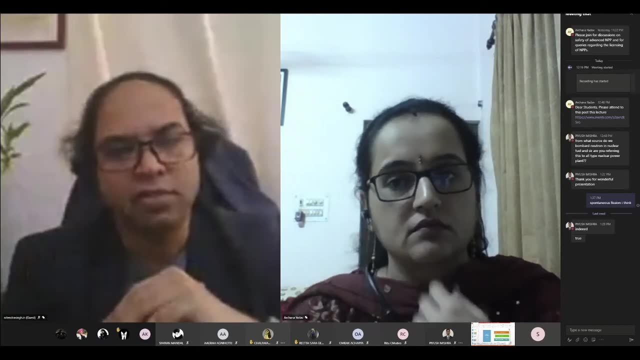 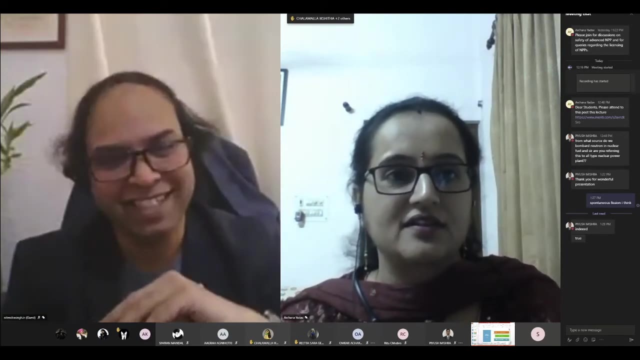 lot of experiences for that, so no other one, because if there is some deviation and then you don't want to, uh, put yourself in that situation, so so only russians do it, to be very frank. but nobody else in the world do it. everyone uses the, the, uh, the neutron source, and 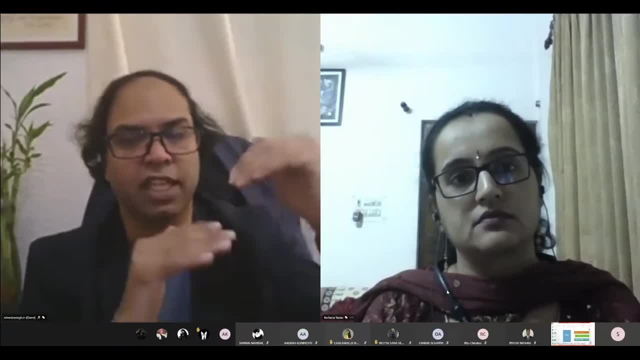 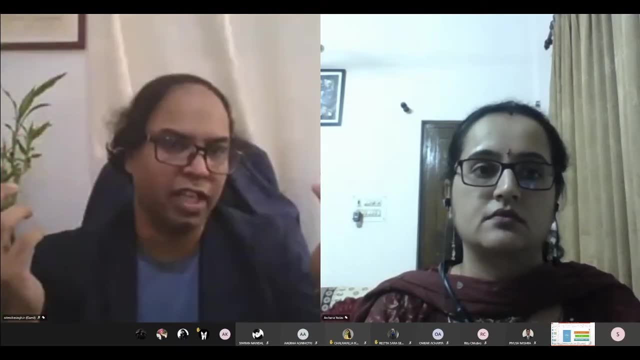 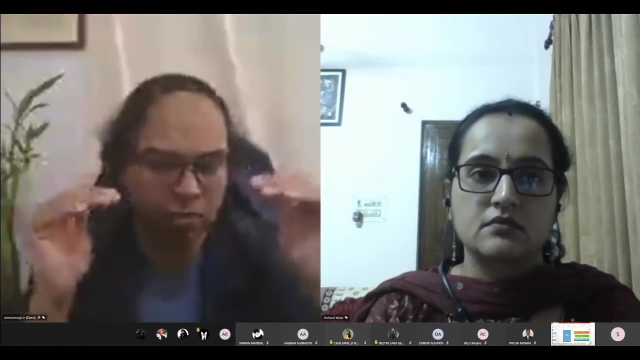 i i like that neutron source concept because, as i was mentioning, you have this to make sure your all data acquisition or your surveillance system is working fine. you can you have the initial data of of the source which can tell you: okay, this is the minimum neutron flux we have through the source. 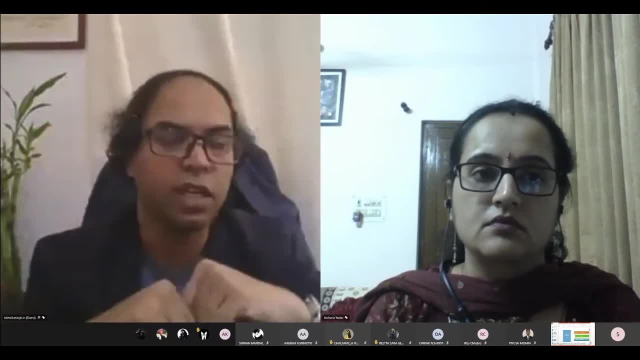 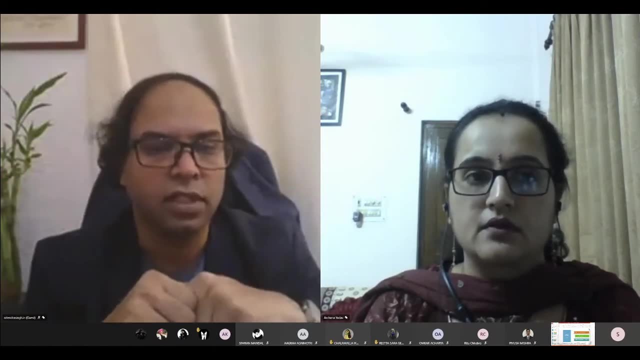 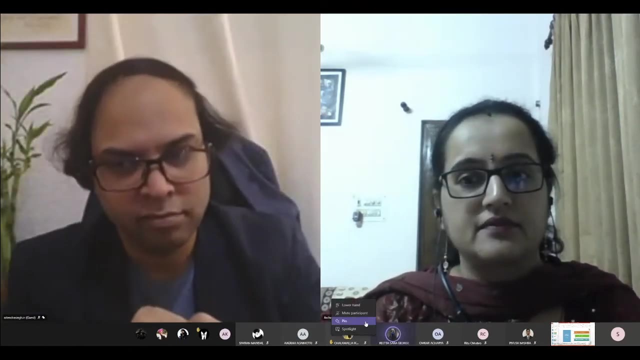 if any deviation is coming because of the increment of control rods, then you can actually detect it. so that's how they do. i think next rita can ask her questions. uh, okay, thank you, sir, for the wonderful presentation. first of all. uh, so my questions, like i have two. 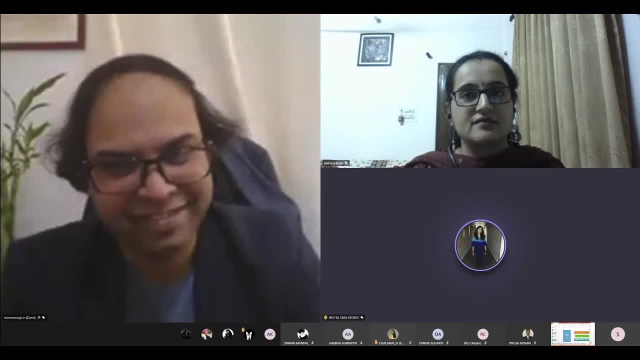 questions, and both of them are mainly from the licensing part of the nuclear facility. so the first one is like: uh, how do, what are the differences in the licensing of a nuclear facility in a country like india and the other countries, which are the superpowers and the other countries? 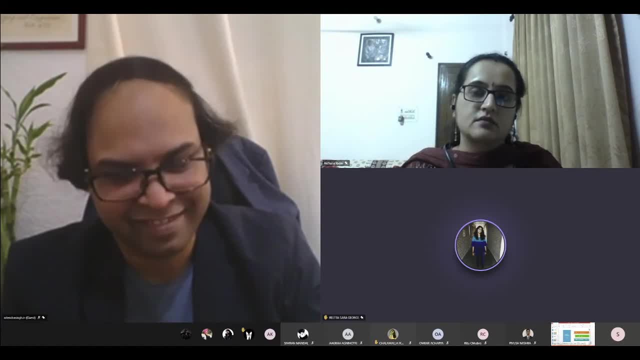 superpowers like US, France, China and others. And my second question is that the licensing of a nuclear facility like the generation 2 reactors and between the generation 3 and 3 plus reactors, like just you mentioned, that there are some safety aspects in the generation 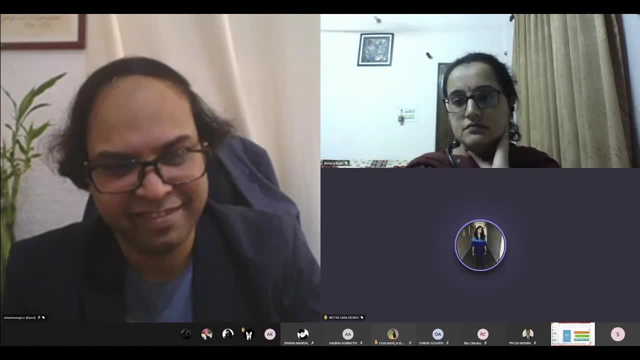 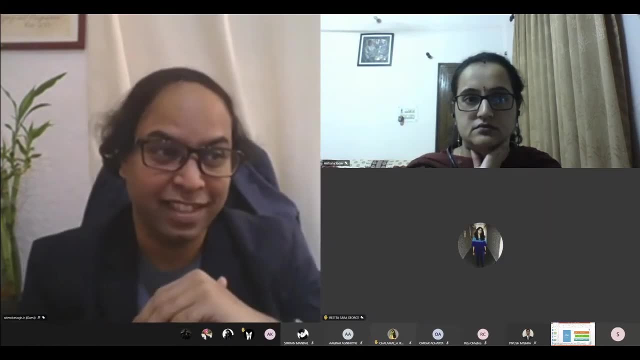 like generation 3 and the advanced reactors. So what are the differences between those? Yeah, so coming to your first question first. So when you say some superpowers in terms of nuclear technology, I count India as one of them, Because you might not know, but Indian, 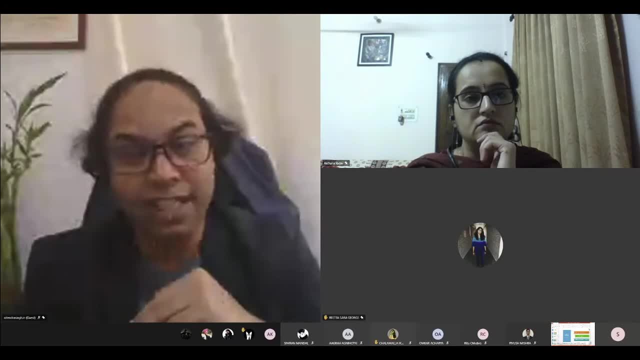 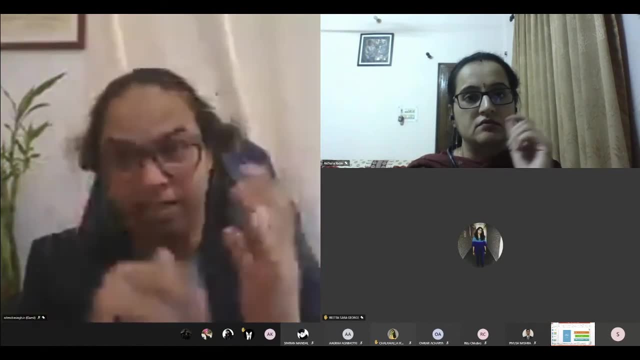 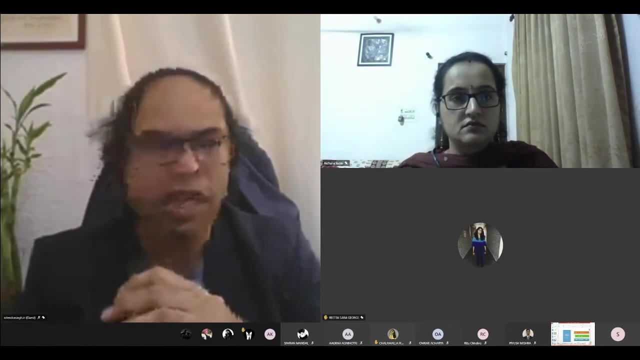 nuclear technologies are one of the best in the world. Mark my words. So yes, I cannot differentiate in that sense. But yes, there are certain superpowers And I think that there is a certain difference in regulations And of course there are differences in licensing. 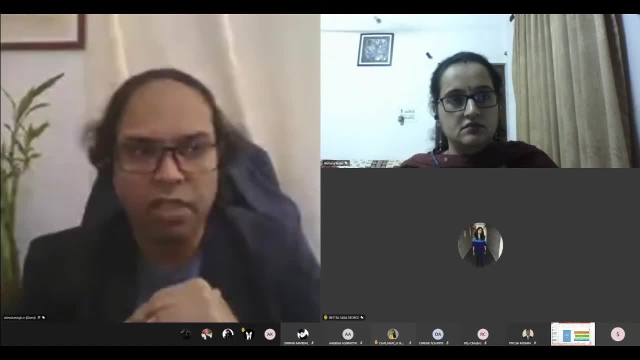 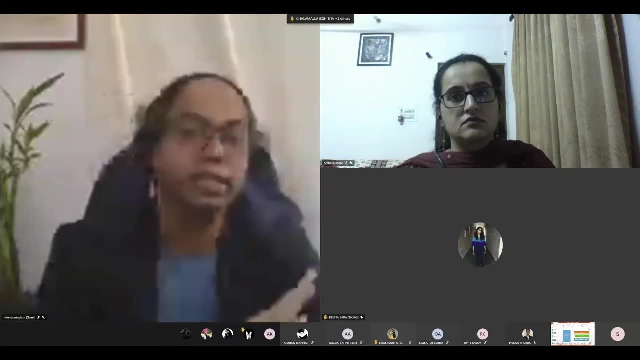 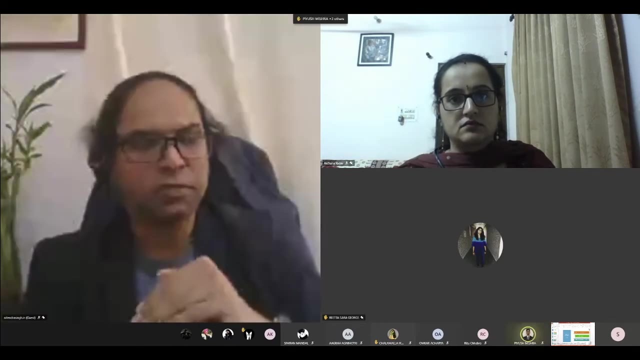 processes. It depends, It varies from country to country, Like you cannot say like US and France has the same, or France or Canadians have the same. They all have different aspects, But few key aspects are still the same. For example, everyone have the you know process. 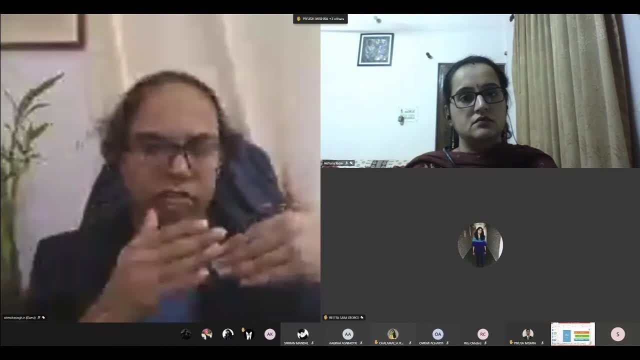 of licensing in a very specific way. So, for example, if you have a nuclear facility, you have to have a very structured manner. You initially give the concept for the review. They review the concept. Then you give the preliminary design. Then they review the preliminary. 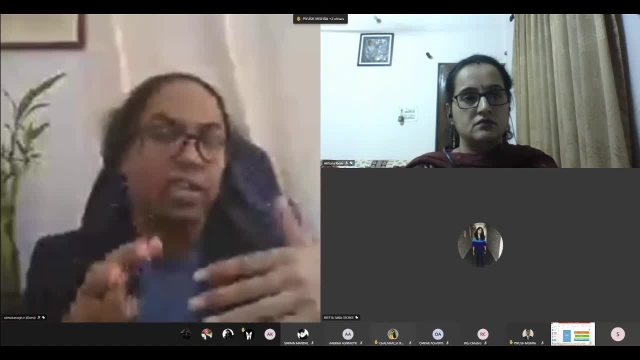 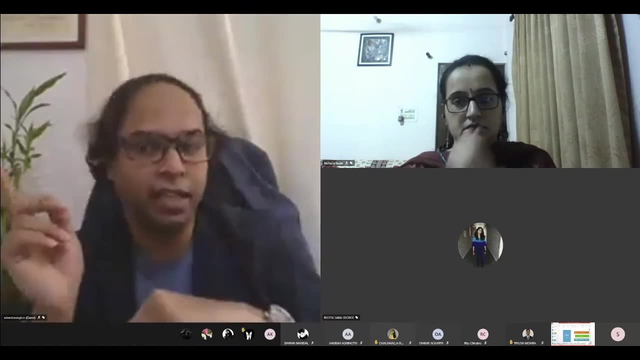 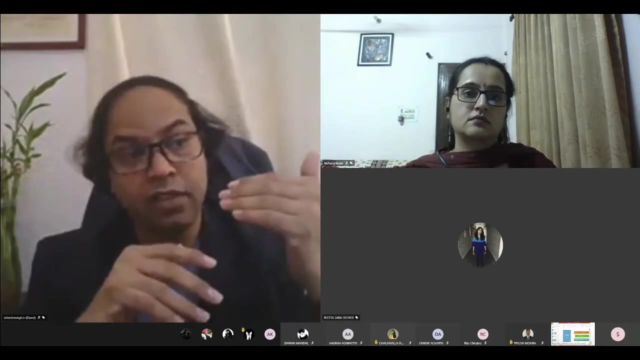 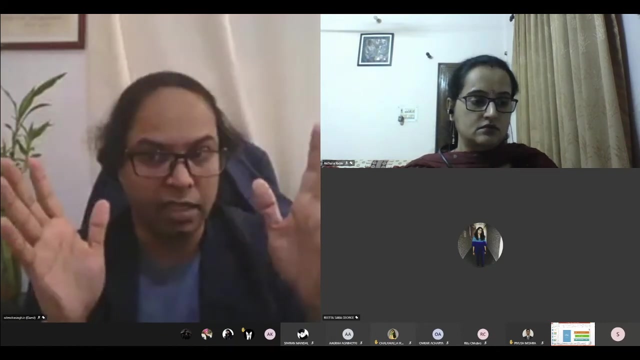 design, Then you give a detailed design report with all your data. Then they review your detailed data with their independent bodies, independent research, and they counter it. And if everything goes well, then nowadays they also review your severe accident management plan And once they are happy with that, then they ask you for the entire detailed report. 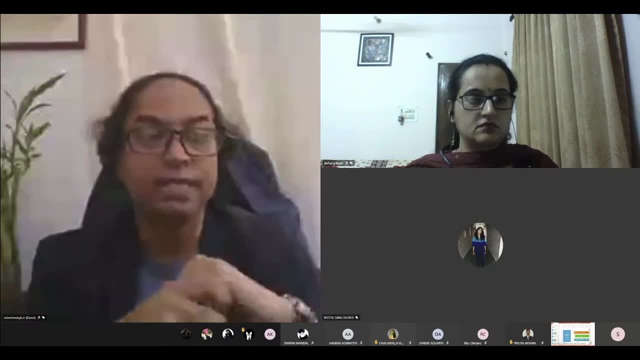 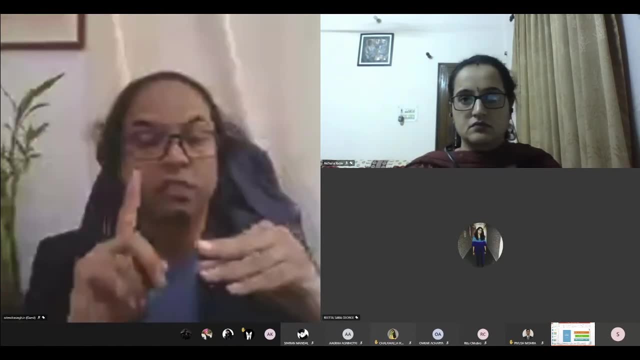 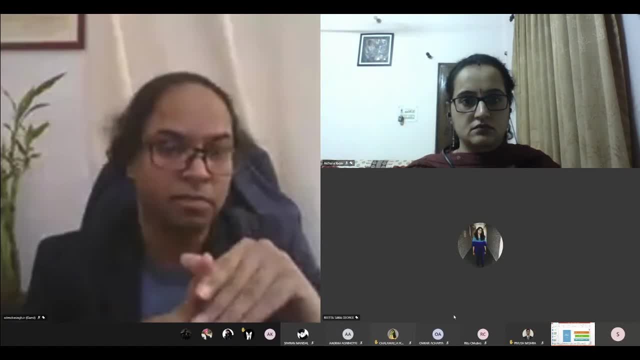 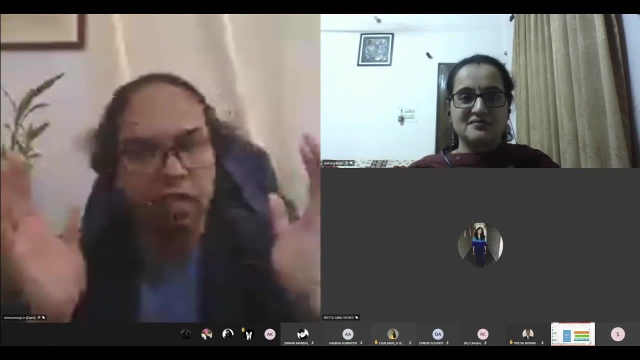 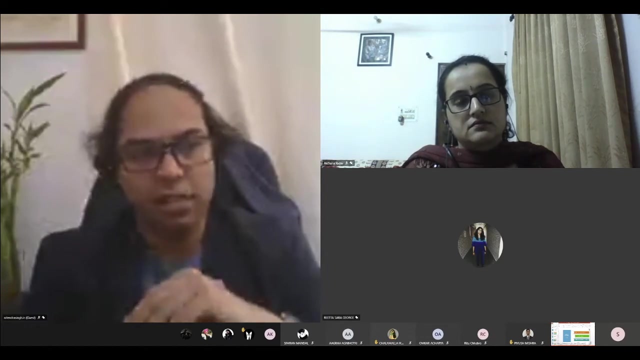 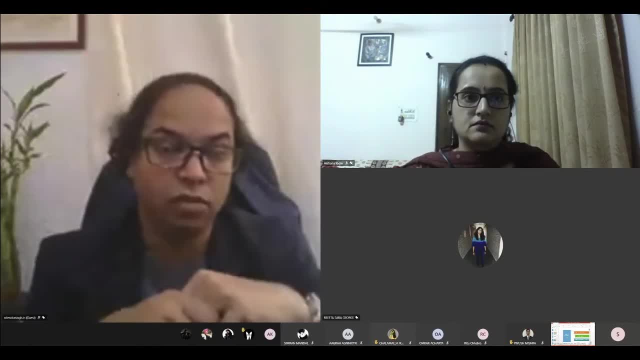 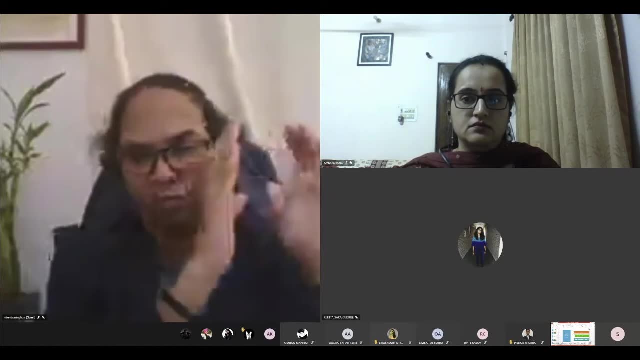 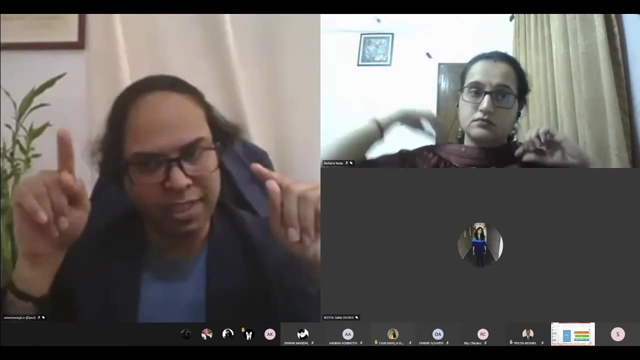 like um, a probabilistic safety analysis. you do so in us, they. they follow, like you know, event approach, where you define one particular event and you use your concept. okay, if this event happened, then you use this procedure and there is a defined criteria of for that event. you know, okay, this, this. 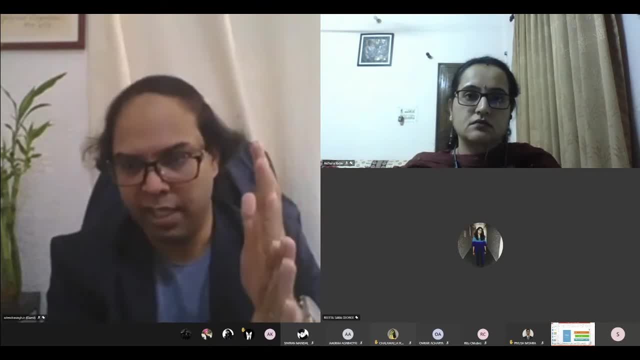 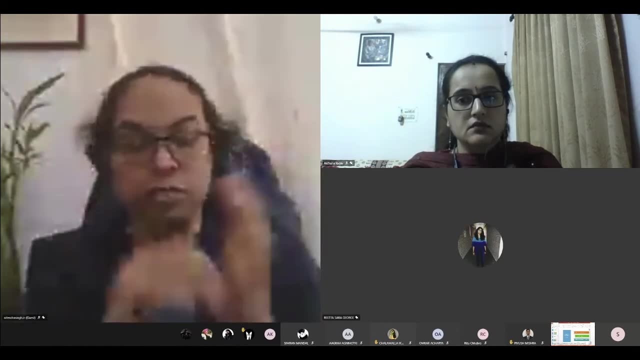 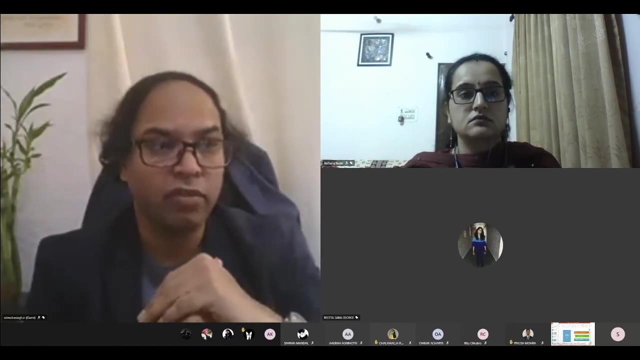 for example, this neutron flux, is this water level, is this temperature, is this? then you switch to a normal condition, to this event. okay, so this is like event approach, mostly united state follow. however, in case of france, for example, they don't follow this. they go with state approach, like what? 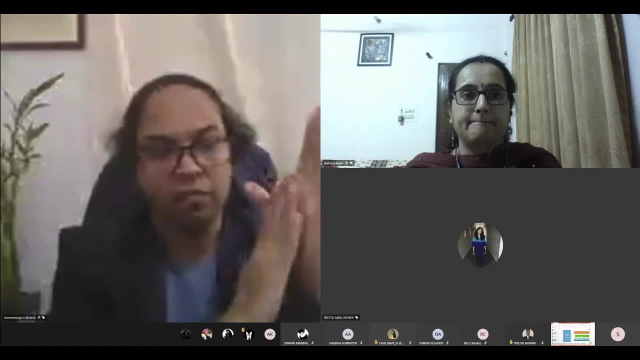 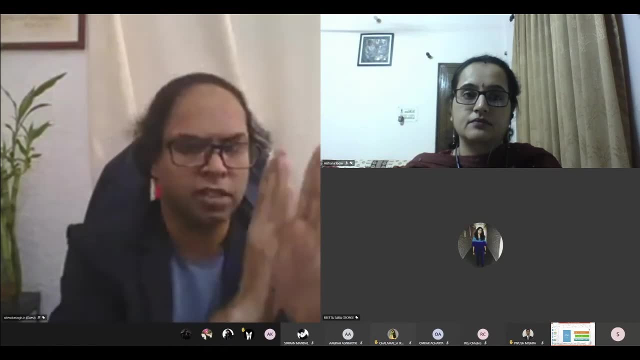 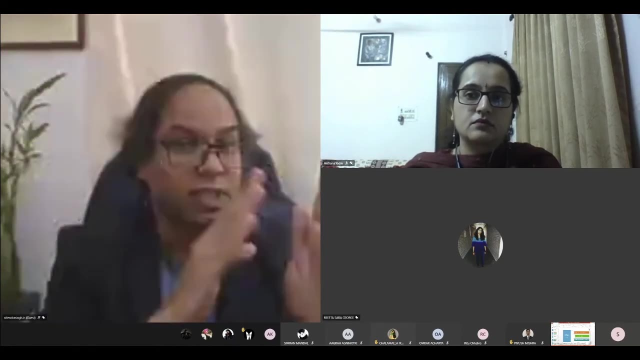 is the state of the plan. so in, in, in, in. for example, in the same scenario, they will not see what is the fixed temperature. okay, you have to switch. you monitor the plan. okay, you monitor what are the deviations? is the temperature is really increasing beyond certain limit and we cannot control it? or the reactivity or the neutral flux is really 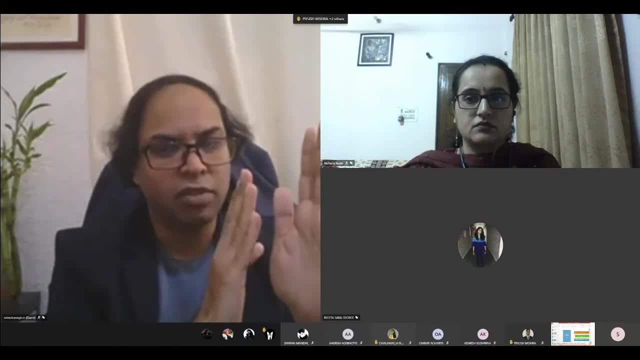 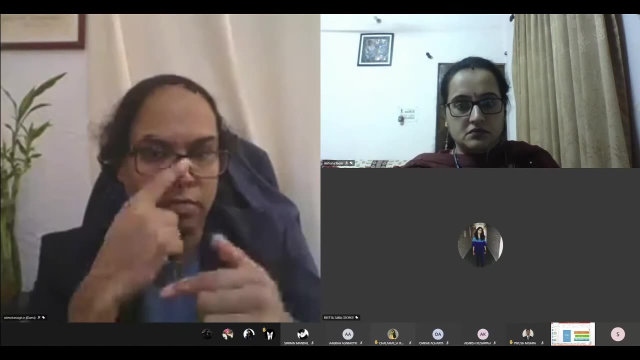 increasing on certain thing and you then evaluate: okay, it might go to this event, it might not go. once they are confident enough, okay, now it might go to this event, then they switch to the that procedure or the accidental procedure. so if this sort of a minute, things keep on varying. 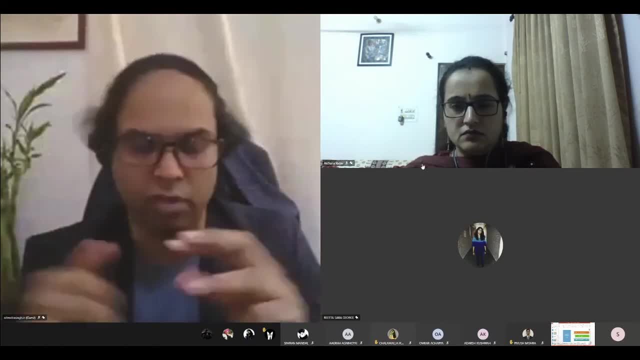 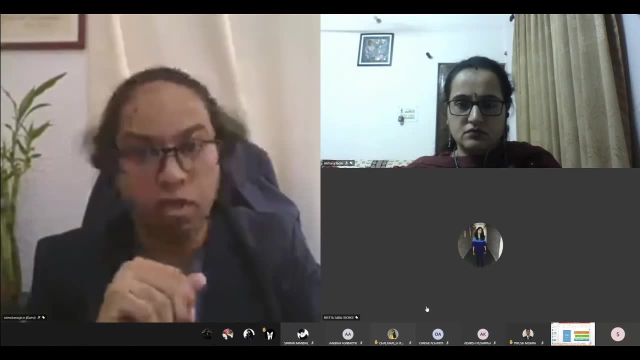 then you have to go with different regulatory board to different regulatory boards. okay, so likewise in india as well. we have our own regulatory bodies. we also follow our own norms, our own system, and in india you have more strict rules compared to other nuclear industries. this i should 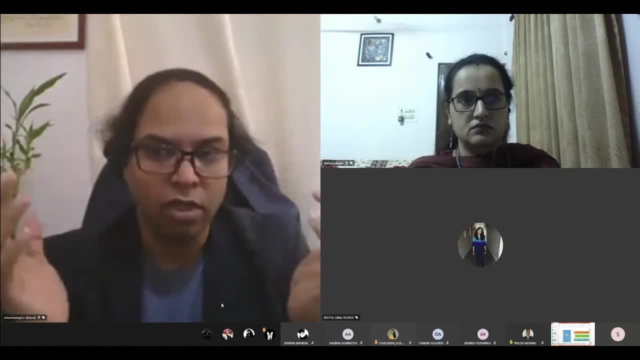 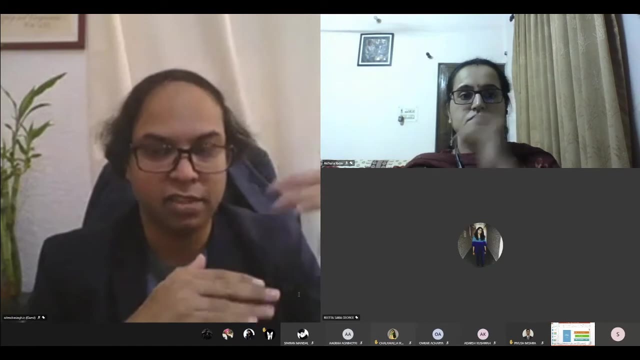 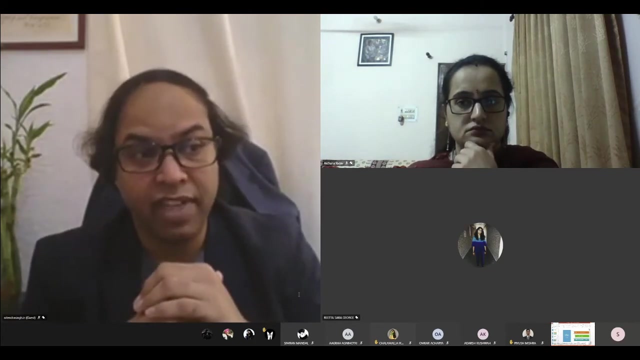 mention. so somehow every country has their own way of doing and analyzing this sort of thing. now i can ask you a question, which is how the licensing process has varied. when you talk about the second generation plants, turn generation in the advanced reactor of four generation, four plus. so of course, system varied because, for example, uh, earlier you were not having passive 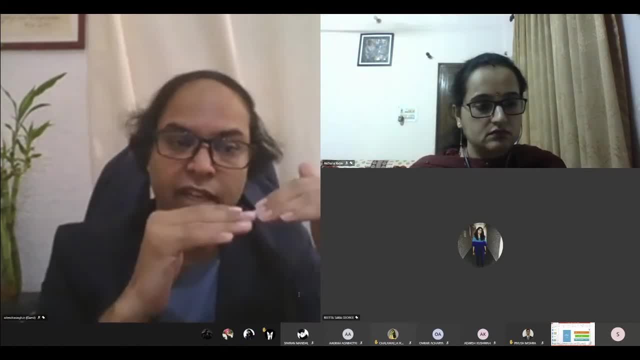 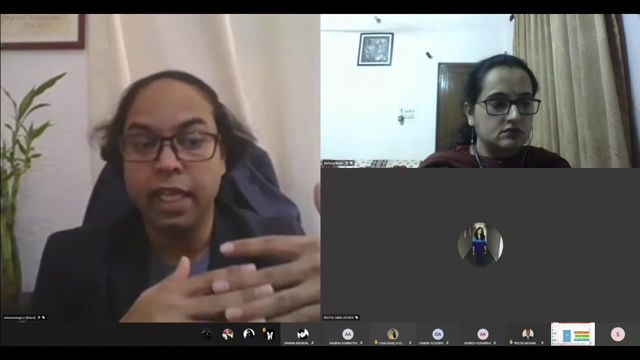 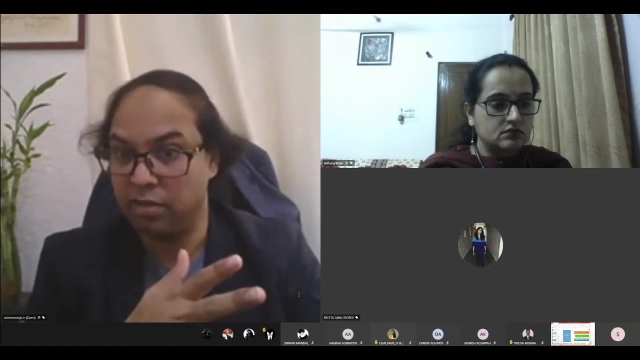 system, for example. so now if you want to license where your design include a passive system, then regulator need to understand that system first, need to test that system first so they may ask you with the data. ok, give me your data, experimental validation, experimental data, which I will also get verified with my own. 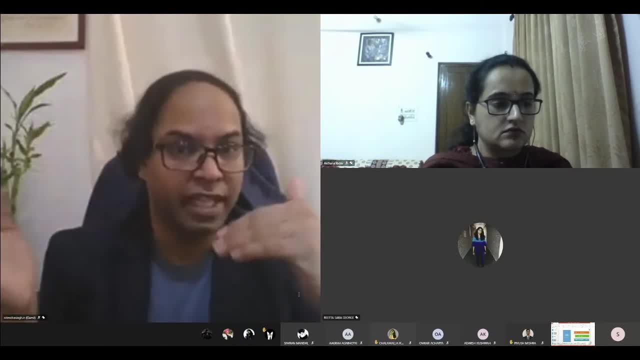 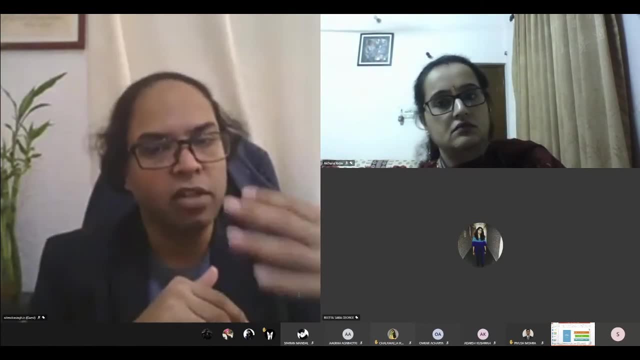 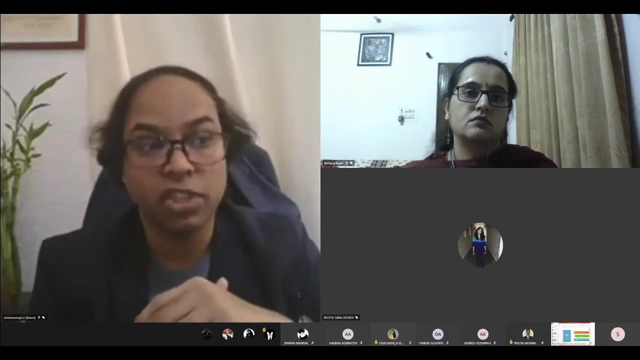 experimental setup or the codes or whatever resources I have, then, once I am convinced, I will allow you to do so. So with all these new things coming, the regulator also have to upgrade itself. So this is one change which few nations have done and few nations are. 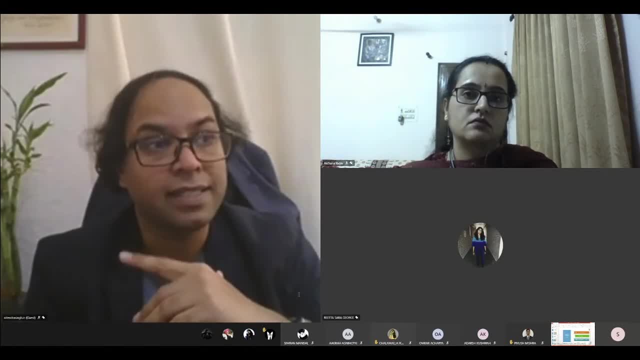 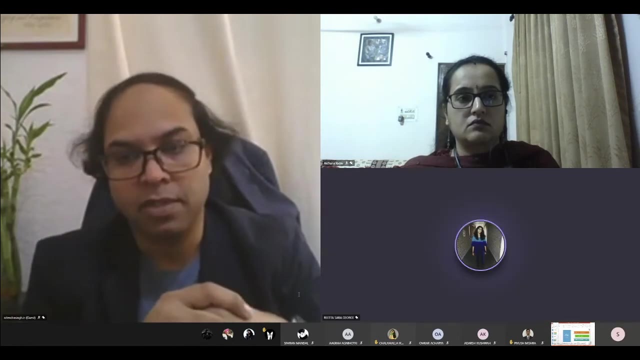 still in the process. And secondly, like as I mentioned, one of the key component is core catcher. not all nations are coming with the concept of core catcher first. Secondly, the core catcher is itself is a complex concept, so few people are coming with a different. 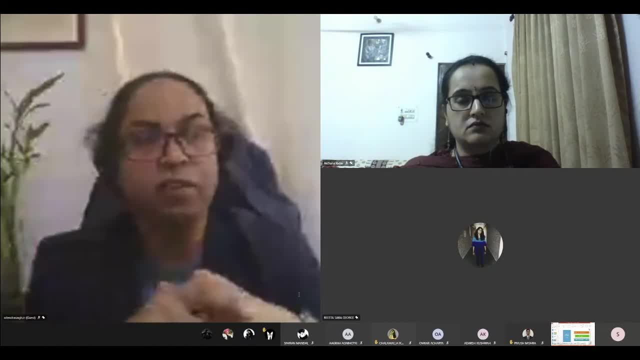 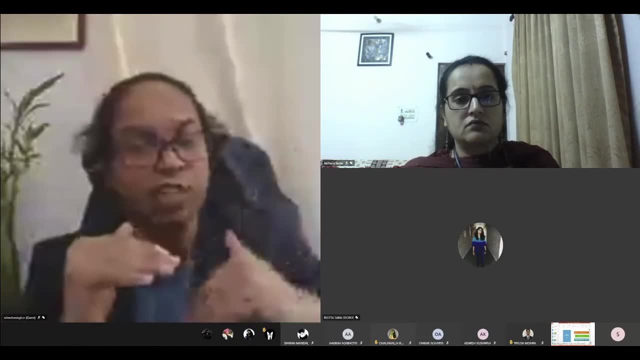 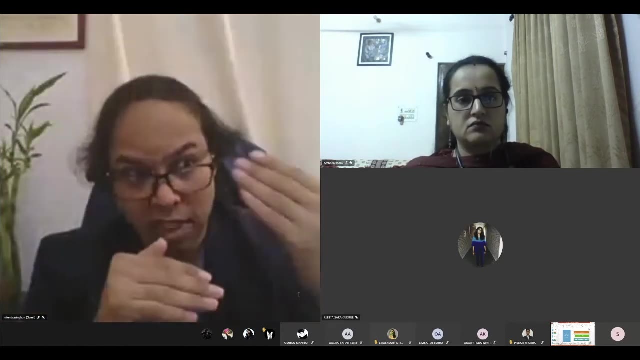 concept. few people are coming with a different concept. So then regulatory has to understand what is good, what is bad, or what is good up to what extent and what is bad after which extent. So regulator also have to improve themselves very much. Third point: some you know earlier they were the thing like people were constructing reactors. 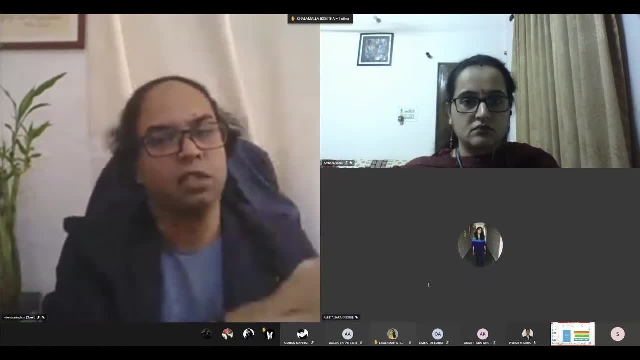 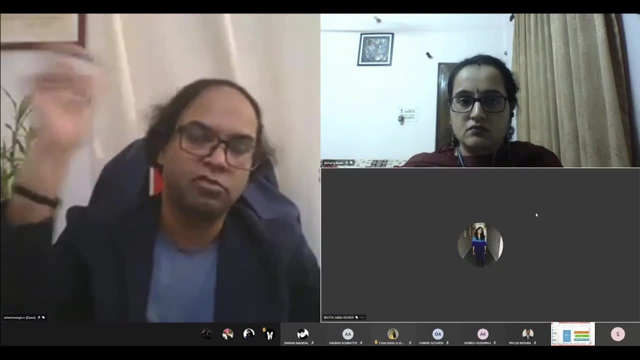 in their own country. Now one country is constructing in another, For example in China. most of the people are constructing In Egypt. people are constructing in their own country. So people from China or Japan, they are constructing. or Korea is constructing, for example, In India. 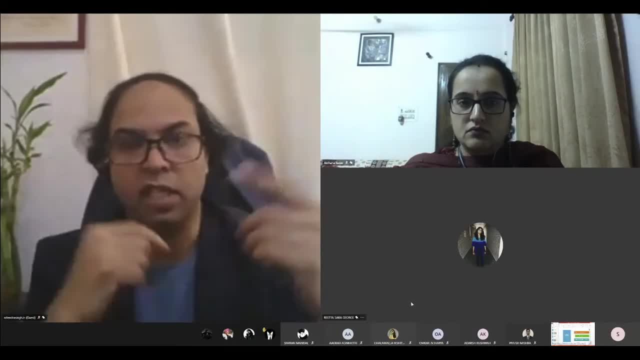 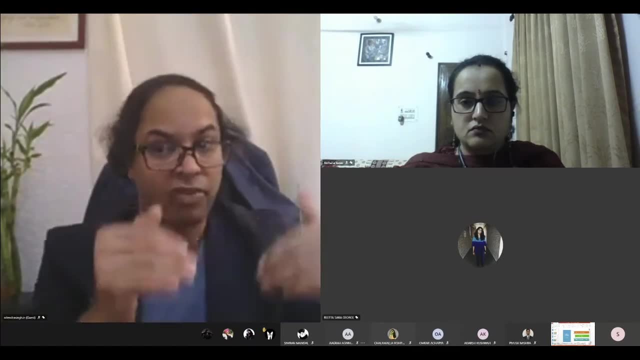 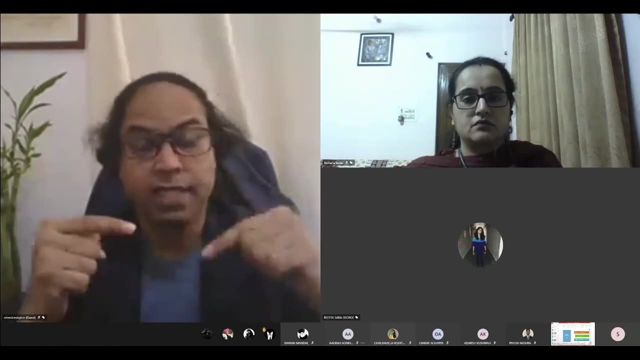 you have Russians who are constructing and France is also constructing. So when you design a reactor, you design it in with your own regulatory guidelines, But when you are putting it into another country, you have to follow their regulatory guidelines as well. So this also adds a pressure. 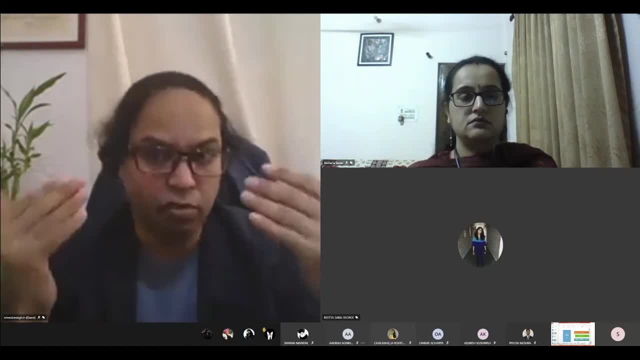 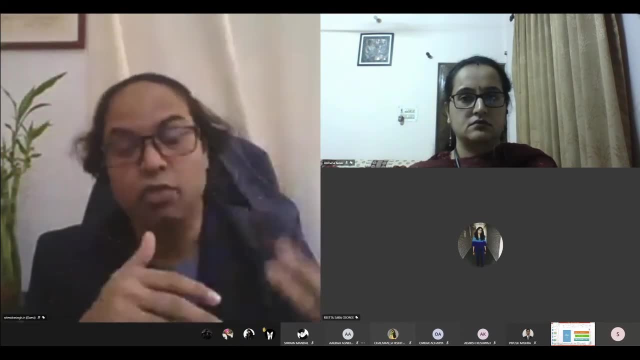 on the regulator to upgrade themselves, to understand what is good and what is bad. So you have to understand all you know to be in sync with all global regulatory bodies. So this is, this is one more change which you have seen, and the most recent, I would say. 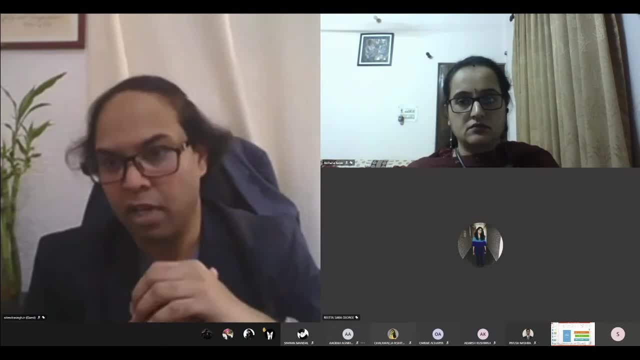 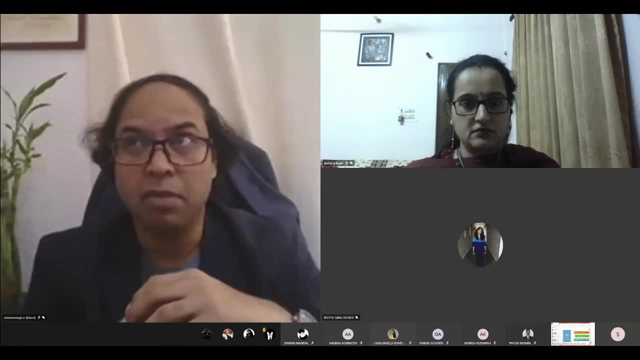 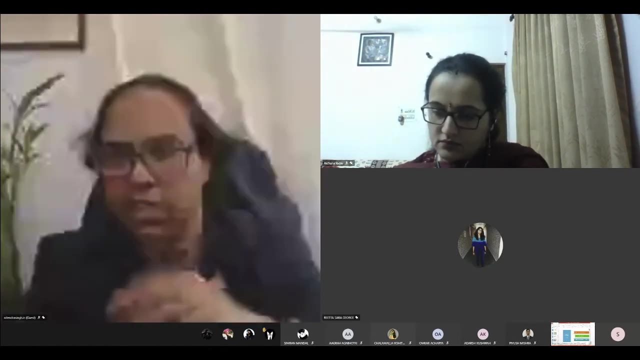 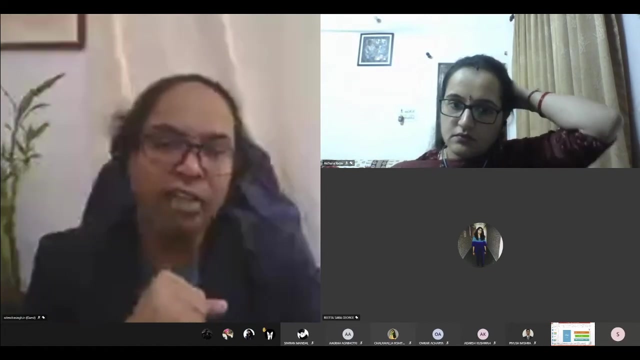 is the SMRs, the small modular reactors, which have come up. So there have been. you know, for the moment there are like almost, if I remember correctly, 80 something plus designs across the globe on SMRs, small modular reactors, in different countries. So, but so far only USNRC, which is the US regulatory board they only have given the approval to 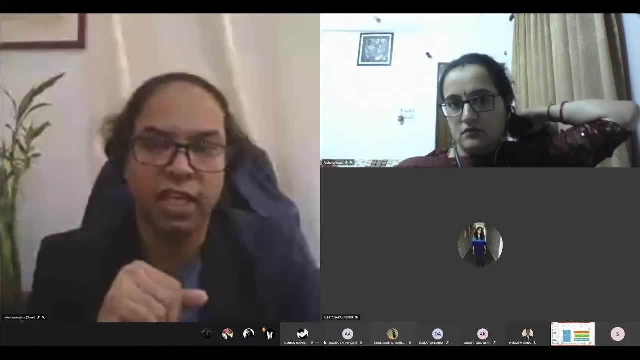 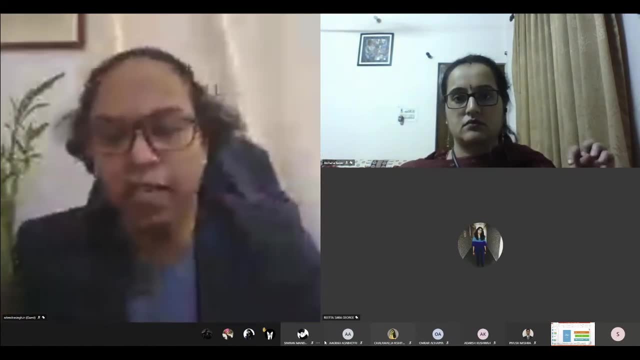 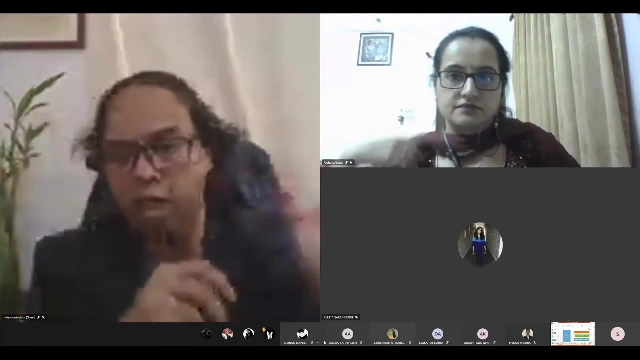 New Scale, SMR. New Scale is the company which made SMR, a small modular reactor in US. So now, and for example in India, we still don't have any, any regulation about SMRs. So somehow, and not many country has, only only USNRC has so far. Other other regulatory boards are: 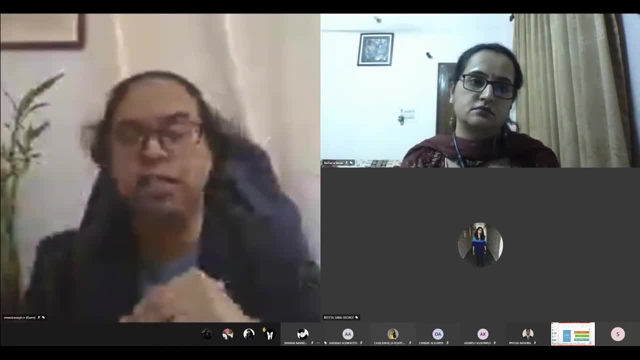 established in India, ARRIVALA RAMANEEVARAMANAN. AND So you are. you are now a successor of the Kandu organization company. So why do you want to do that, please tell me? And you have been, are still working on it. so that's how you, because of the change in technology, 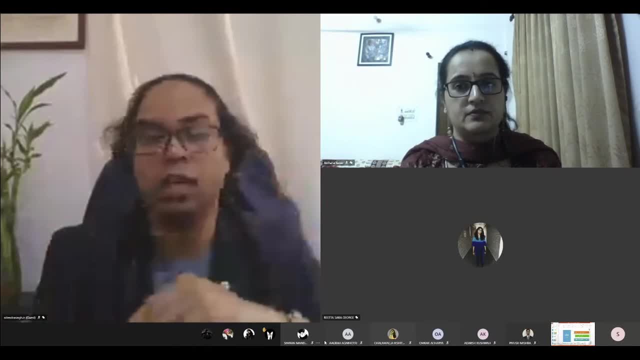 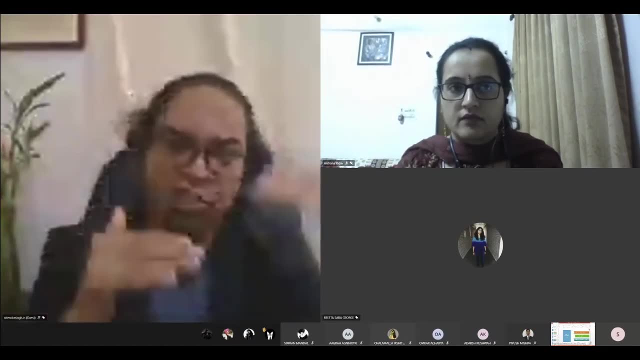 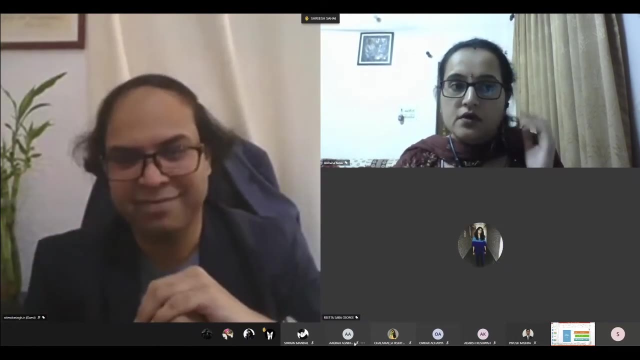 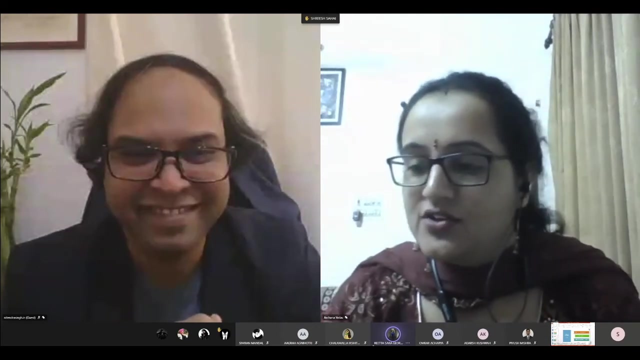 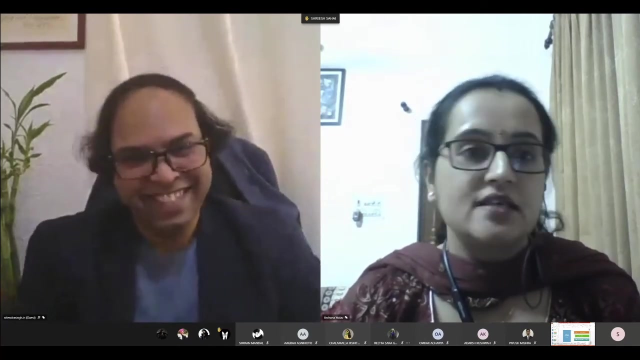 because of the improvement in the technology. you basically upgrade or improve your system yourself as well as a regulator. so that's the change. you will see both your passions you mentioned in one of the slides, that is, elimination of emergency planning and, as I understand, licensing requires an 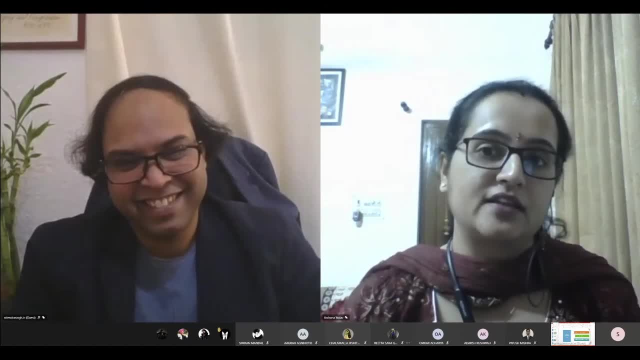 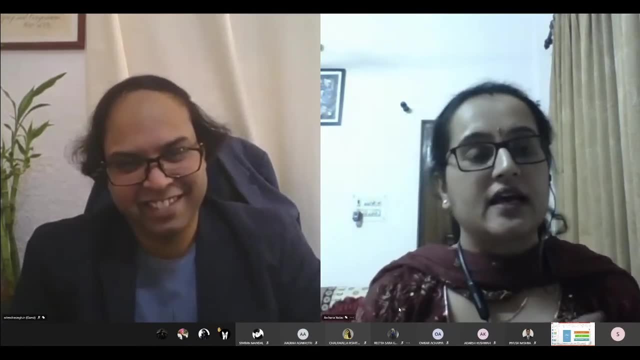 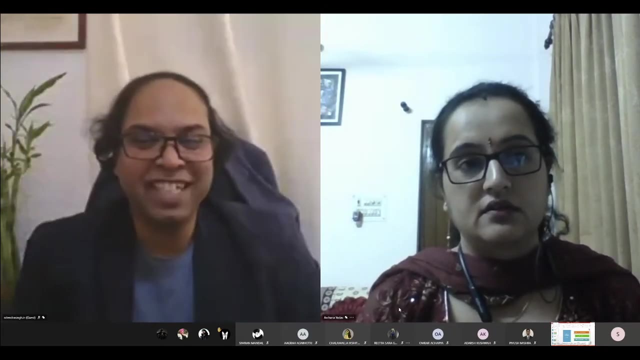 important consideration of even the emergency planning that's also covered. so if this part is somehow taken care by the design and the inherent safety features, I think the licensing will become much more easier. yeah, so that's where the clash between a designer and the regulator comes. so for 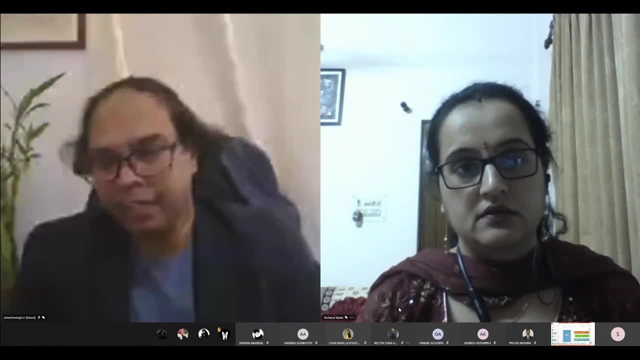 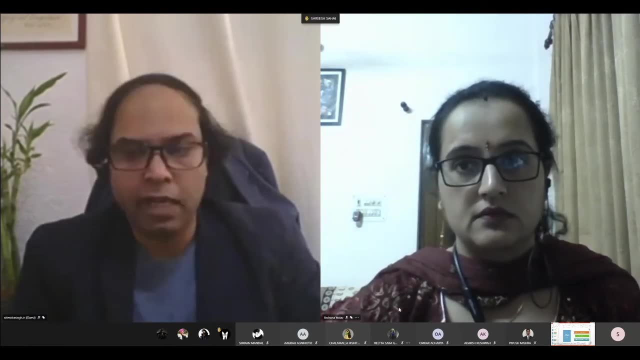 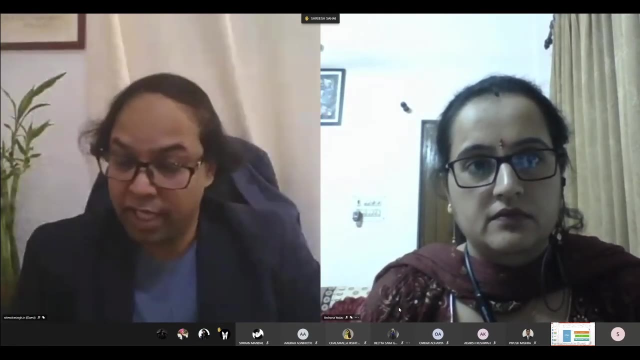 example. I go back to 2010, for example, when they designed EPR. so EPR was one of the most advanced design at that time and they were claiming it. like you know, this is a reactor which can be constructed in the middle of the city without any 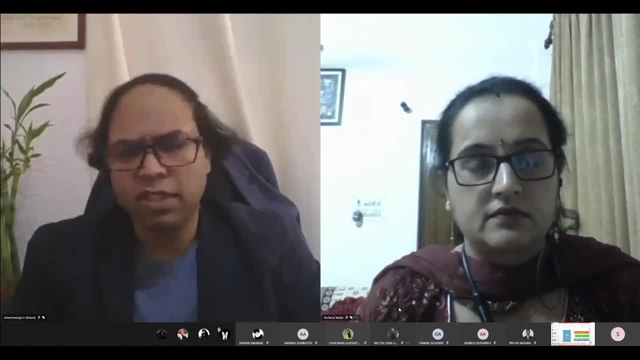 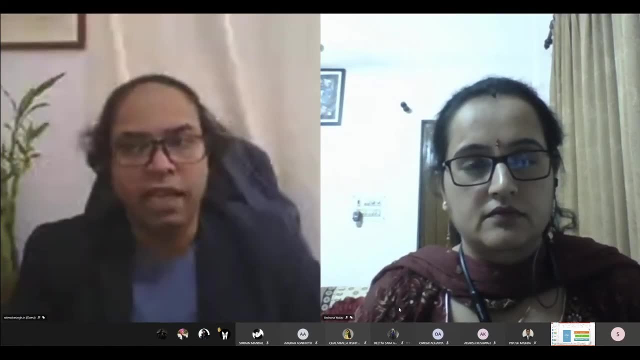 exclusion zone without any emergency planning and of course they included a lot of great safety systems. I would say at that time they were adding a core catcher. at that time they were having so many passive system and stuff, but the regulators were not ready at that time they were. there were a lot of debate going on. designers wanted to do so not. 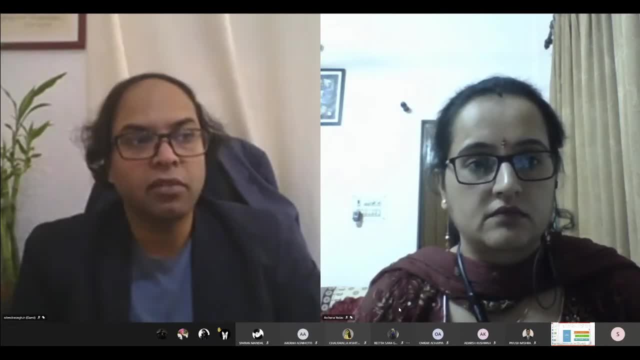 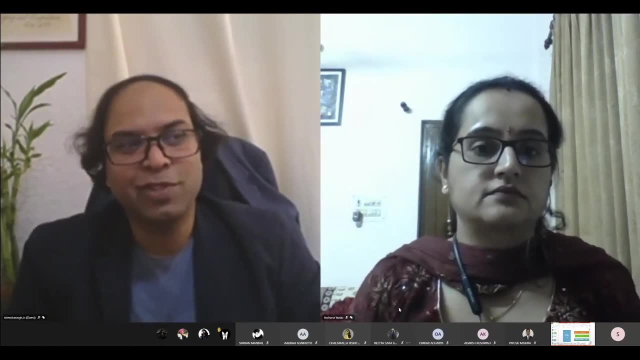 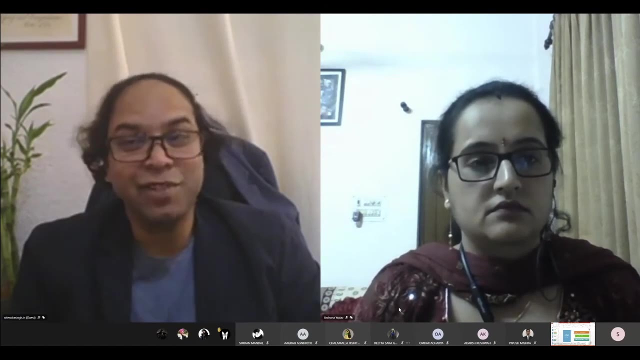 because they wanted to compromise with the safety, but they wanted to do it for, you know, gaining the confidence, like you know, we can make such a safe reactor. unfortunately, in 2011, March- March 11, of course, to be precise- Fukushima happened, and so those regulators who were, like you know, trying to think of: okay, let's. 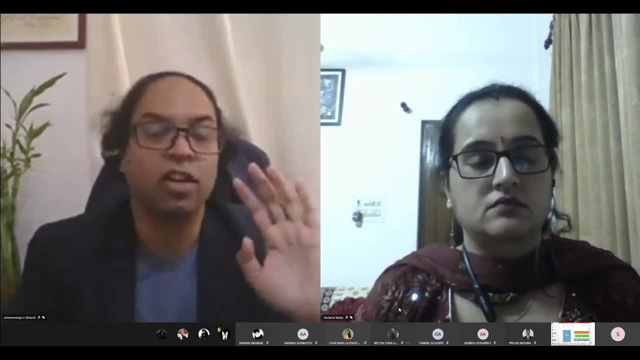 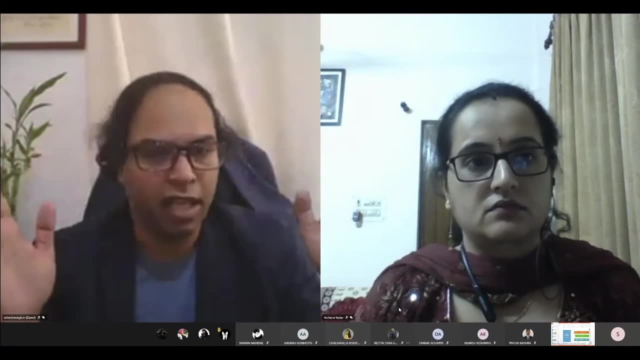 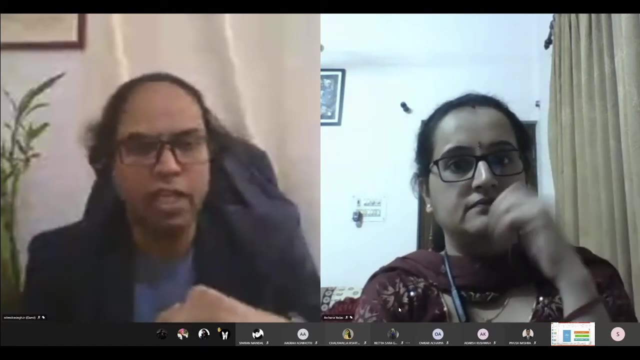 give it a try. they again went back. no, we cannot. we cannot think of. even if your reactor is that safe, it's okay. there's no harm in having an exclusion zone or the emergency preparedness, which is a wise thing, I would say, as you know, in. 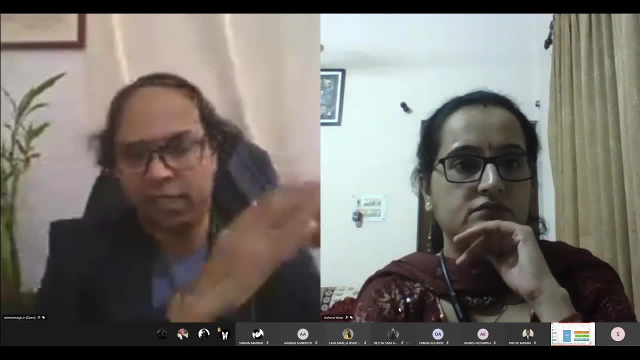 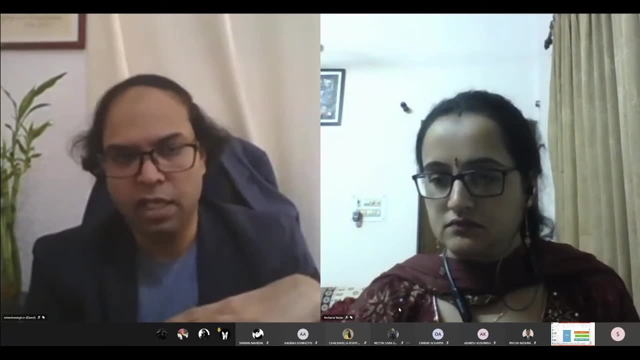 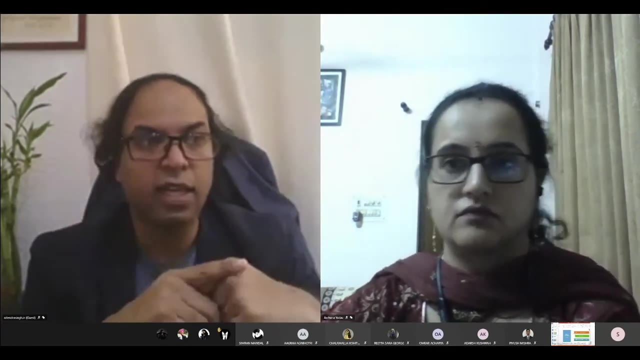 nuclear industry we always follow to have a redundant systems on and the diverse system. so having one more redundancy there's no harm. so, as a regulator, if I am thinking when I am thinking in a correct manner, this is: this is one. secondly, when designer wanted to say that we do not have the right infrastructure, 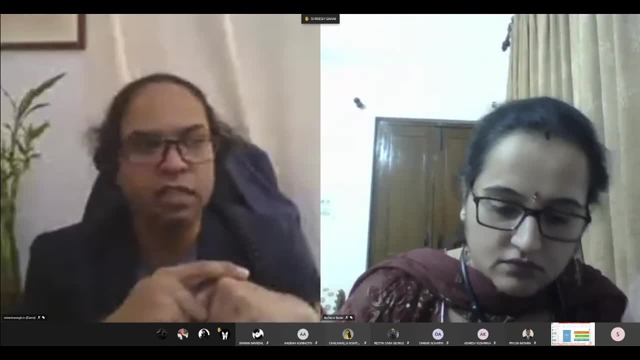 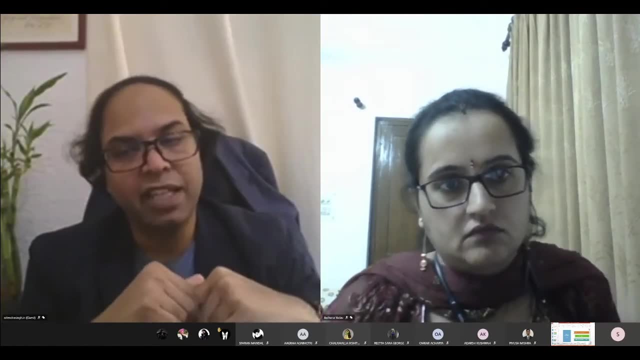 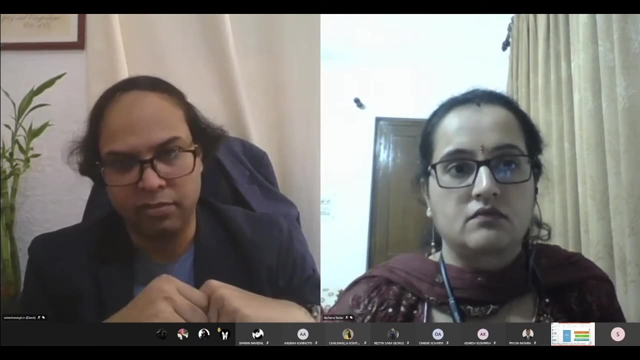 want to have any emergency planning. they were okay with it, but they were missing one aspect which i would like to highlight here. epr, when they were proposing epr, is, like you know, 1300 megawatt electric uh capacity reactor, which means, like uh, almost 4000 megawatt thermal energy. you. 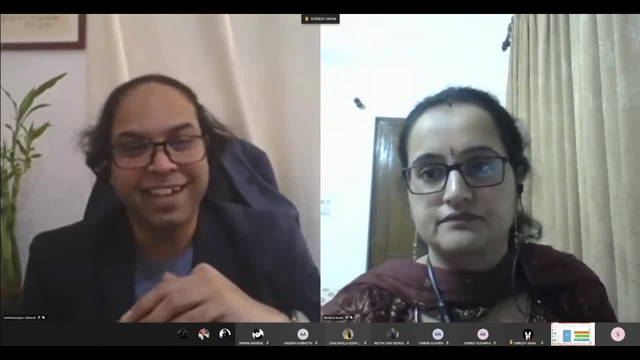 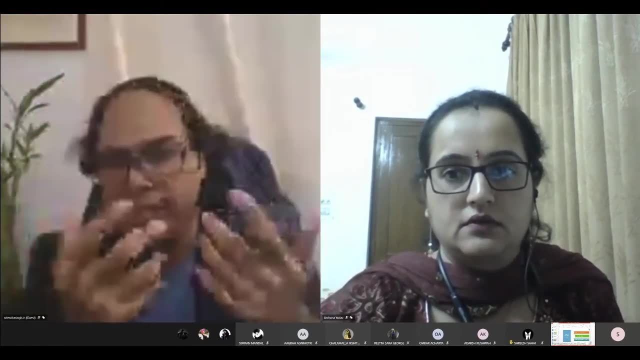 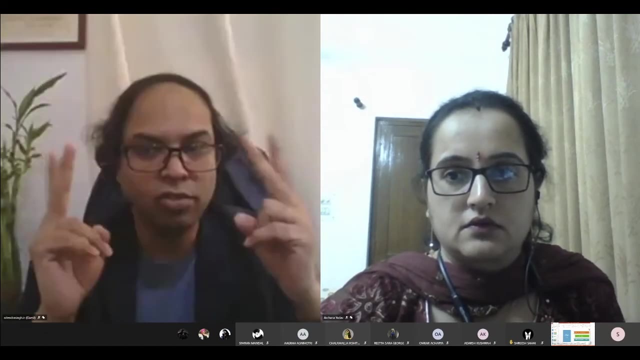 are putting you want to put in the middle of the city. so, in any case, if any kind of deviation will take place, it it's an added risk, then why to add it? however? uh, if you see the concept of smrs now, now, if you compare these two, because these two are the main designs, or or generation four plus, 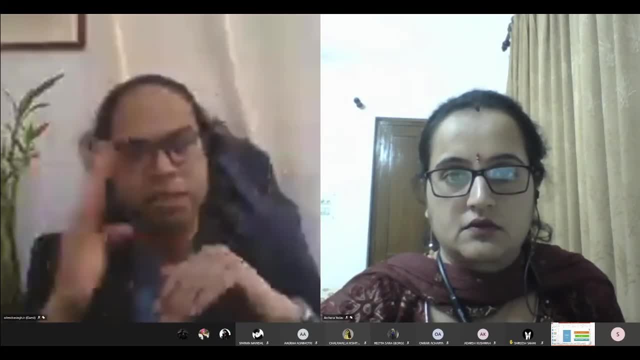 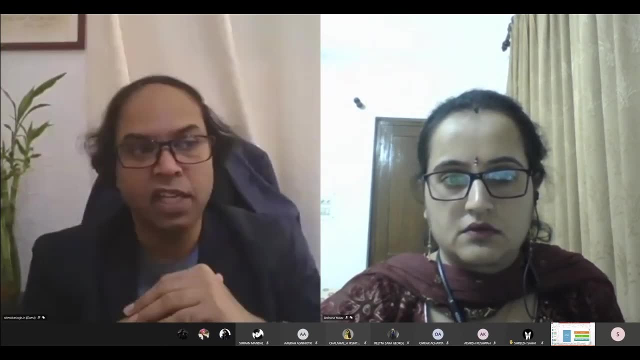 if you compared with the, with the smrs. so generation four plus and smrs both claim that we can remove the emergency planning in a way. so in smrs, if you say the smrs, uh, most of the designs are of, you know, 80 megawatt. 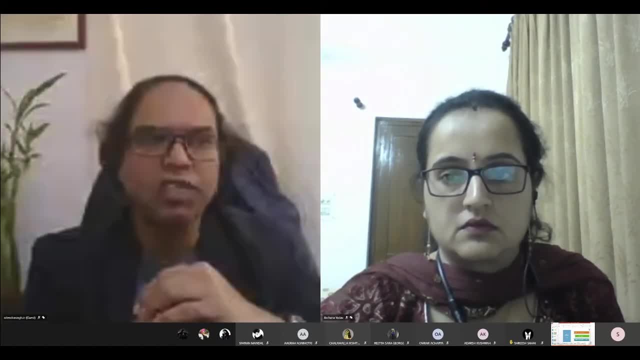 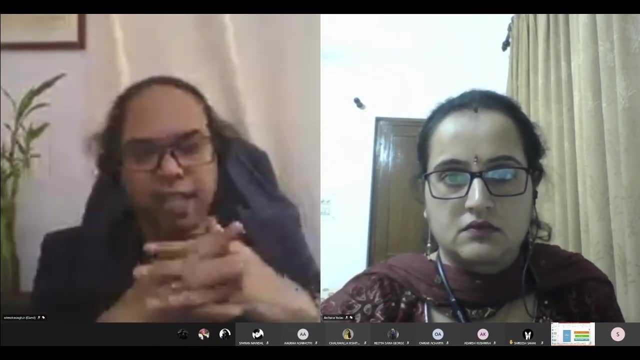 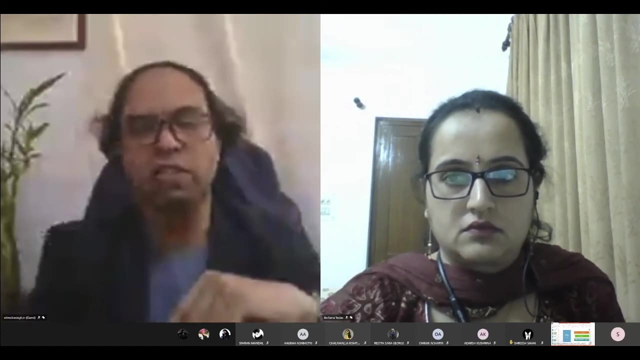 100 megawatt of this, this, this power level, which is okay, which is okay. and also, they are integrated modules, like you know, the the chances of leakage are minimal because you don't have anything coming out the out of the pressure vessel. first of all, and in most of the scenarios, these 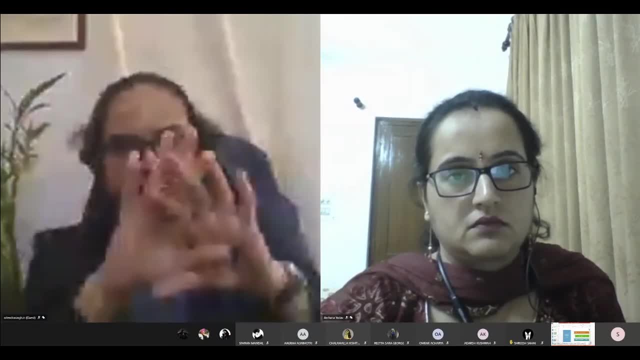 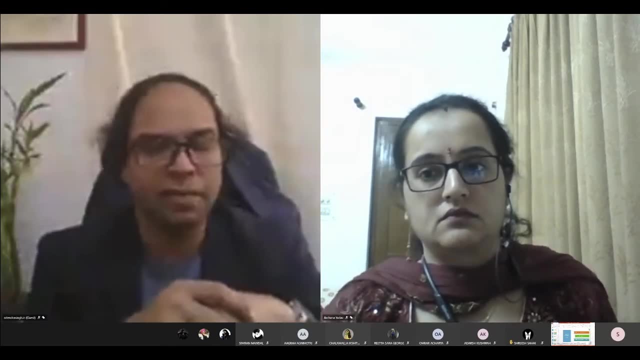 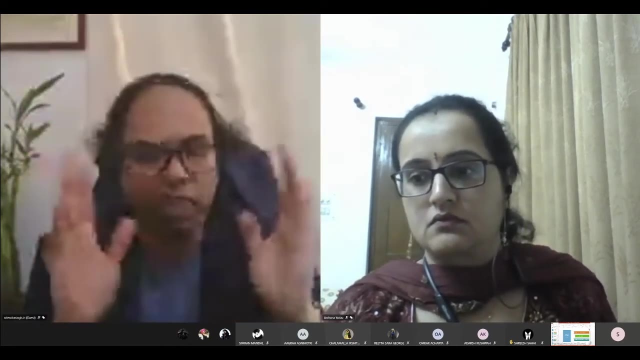 entire reactor within the pressure vessel is already dipped inside a water, so the chances of a core melt and stuff they. they are eliminating that in a way. so of course they are also coming up with this kind of clean. so it's okay in terms of a designer's. 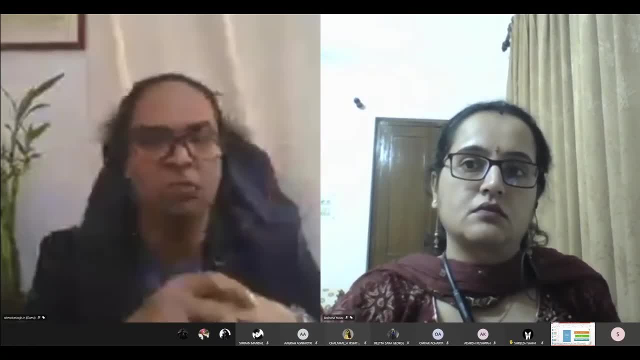 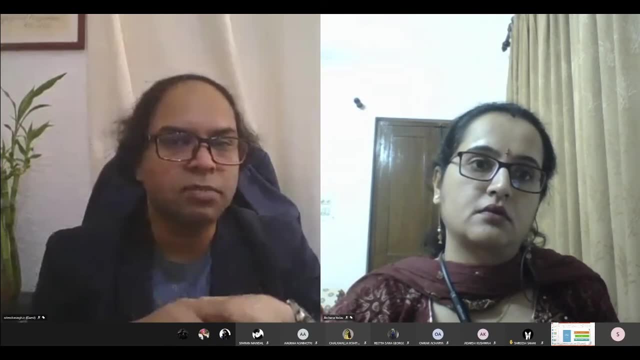 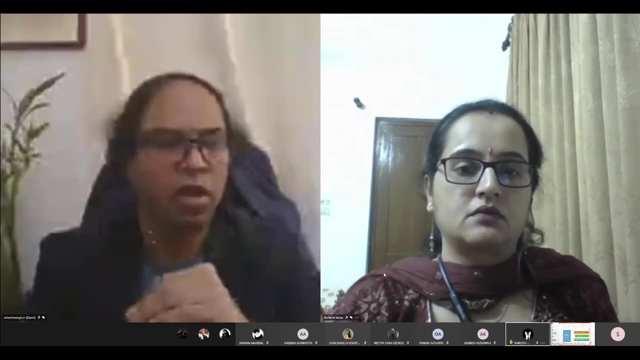 perspective in terms of engineered safety system, but in terms of regulation, uh, regulator is someone who is responsible for the public. you know they have to make sure that whatever is going to the public domain, it should be perfect. so if they are asking to have one more added level of emergency to 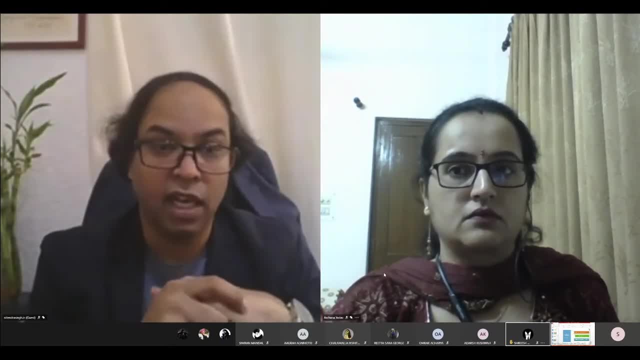 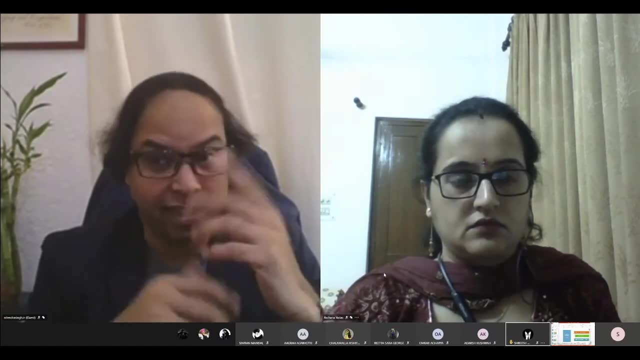 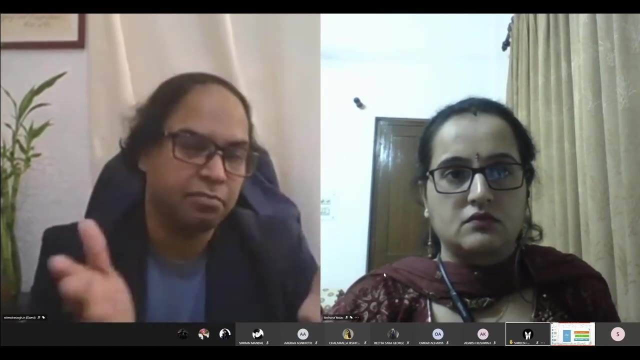 planning or exclusion zone, then there is no harm. I don't think. of course there is a added price to it for the, for the operator or for the designer or whosoever is constructing that. but in any case, our first priority is the public safety, so there is no harm in editing. 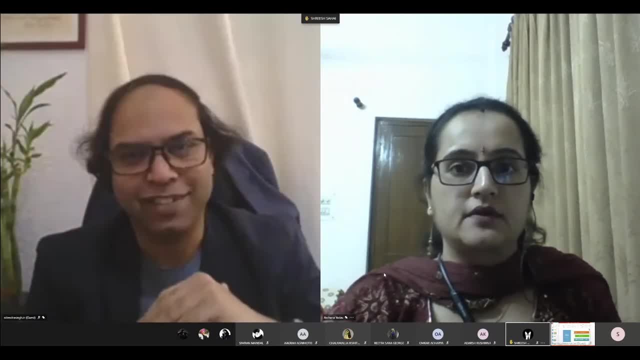 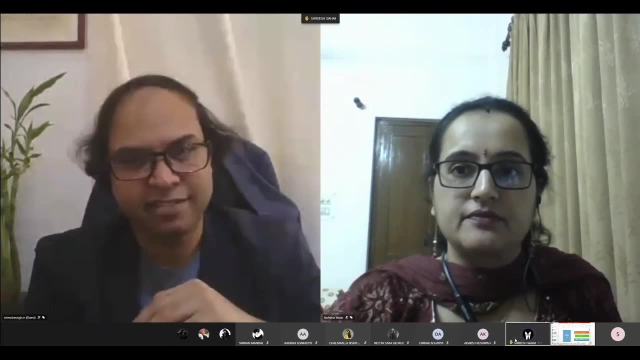 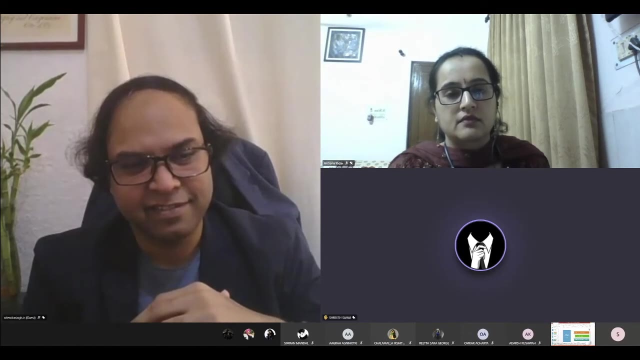 yes, that's what I feel, okay, so next I think Shreesh would like to ask a question. Shreesh, please unmute yourself. yes, thank you, sir, for that presentation. in the beginning you had you had started with the concept about safety and you had also mentioned the IAEA definition. 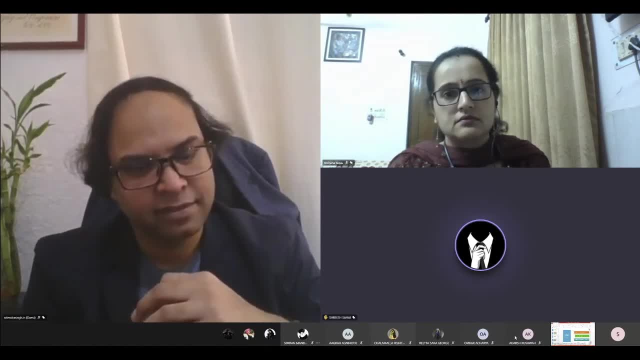 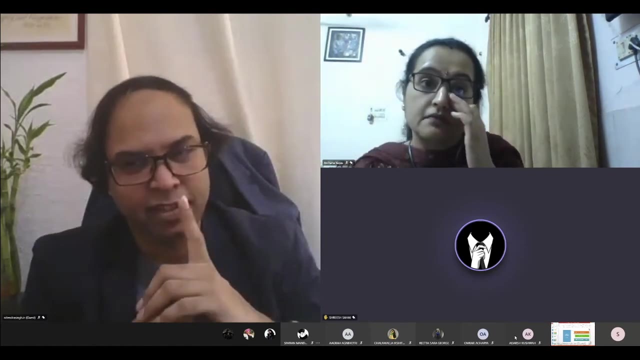 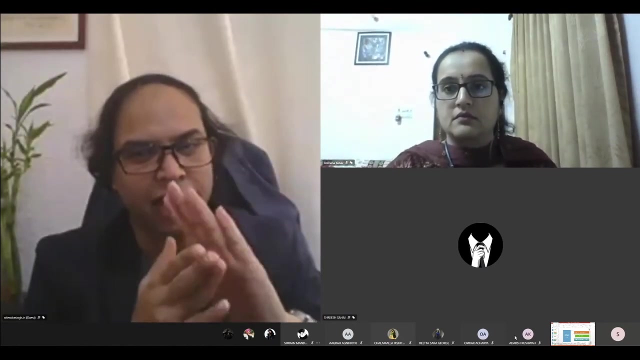 and all that. so my question is that, assuming that TMI and Chernobyl had not happened, what would have been the state of the security measures that are taken by nuclear power plants in today's context? so you have I, if I want to understood correctly, you have mentioned security. you want to understand? 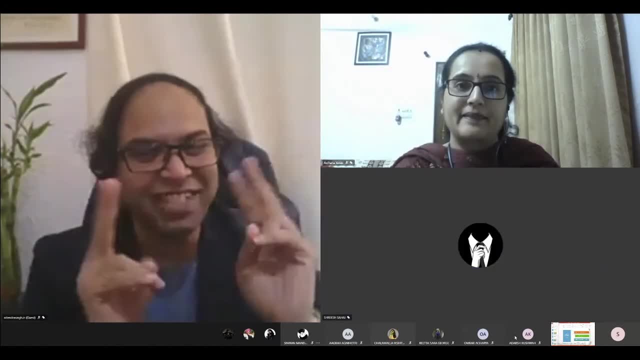 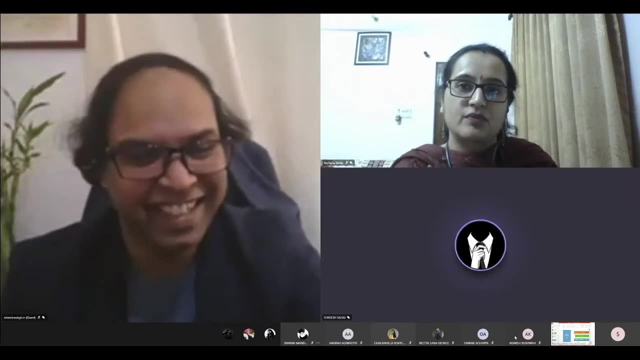 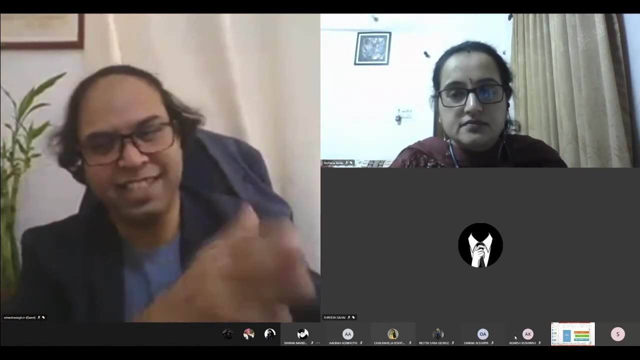 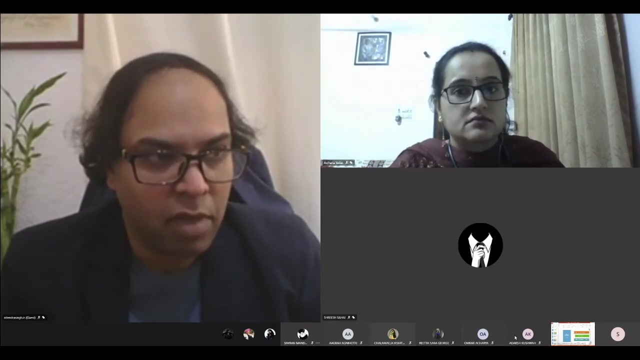 about security or safety, because they are two different things which work hand in hand. I may comment on both, so it would be better if you could mention about both this. yeah, yeah, yeah, yeah. so let's discuss the safety first and then I'll come to security. so yeah, let me tell you in this manner: if TMI or Chernobyl would not have happened, so you mean to? 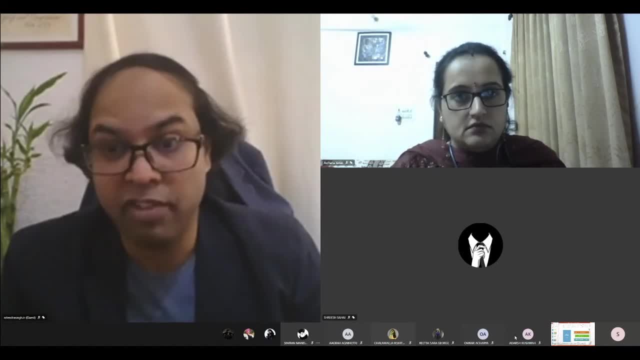 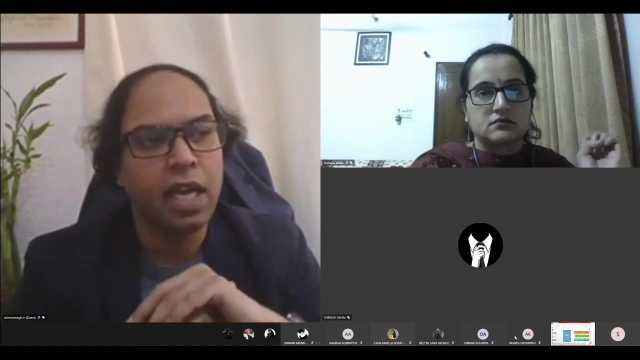 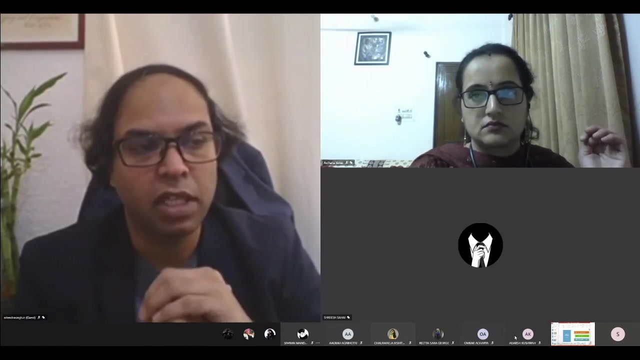 say, if they would have not have happened, we might not work or we might not improve our safety level. what we are having now, if I understood correctly, that is your concern. yes, let's tell you one thing: before TMI And before Chernobyl, Chernobyl was in April 1986 and TMI was in, if I remember correctly, May 1979. 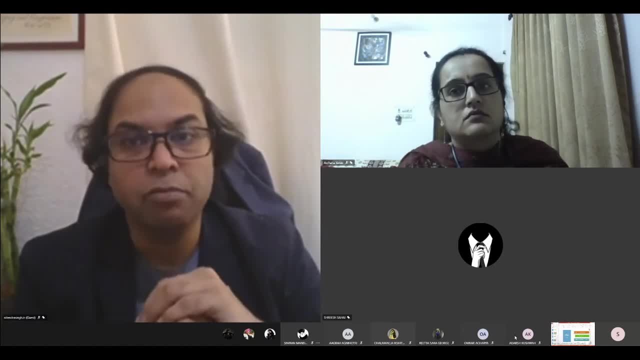 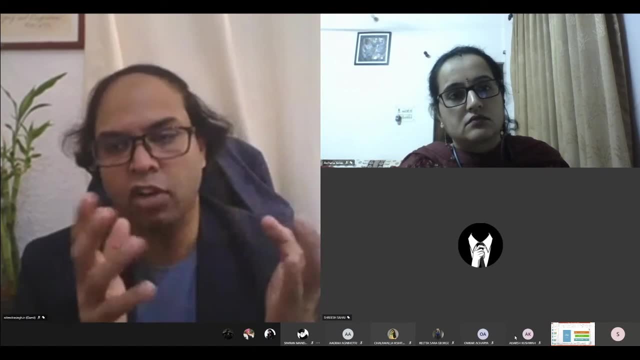 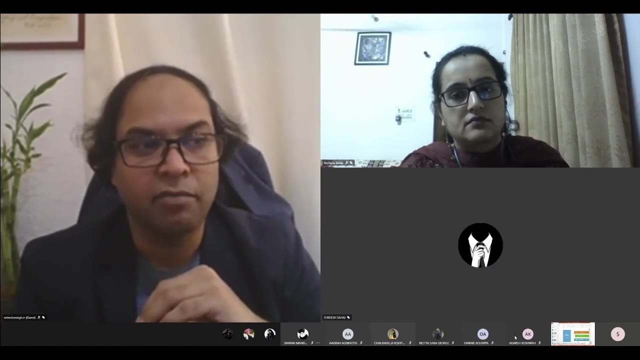 But in 1974, there was a report which was, you know, generated by a team which was headed by Rasmussen. We call it as the Rasmussen report or WASH 1400 report. It's a very famous document, very relevant for all the nuclear safety aspect. 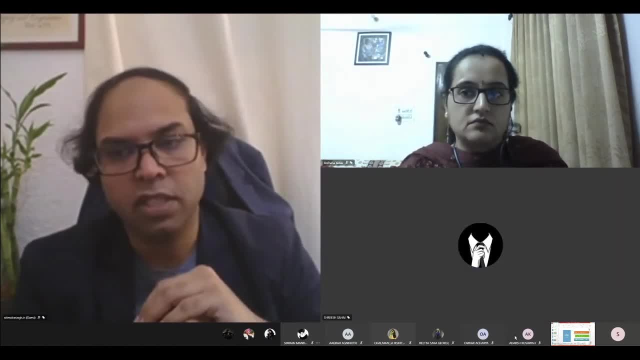 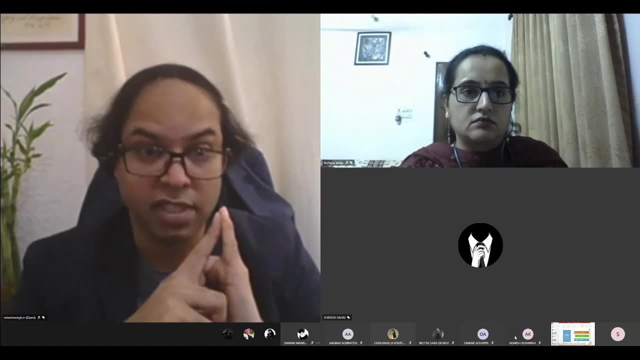 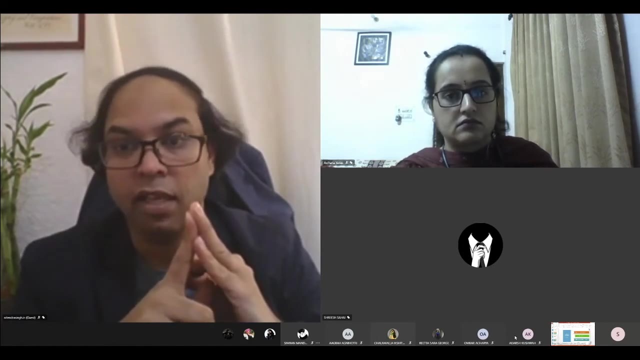 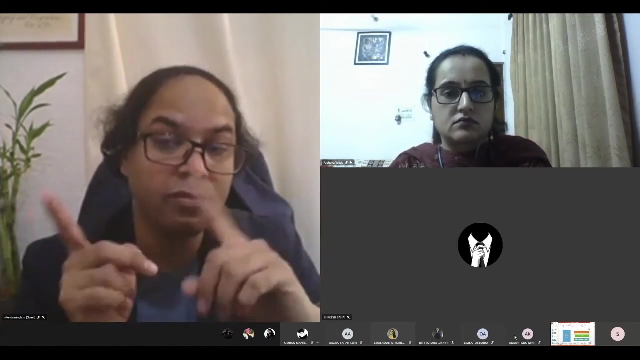 So that report, you know, for the first time, mentioned critical things about, like you know, they mentioned the possibility of core meltdown for the first time. They mentioned the possibility of- you know this- common cause failures And they mentioned the possibility of integrated failures, which actually took place in Fukushima, for example. 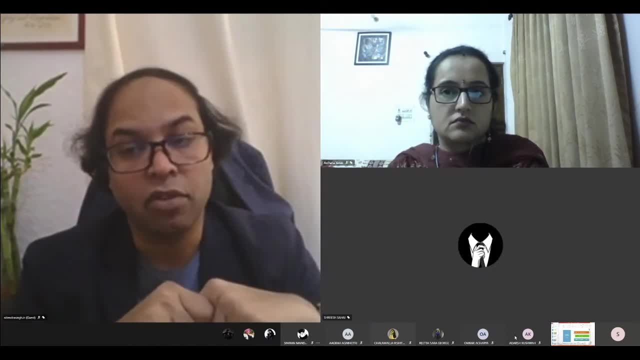 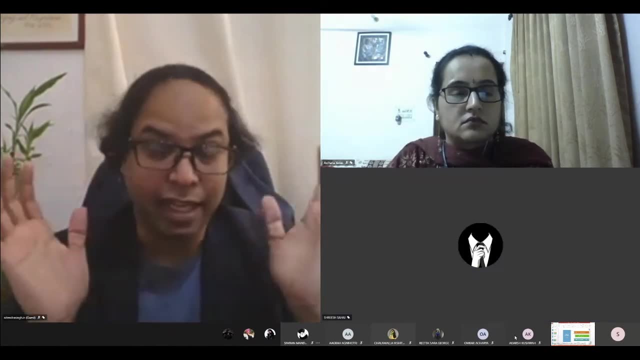 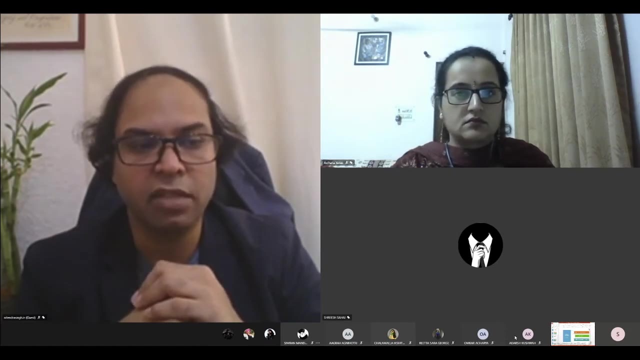 So I'm talking about in 1974.. So when they come up with the idea, designers at that time they said: okay, it's a great report, It gives a great possibility to understand and it's nice. Everyone appreciated. but designers were questioning. 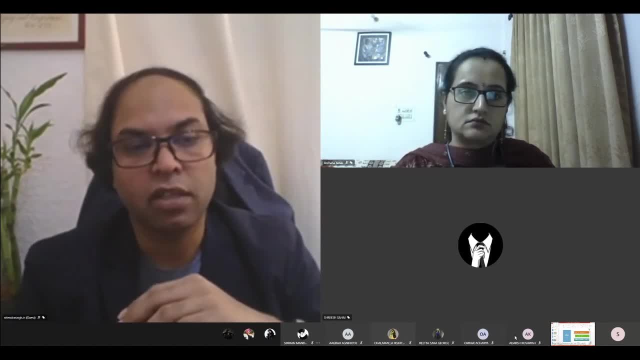 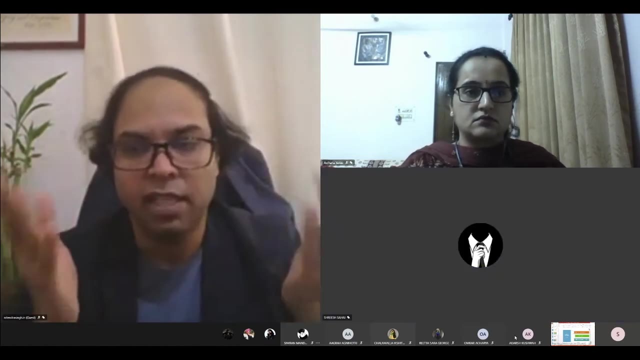 Because, in a way, it was questioned. it was like you were questioning the capability of your engineered safety system and, indirectly, you were questioning the designers, like what you have made. But it was not like this. So there was this debate started. you know, like we made safe the report, want more safe, this thing started. 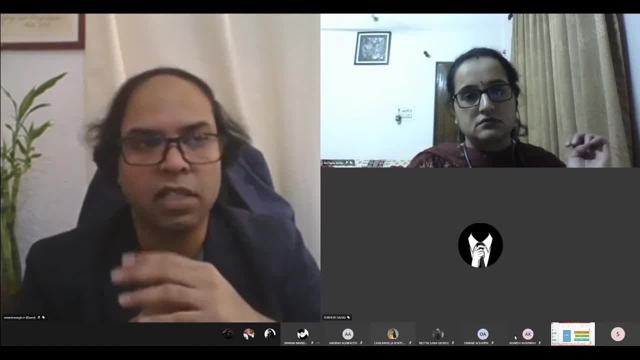 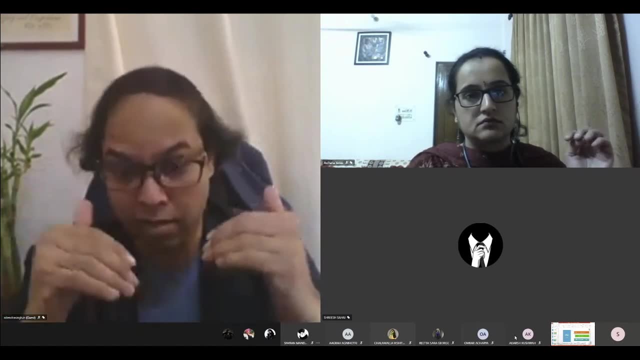 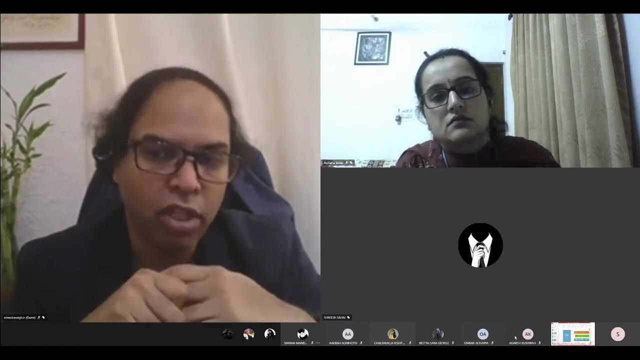 If I understand correctly, okay, at that time- We are talking about 50 years back- might have took a while to improve to this level. If I want to add one more point of it, as I'm saying, like after Fukushima, everyone wanted to have a passive systems. 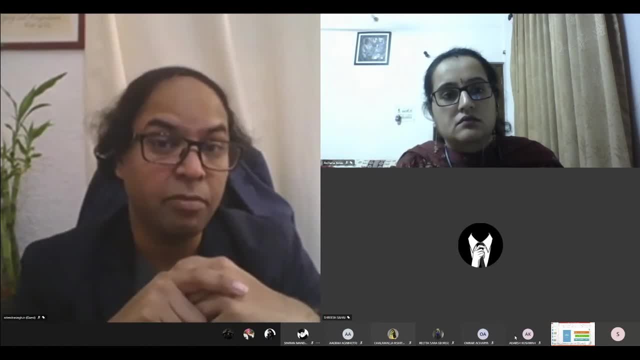 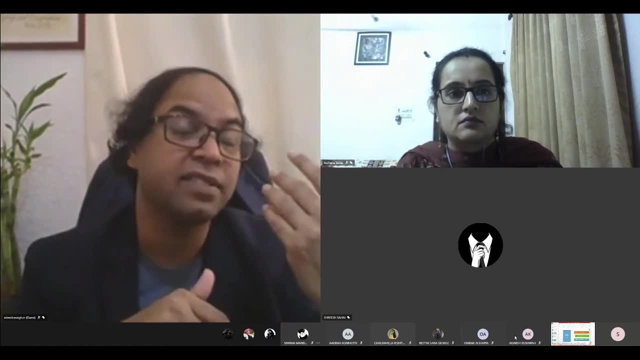 However, if I recently mentioned, however, EPR already had that in 2010, when they were proposing to construct a reactor. they already have a passive system into into their designs. They already have a passive system into into their designs. 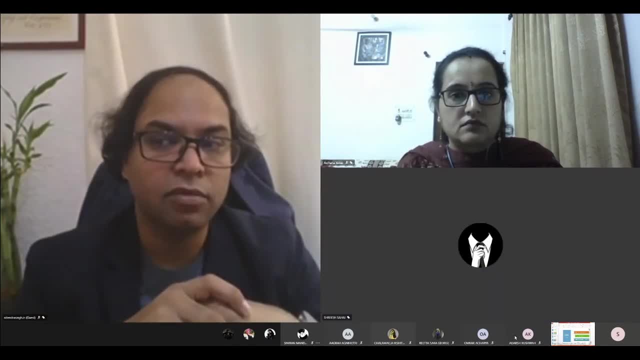 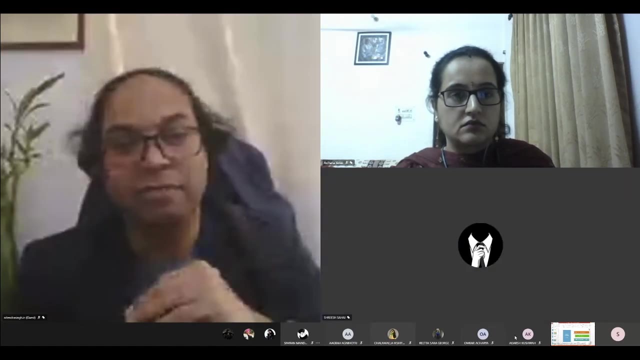 So it is not necessary that even these things would not have happened. We didn't have this level of safety aspect. Now, this is one and very clear, What these experiment did. they reduced this timeline, so to say, Because once TMI happened, they saw the core melt taking place, you know. and then they understood: okay, even when, and TMI was in US, okay. 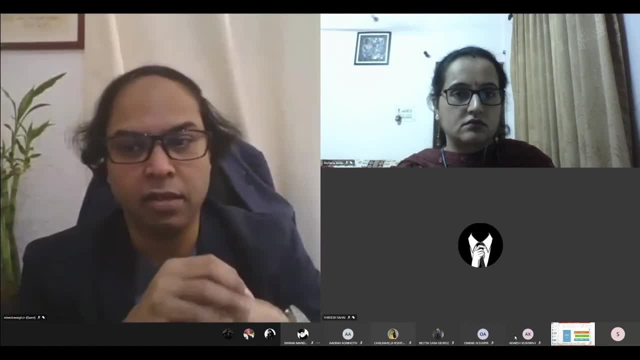 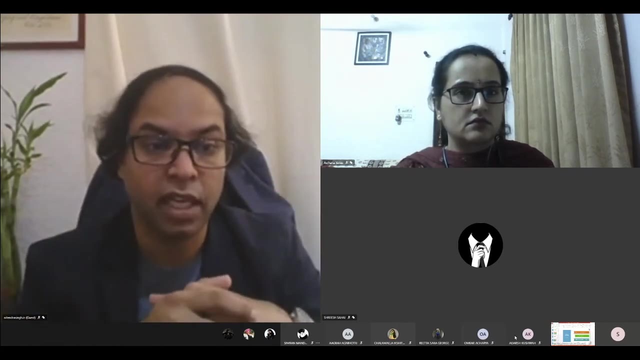 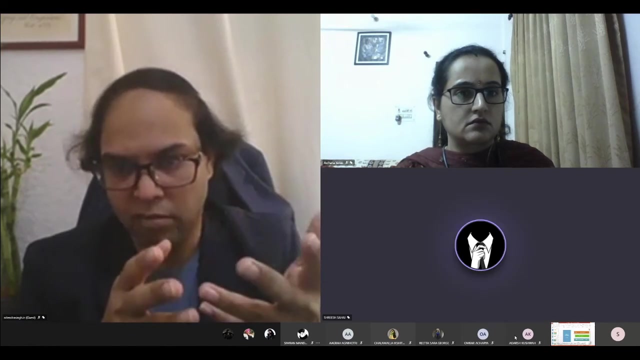 You cannot. US used to claim like we are the best in nuclear technology and they saw a meltdown taking place in their own reactor. So everyone and this report was also under US NRC, so they understood the criticality and the the real vision about real vision of this report. 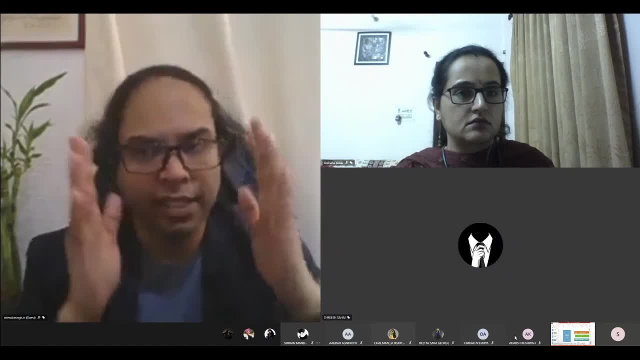 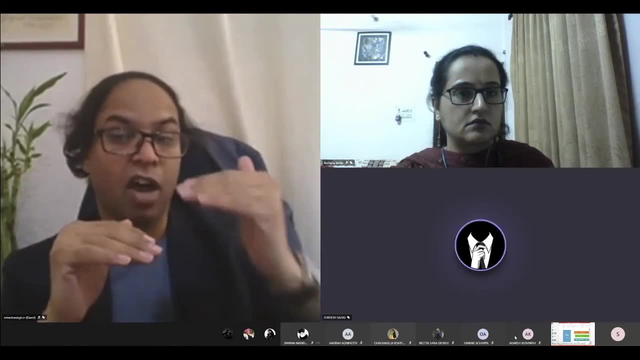 So, yes, these reactors in a way helped the nuclear industry. So, yes, these reactors in a way helped the nuclear industry. So, yes, these reactors in a way helped the nuclear industry. To consider all these scenarios which were hypothetical in the report, but now they are the reality in, in, in the life. 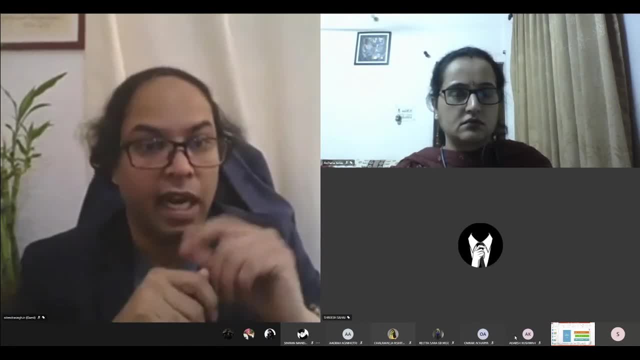 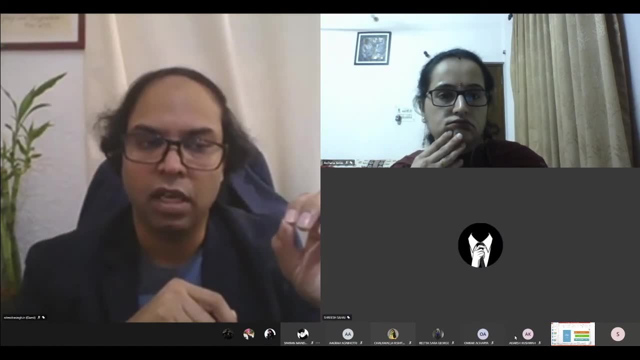 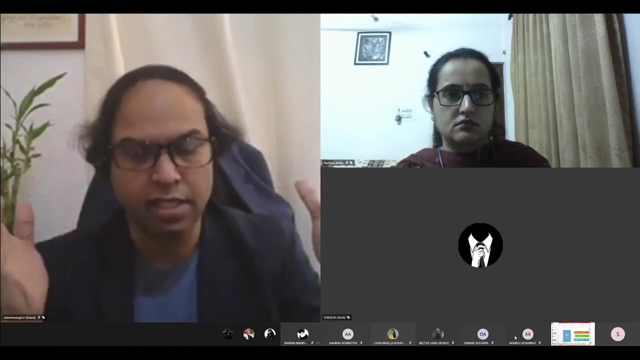 So somehow they accelerated further And after that, if I say after 1979, only everyone understood, like all these analysis, all the report, or all these hypothetical situation with all the designers, or all the- They are like people, experts around the globe. 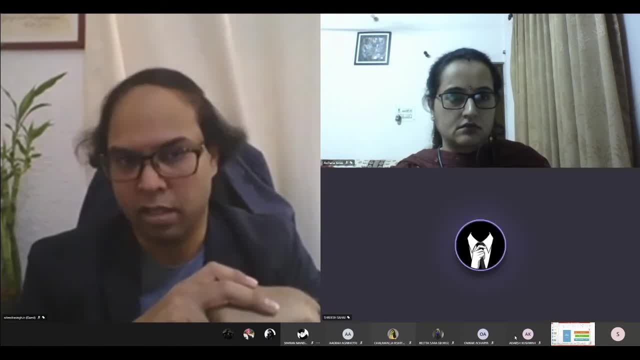 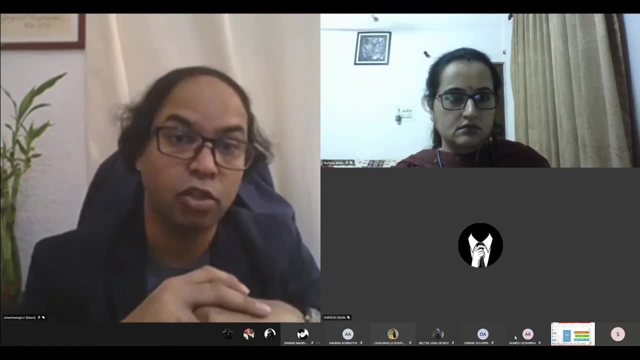 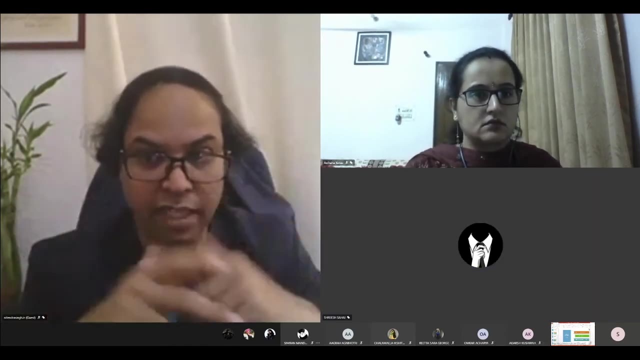 They are thinking. you should not ignore it in any manner. So this was the first lesson, then I would say, one of the key lessons everyone in the nuclear industry took at that time, and it is still continuing. So all that old research or this containment venting system I'm talking about. 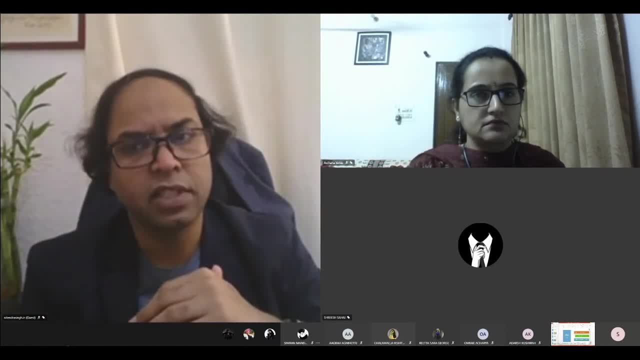 All the hydrogen management. This is under the research since then. only it did. It has not started after fukushima, so to say, or after chernobyl. i would say they started long back itself, after the res nation report. but of course the phenomena are quite complicated. so research. 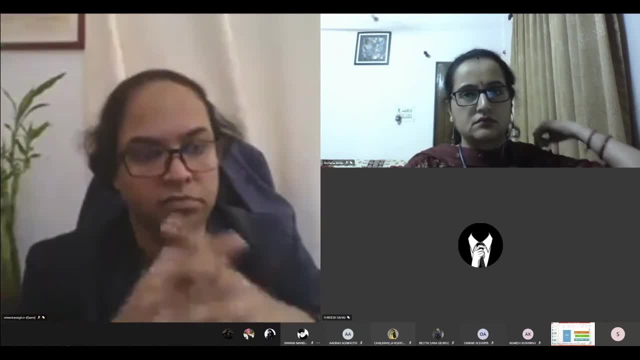 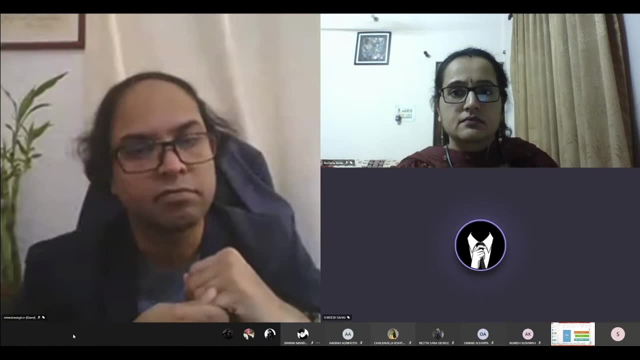 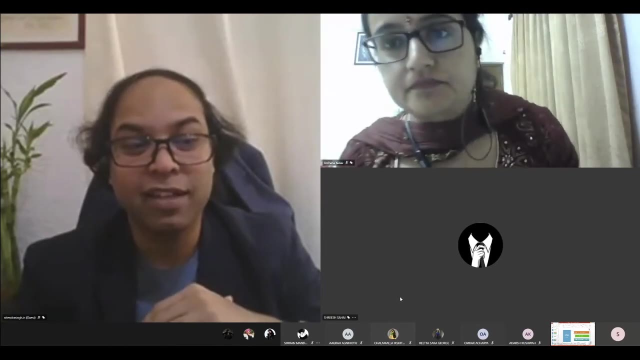 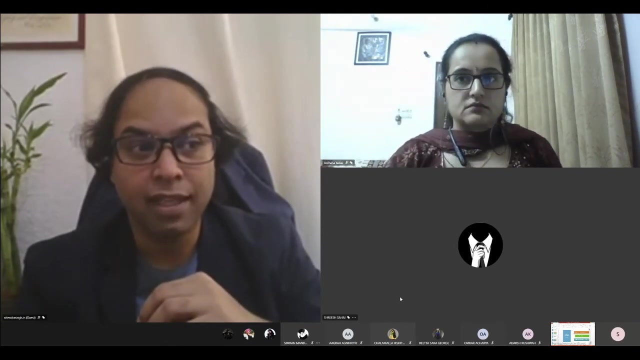 is still continuing and we are still improving on it. so this is the scenario. thank you, sir. oh yeah, i forgot to mention on your security part as well. so, yes, at that time security were- uh was not that much of concern, because the only concern when they were focusing on security was the war, because, uh, war used to be very prominent stuff at that time. 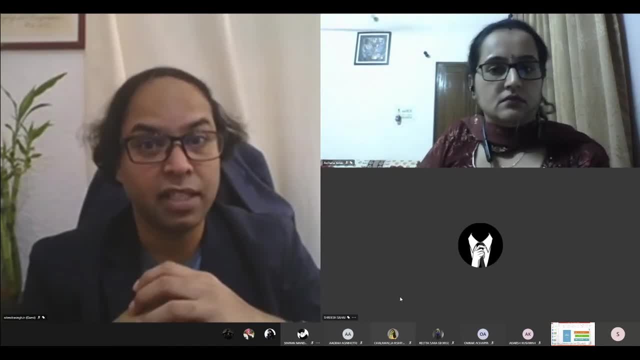 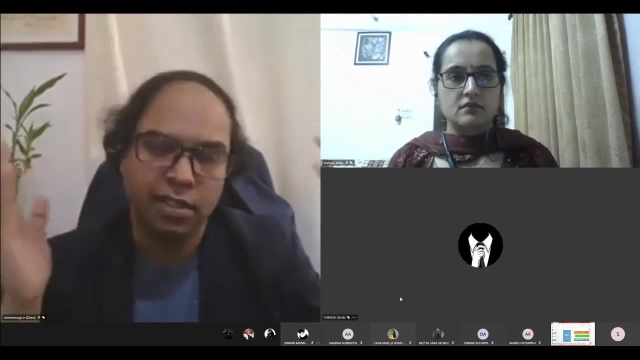 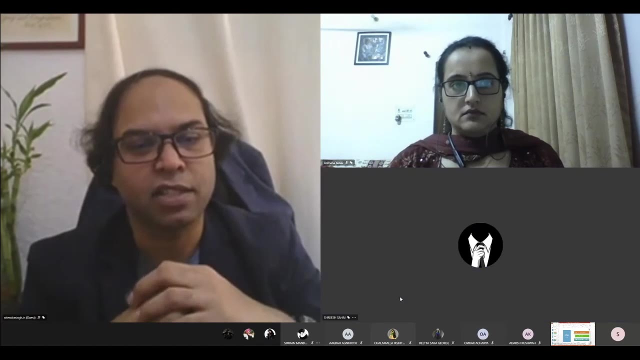 so people were afraid if some war-like situation will occur. so you need to make sure that your nuclear facilities are safe. and uh, like these, the superpowers at that time, they thought: if you have- uh, you know- the weapon of mass destruction, you are you, you are pretty safe, nobody will question you. 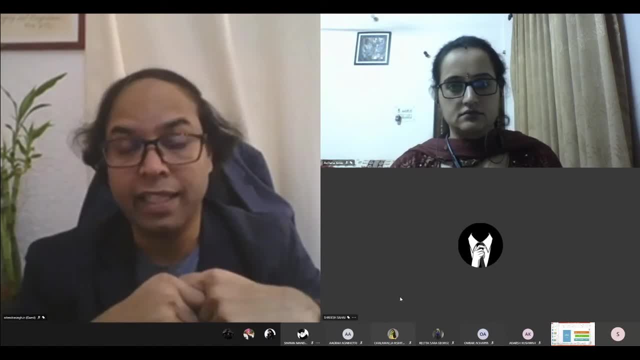 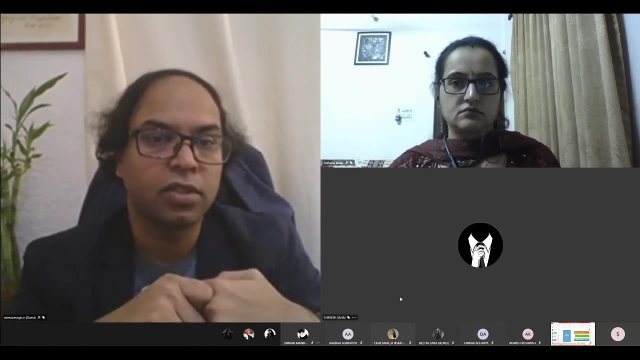 and things like that. the things went wrong in 90s when the terrorism started to rise, which increased the risk and which increased the, which in fact questioned the security aspect of nuclear facilities. so this was also the concern of the designers. so it was a very, very, um, very, very important thing that we were trying to address. 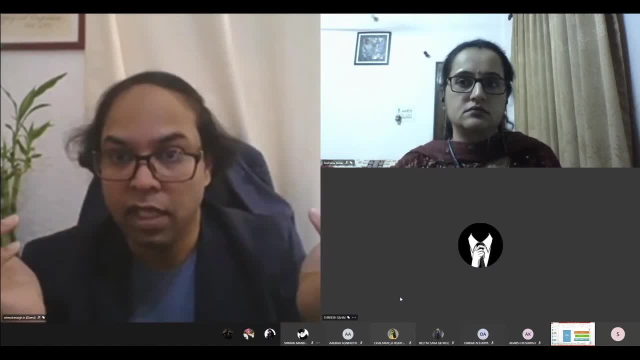 and i think this is very important and it was a very background of the work of the development of this university, and the development of the university was to make sure, like, for example, if you um, you know you, you drug the operator, for example, or if you kill the operator, so to say. 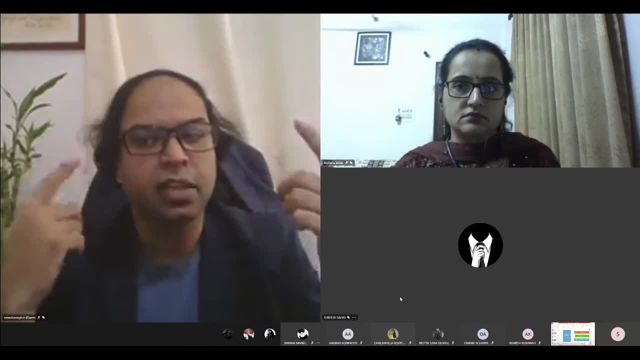 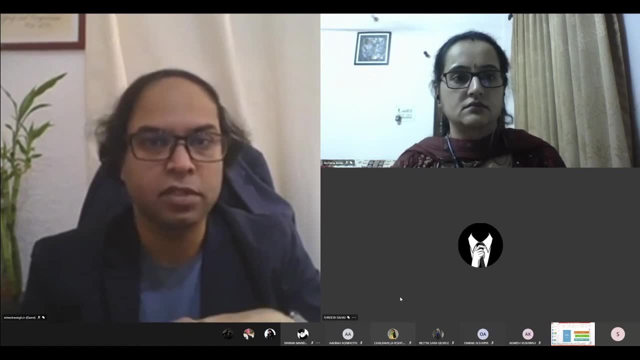 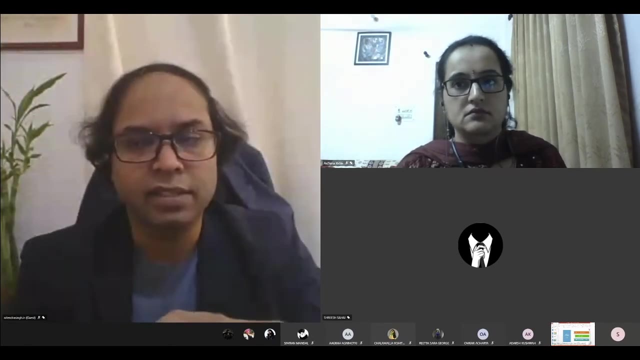 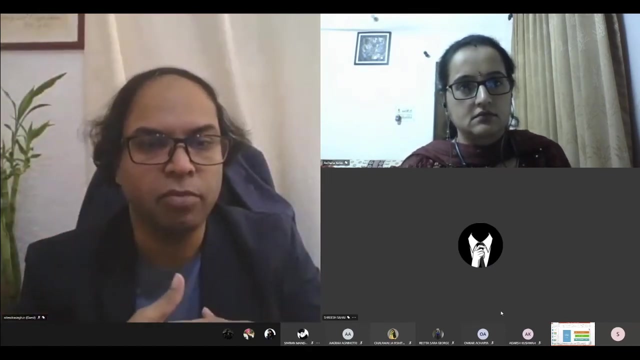 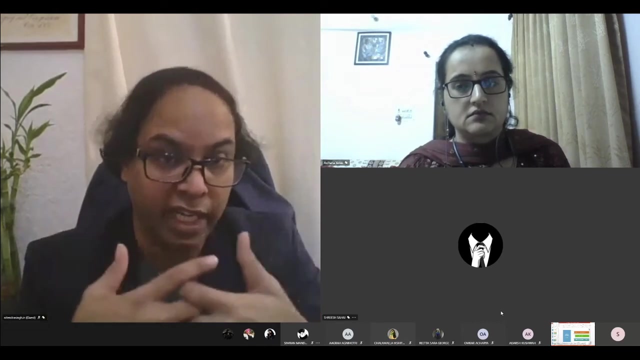 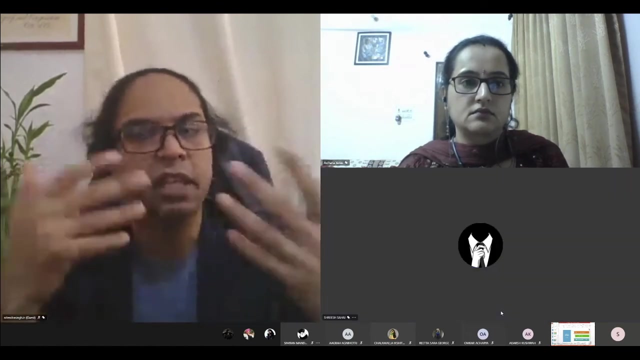 So somehow, to consider this scenario and to address this scenario, people started working on passive systems long back, So I would say the passive system research experimentally started long back in 1970s or 1980s itself. And, of course, with the improvement in technology, with improvement in data acquisition, with improvement in, you know, experimental possibilities, things got improved And nowadays you are using artificial intelligence as well in the field of nuclear safety. So, yes, everything kept on increasing. likewise, 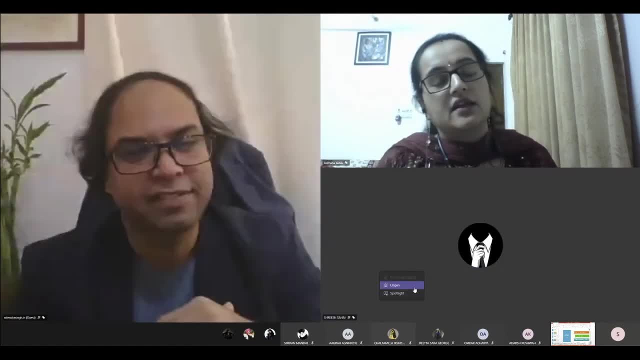 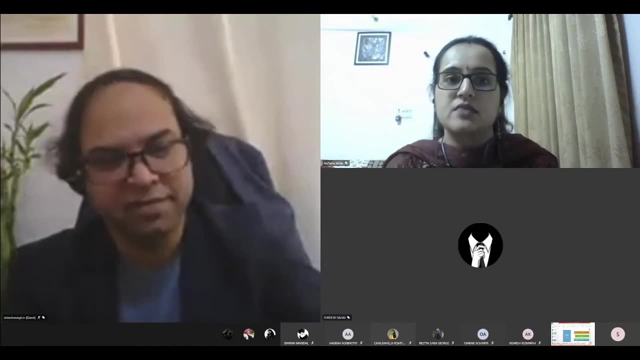 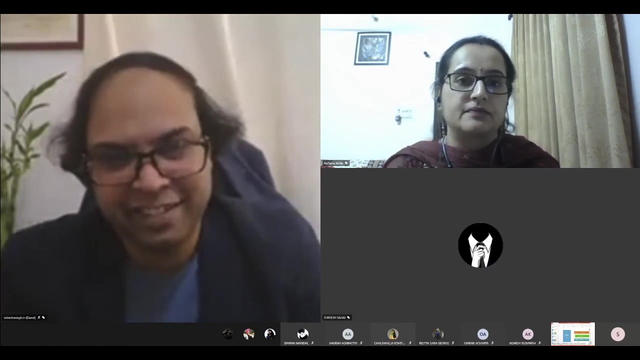 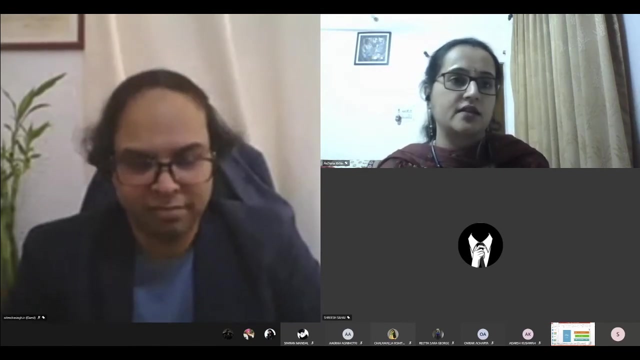 Thank you, sir. If I can add to it, even the Indian advance: The water reactors had this passive system, that is, safety system, And this was much before Fukushima. They had developed everything before Fukushima actually happened. And for Fukushima, of course, there were many changes that took place, even in Indian reactors And I think globally also, major changes took place. 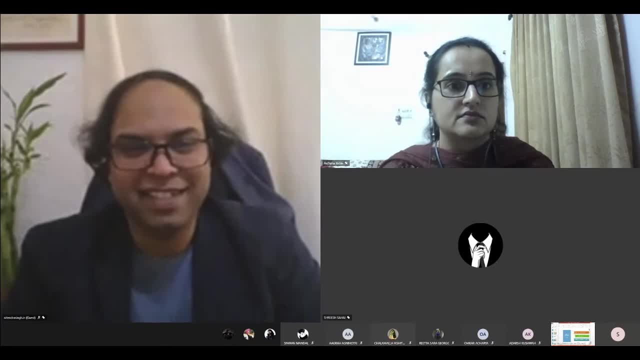 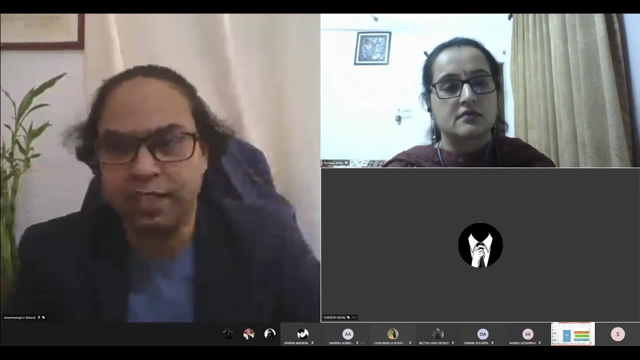 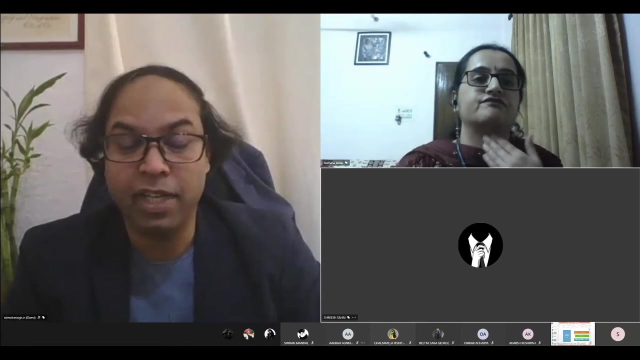 In fact, I would like to add to ASW, as you have mentioned, the advanced water reactor. Yes, indeed, This reactor, This reactor was designed in like 90s and they have all the safety: passive safety system. In fact, ASW has this feature that it can even operate passively. It don't need any operators intervention to even operate on its own. So, yes, and this was like way back. 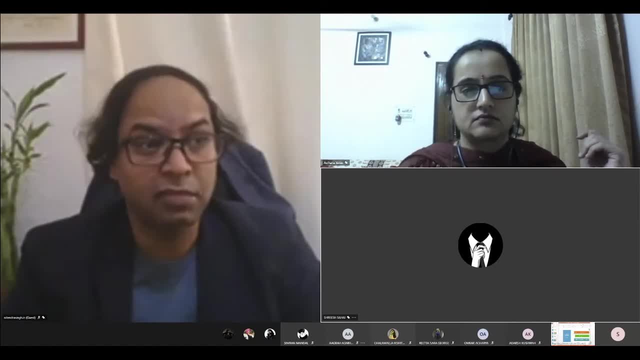 If you read the papers on it, the complete design papers, you will find in 2006,, 2002, 2003.. At that time- and Fukushima took place in it happened in 2011.. So, yes, you rightly mentioned So- people were working on this long, long, long time. They wanted to have it. 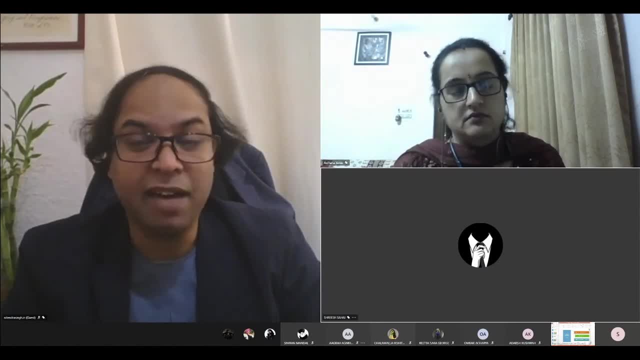 But, as I mentioned, Fukushima alarmed everyone. Now you cannot ignore. Earlier people were doing it by choice, but now it became the part of your- like, you know the design, or part of your thinking. so that's what will be the major change, i would say. i think both the regulators and the designers emphasize more on the safety features. 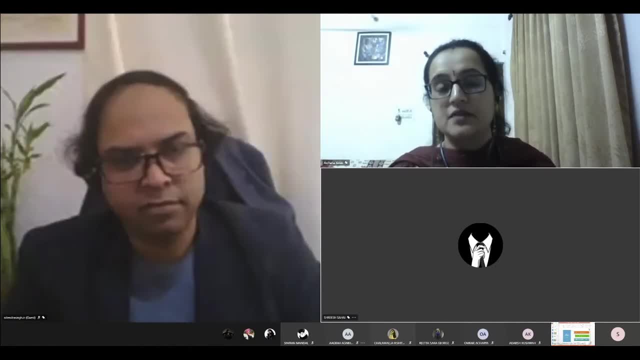 and actually are more sensitized towards these aspects. but it is like the others who are actually non-nuclear. it is their repulsion or hindrance, which is increased after such accidents, which actually retards this entire motion. the nuclear industry is actually not taken or set aback by. 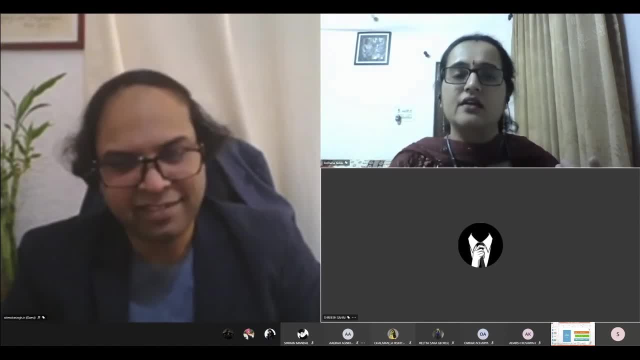 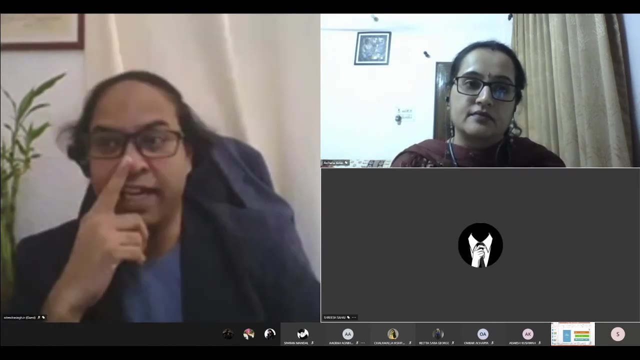 any of these accidents, so they always gain. it is, i think, true for any industry that you gain from your accident, but of course, for chemical sector we haven't seen such developments happening for nuclear. they have learned a lot. yes, i want to add to it: you have rightly. 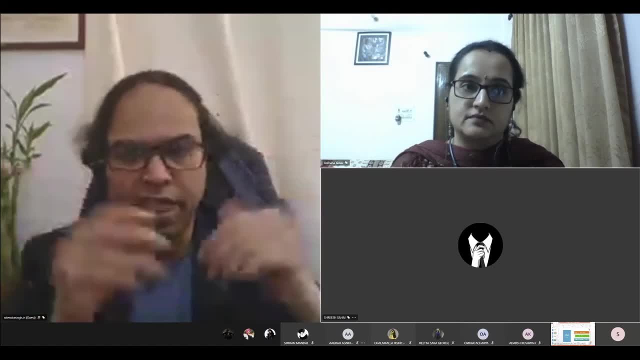 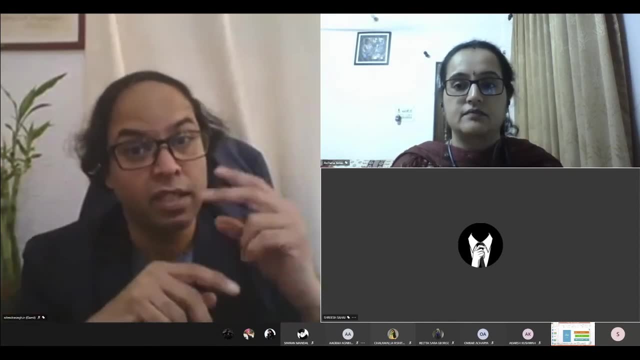 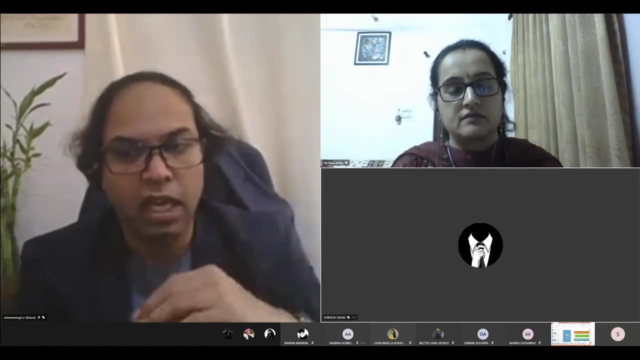 mentioned, like not other industry, even even if you take mining industry or you take a chemical industry, they have not improved a lot in this sense. indeed, the two industry which i always respect- and they go hand in hand because they are directly related to the people- are the aviation. 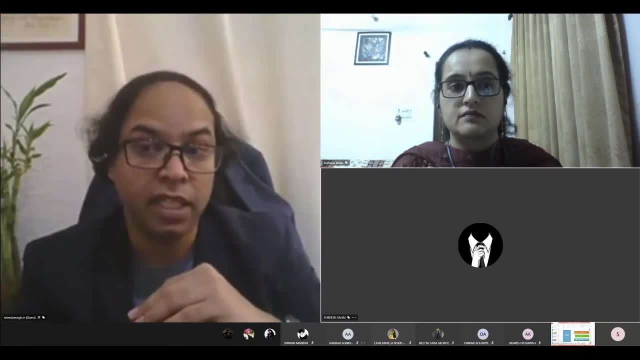 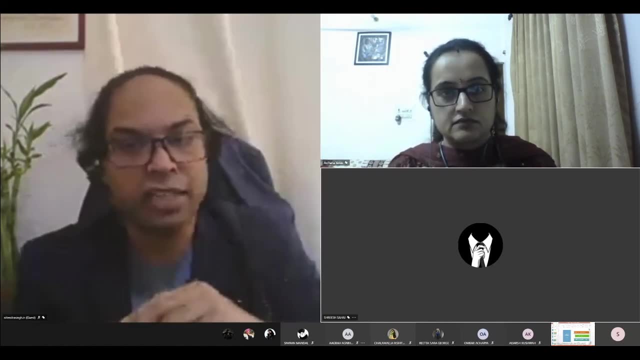 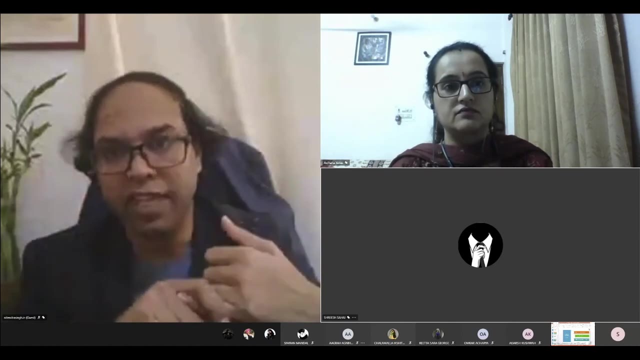 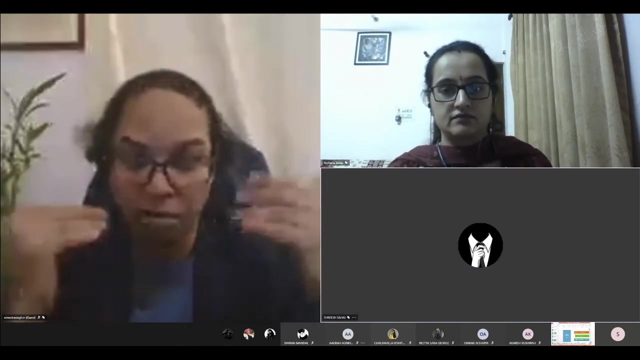 and nuclear industry and both of them. you see the improvement. if you remember, there were a large increase in the aircraft accident in the late 90s because the people were more. people were became more capable of taking those flights and flying. they had the economy started increasing. everyone wanted to fly. so number of flights, number of 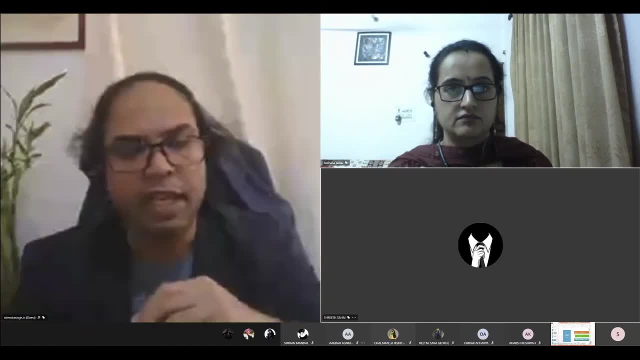 aircrafts increases increased at that time and resulted in a lot, lot many accidents taking place. but then they came up with new design. if you see the a380 or the dreamliner, they, they came, you know, they were not, you know, just like that one day affair. okay, we want to make a haircut tomorrow. 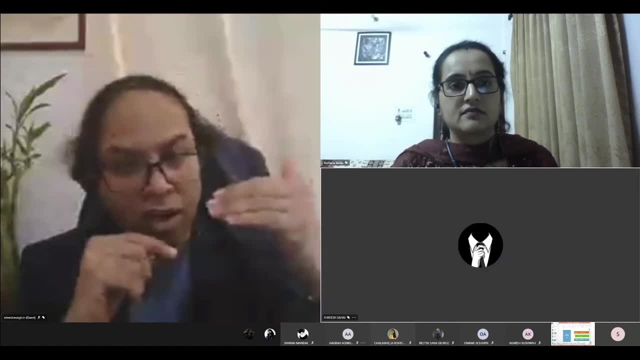 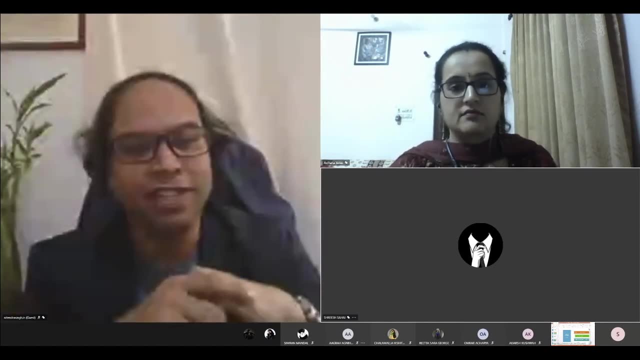 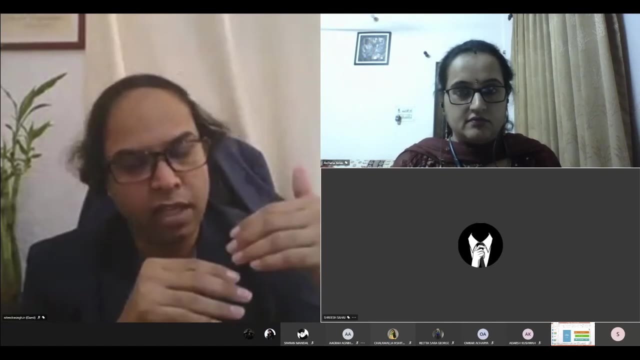 just do it. they had a long research for it. you know, making such a big aircraft, you are still keeping the dimensions of the wing and everything. they change the entire aerodynamics, they change the fuselage, everything. so this, this way, you continually, continually improve your research and to make. 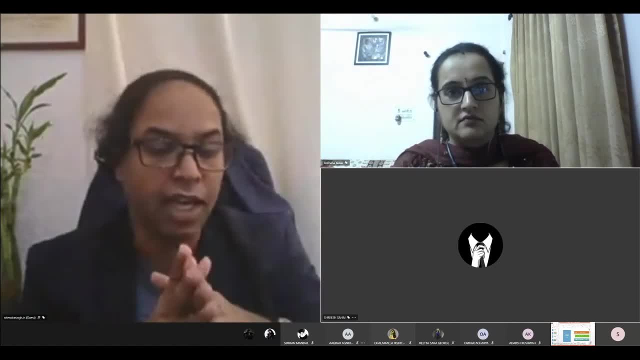 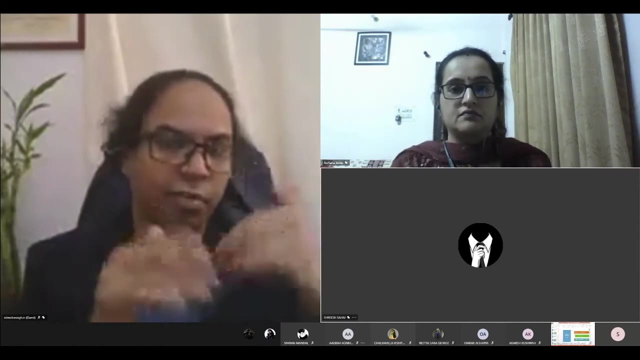 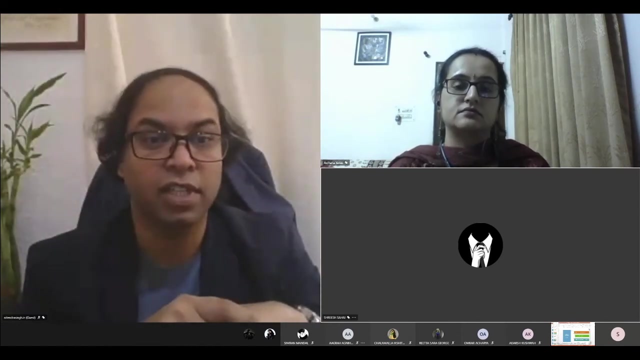 things improve this. this is one of the good aspect, mainly taken care by two industries: nuclear industry and the aviation. so, yes, things were. people are walking, as rightly mentioned, asana, like the designers or operator, or all the people, or i would say all nuclear professionals. they were not at setback or they were not just sitting. okay, something will happen then we will. 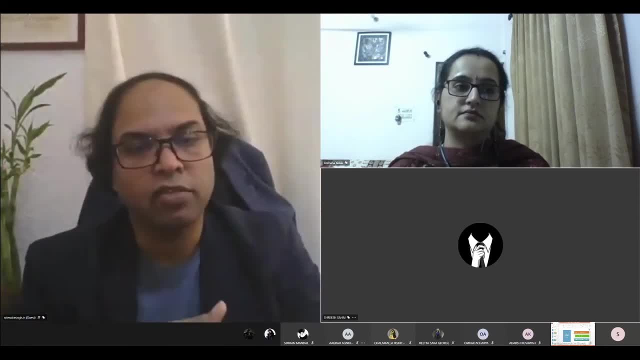 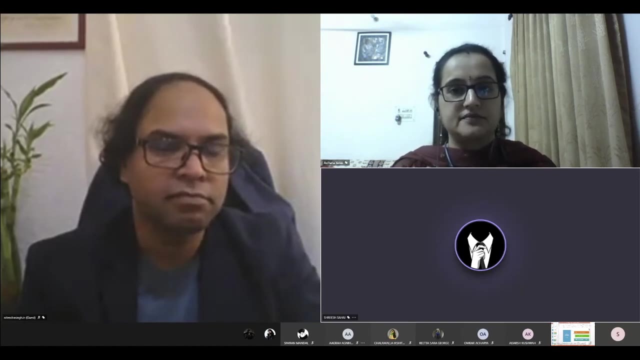 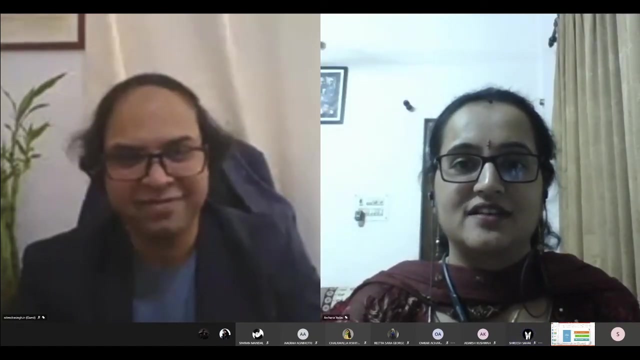 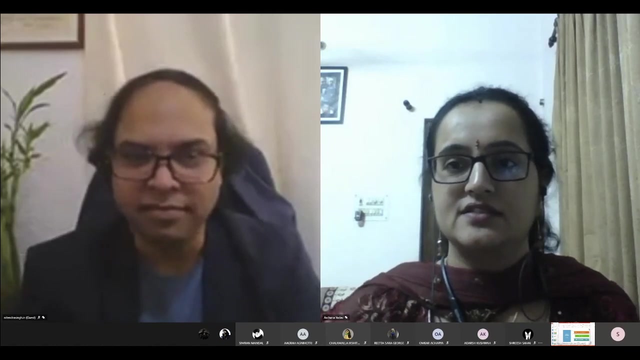 start thinking they were continually walking to improve the safety and all the aspects. but these things just highlighted the, the, the concerns of the public, peace. any more questions? thank you, mom. thank you, sir. any more questions? if you wanted to ask something, or is it clear to you? 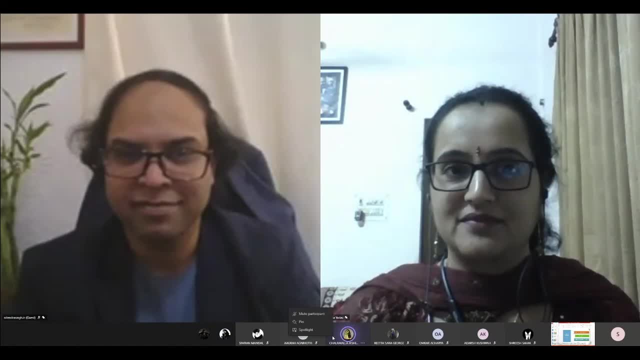 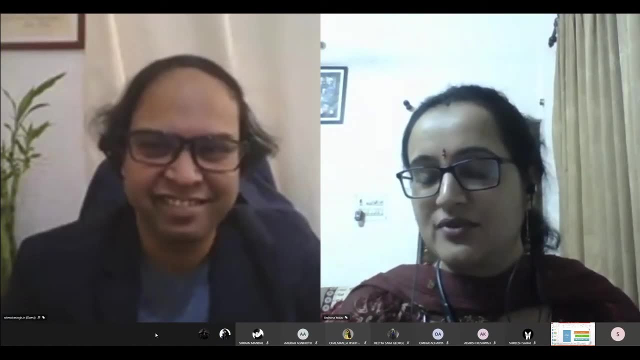 um, i wanted to ask, but then rita asked the same question and now i'm clear with it. thank you so much. okay, right, so i think there were. there was one question which tushar wanted to ask. tushar is actually from the second year. he doesn't have much information about the reactors and he wanted to ask about. 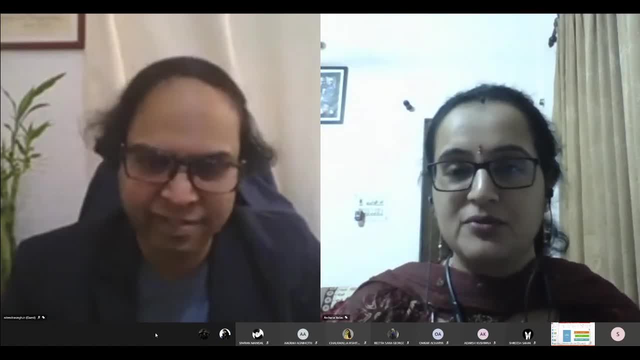 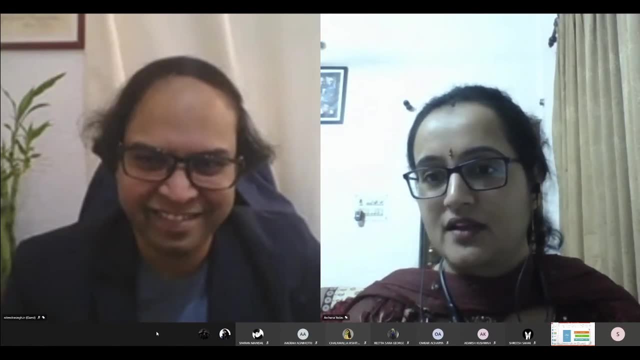 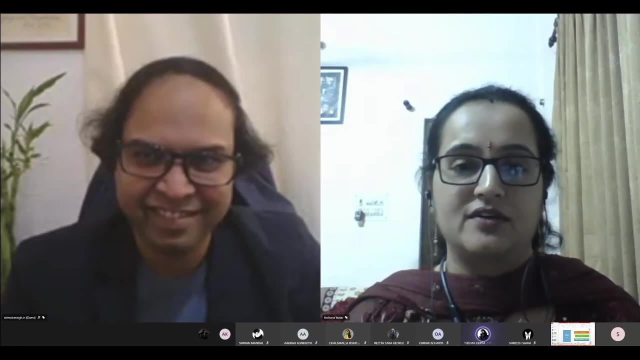 what actually happened in chernobyl, and samyak and puge together did a wonderful job in clarifying himself. so, tushar, if everything is fine, we can move on with the questions. would like to ask something? no, ma'am, it's fine. thank you right, but one thing i would like to. 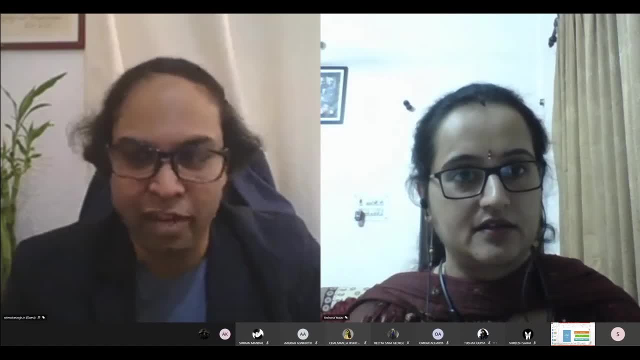 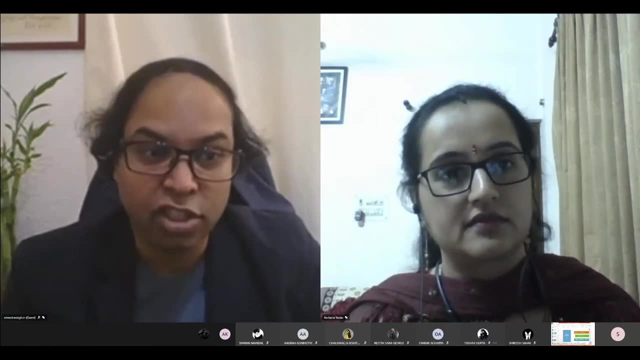 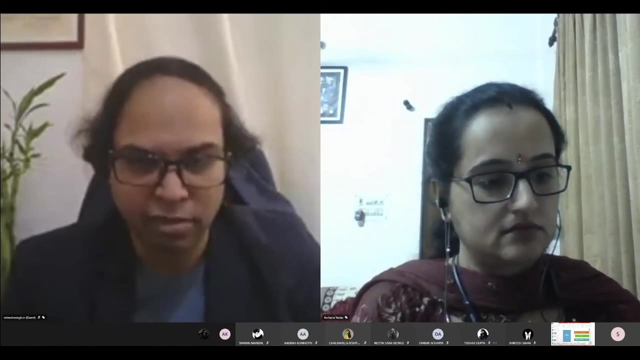 highlight here which most of the people are not very much aware. they think like chernobyl and fukushima are the same, but i still want to highlight chernobyl and fukushima are two very different accidents. chernobyl was a kind of nuclear accident, i would say. however, fukushima 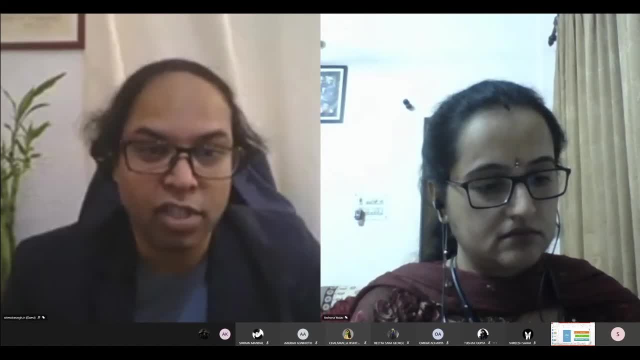 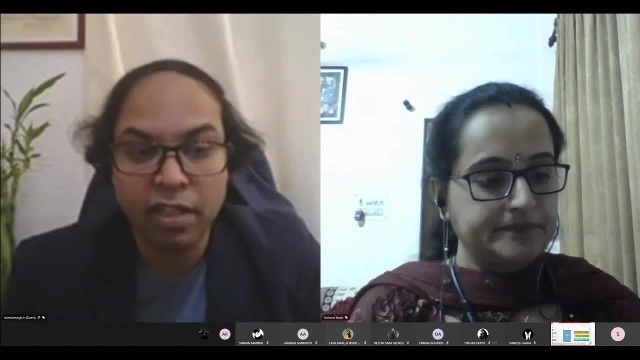 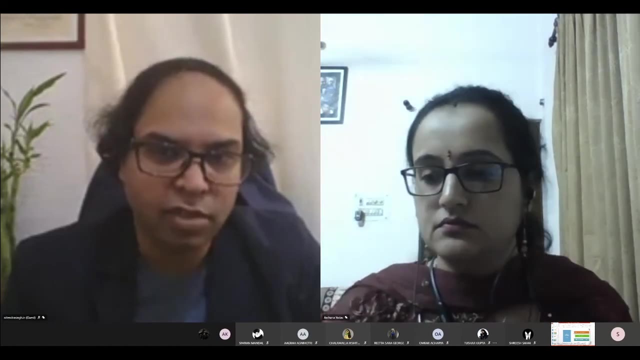 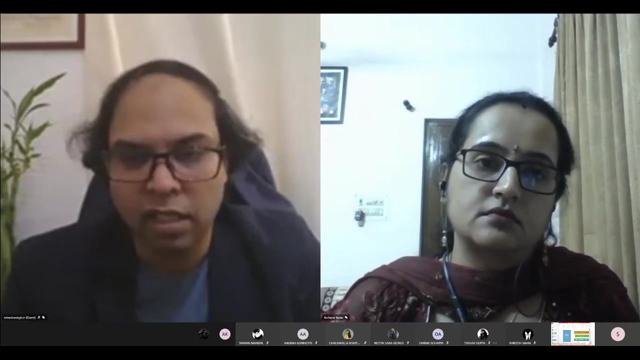 was not the the nuclear accident. it was initiated by the natural calamities, but the accident which progressed it was mainly due to the chemical reasons. the explosion was not the nuclear explosion, it was just the hydrogen explosion, which which is a kind of industrial explosion, i would say, because hydrogen explosion can occur in several industries where you have a high 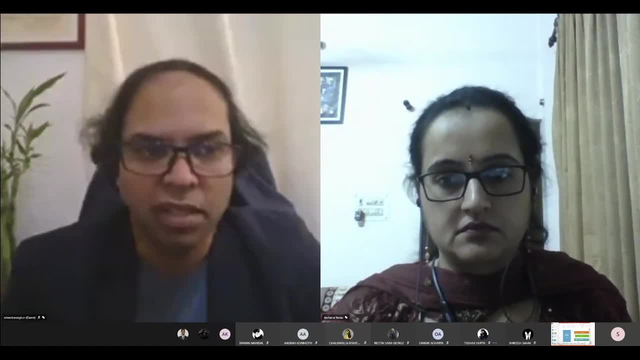 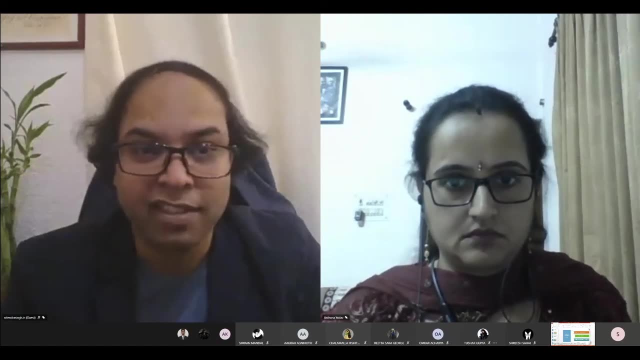 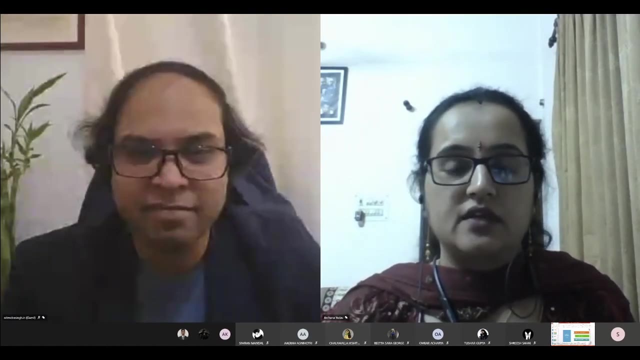 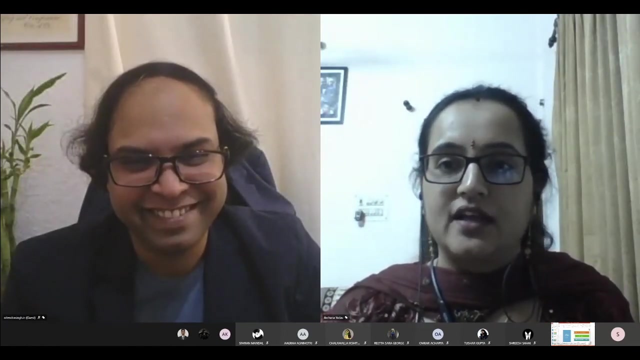 temperature interaction and water interaction, maybe in a metallic industry and others. so yes, this people should understand they are not the same accidents. i think with no more questions we can wind up this session. i thank you for your time, my pleasure and this wonderful lecture, and i thank all the participants because it was. 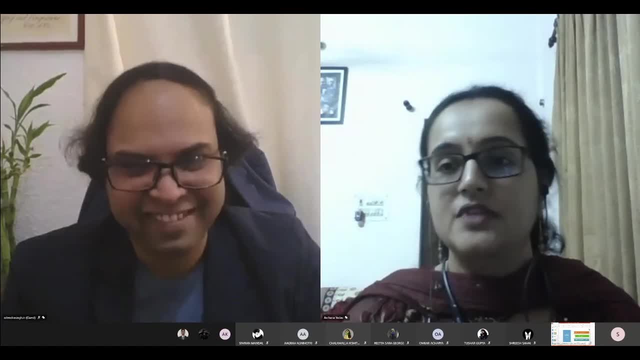 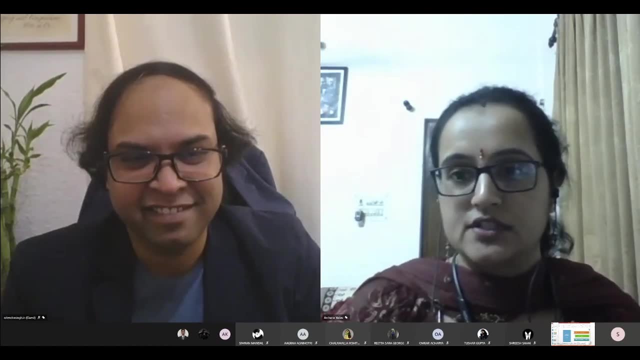 became interactive because you all were present. so i hope this session went well and i hope you all enjoyed it, and i hope you all enjoyed it and i hope you all benefited you and you had some good takeaways. so i request you to just go to the menti meter and 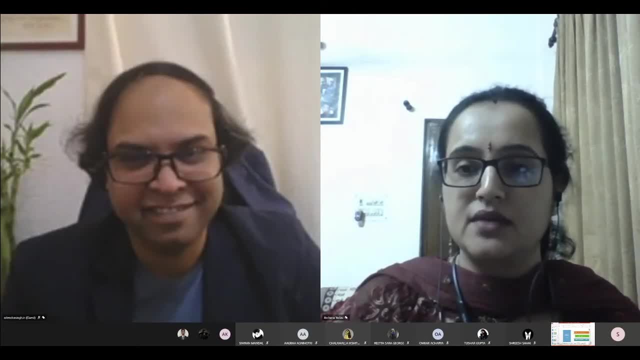 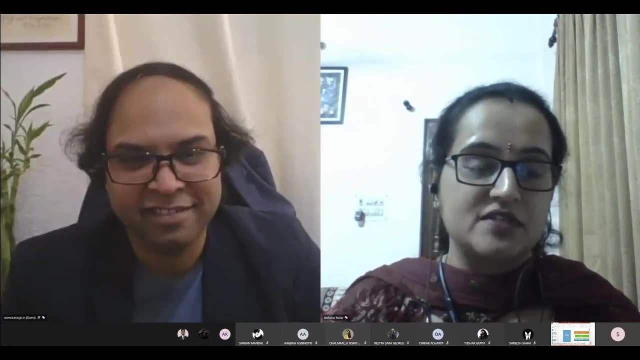 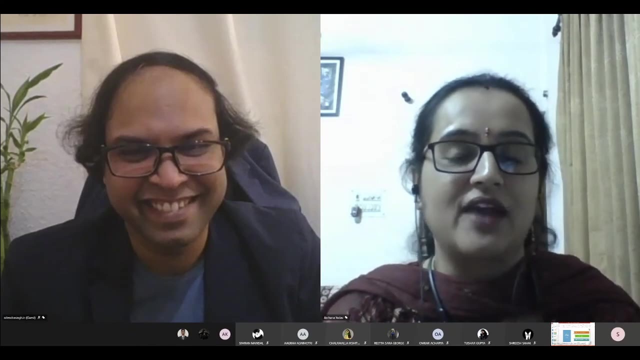 fill up the feedback of this lecture. in case you require something more, please let me know so that we can arrange for a further interaction. it has been almost like one and a half hours since we started, so that's a long time. thank you so much for to the speaker, who has given us some 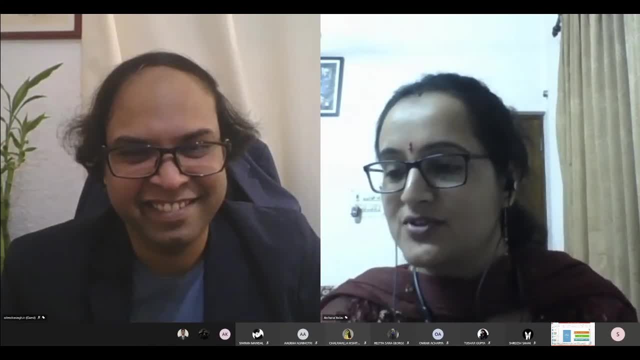 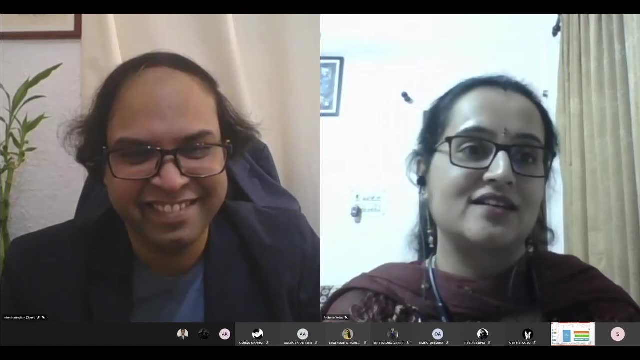 valuable information, and to me also because i just came to know you all and i hope you all did have some valuable information, and i hope you all did have some valuable information, and to me also that there are 438 types of nuclear reactors that are operating around the globe, and so that's quite. 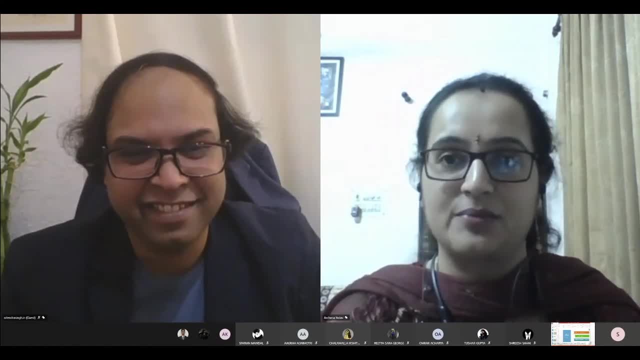 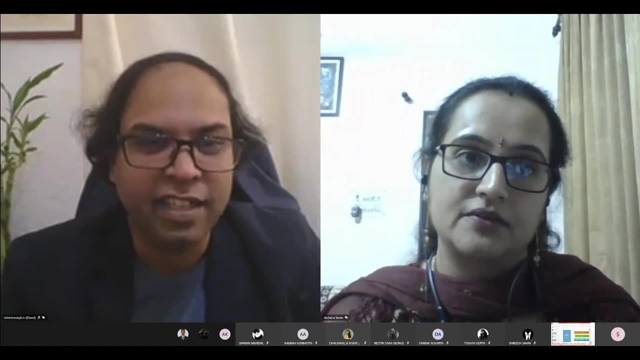 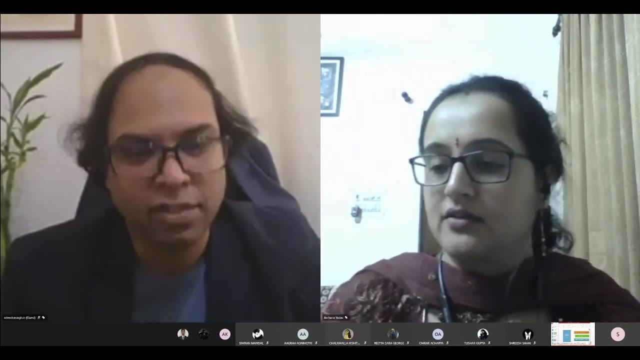 a different. i mean that's quite a wide variety which is operating, not variety. 438 are operating of different kinds, like out of which there are pwrs, there are vbrs and different kinds, but 438 are operating. for the moment, reactors are operating. okay, thank you so much. i hope, uh, all our 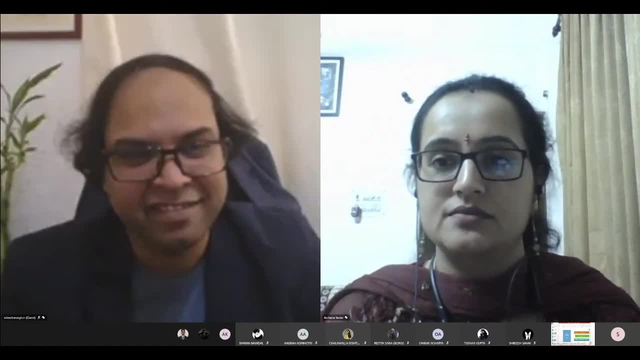 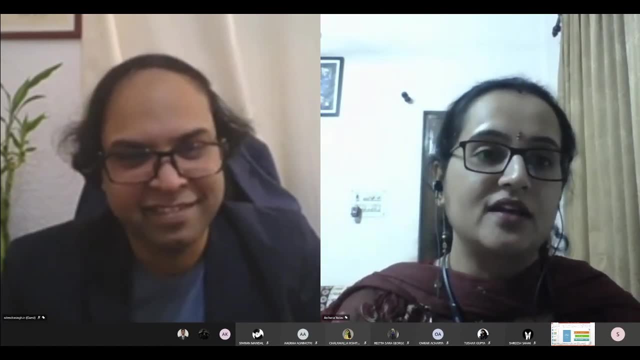 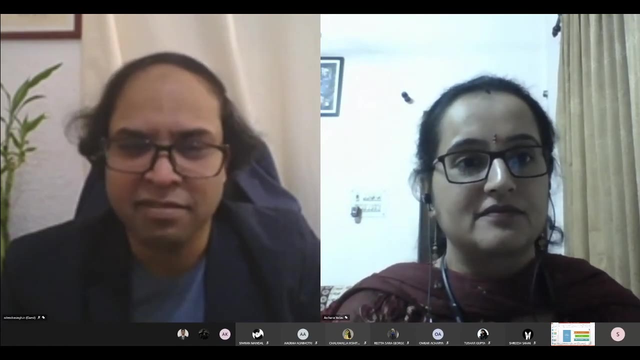 participants would clarify their doubts. in case you have some more, you can let me know. i can pass on your questions to the speaker. and let me tell you one more thing. uh wanted, if you can, to know that if you can share your presentation, so would that be possible? yeah, yeah, if you want, there is. 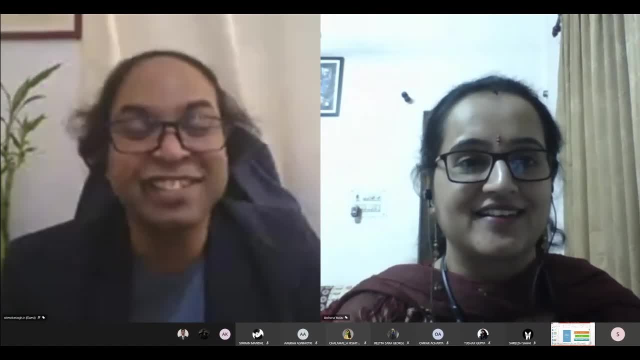 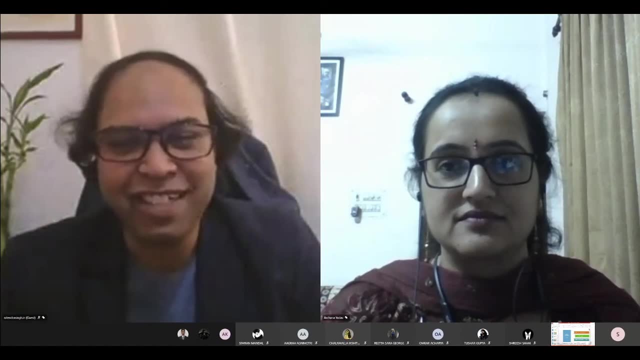 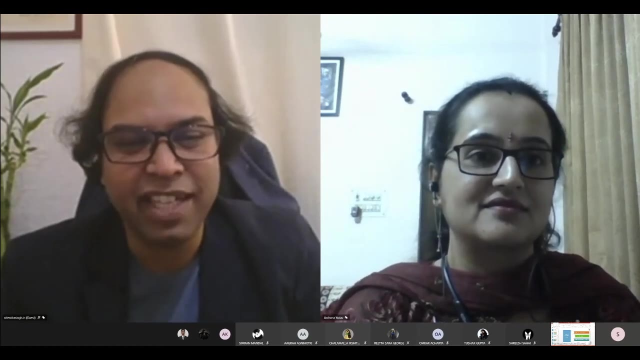 nothing in that presentation. i i never uh this. this is one thing. okay, just out of this context, i was discussing with one of my colleagues: well, i don't make this self self-explanatory presentations. you can have it. but if you have any doubt with this presentation, you just write to me.